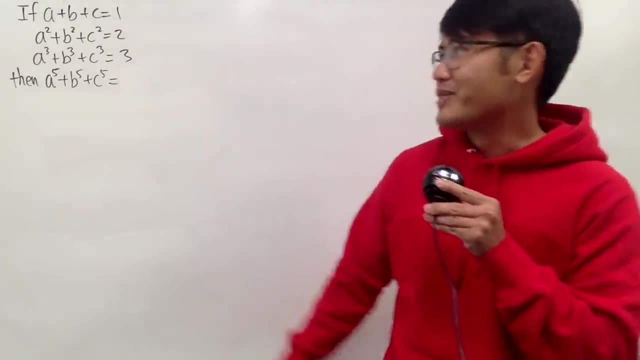 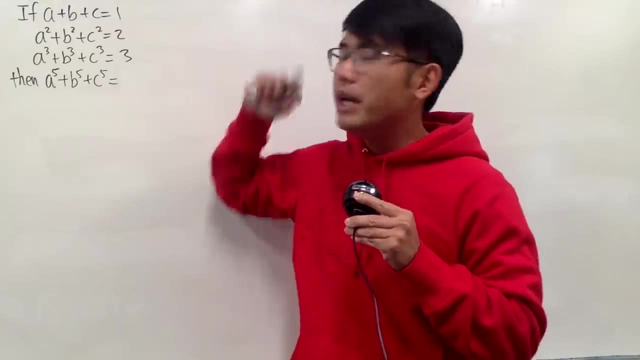 Okay, let's do an extreme algebra question for fun. Here's the question: If a plus b plus c is equal to 1, and a squared plus b squared plus c squared is equal to 2, and a cubed plus b cubed plus c cubed is equal to 3, then let me ask you guys what's the value for a? 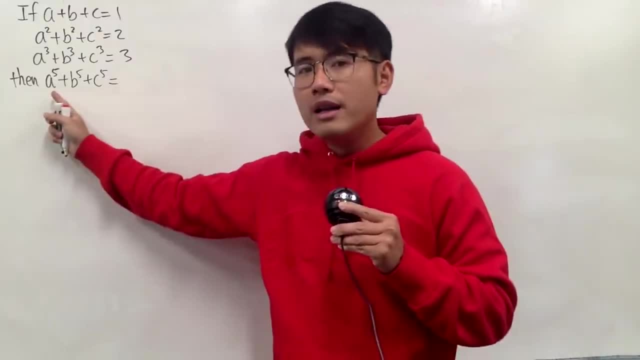 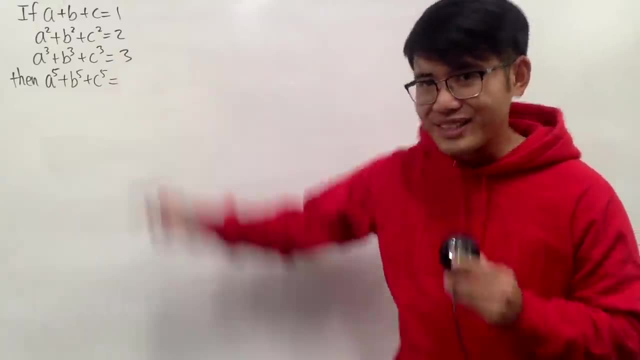 And we know the fourth power is going to be too easy, so let's deal with the fifth power. Let me ask you: a to the fifth power plus b to the fifth power, plus c to the fifth power is equal to what? And, as always, please pause the video and try this first. 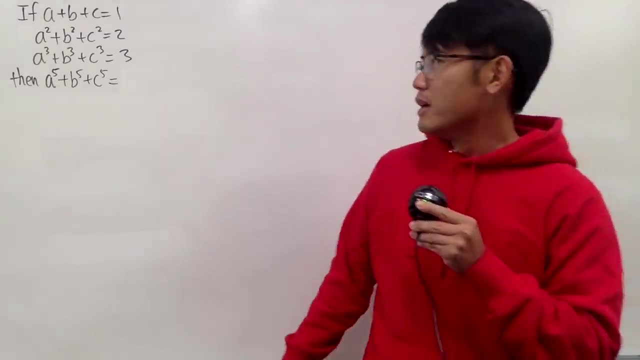 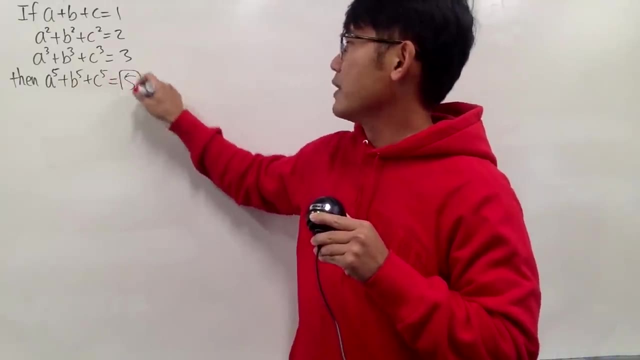 Okay, so of course, you see, the first power is equal to 1, and then the second power is equal to 2,, the third power is equal to 3,, the fifth power is equal to 5,. right, Happy April Fool's Day. Yay, And, as always, that's it. 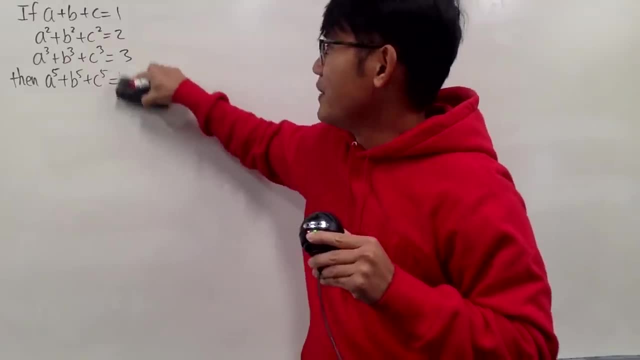 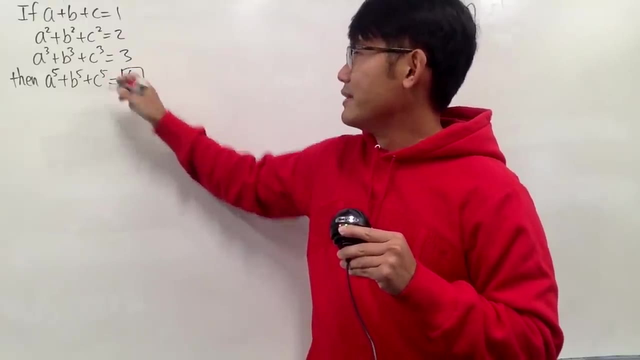 Okay, just kidding, just kidding. If you end the video, then no, no, no, no, no. The answer to this is not 5.. In your serious business Now. the answer to this right here is equal to 6.. 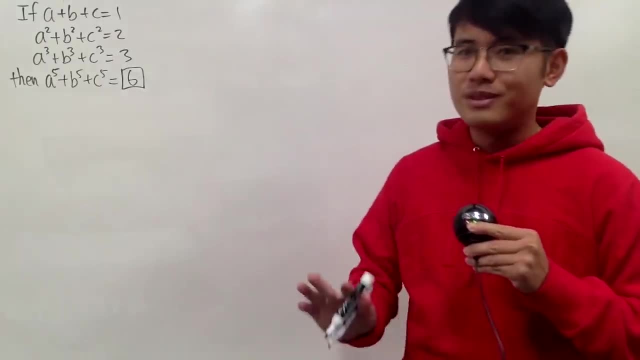 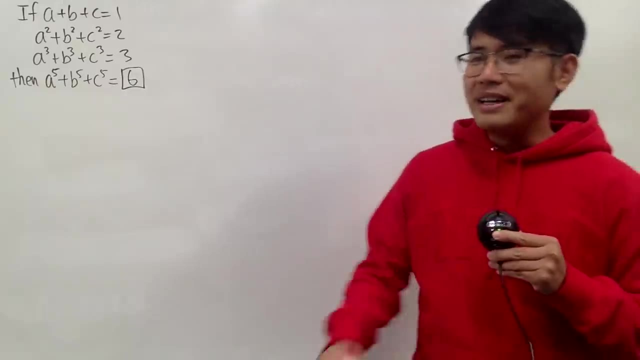 Why? Because 2 times 3 is equal to 6.. No, that's a joke again. Why Because 1 plus 2 plus 3 is equal to 6.. Sorry, no, Okay, in your serious business, this right here is really interesting. 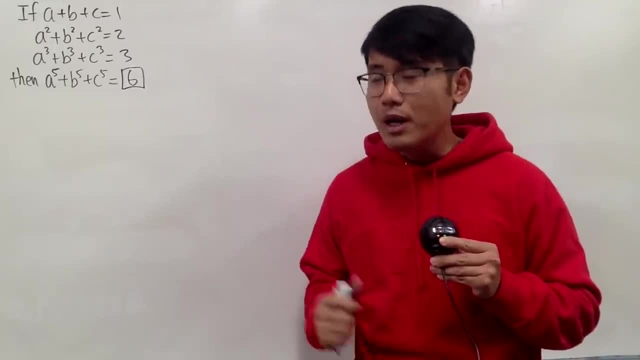 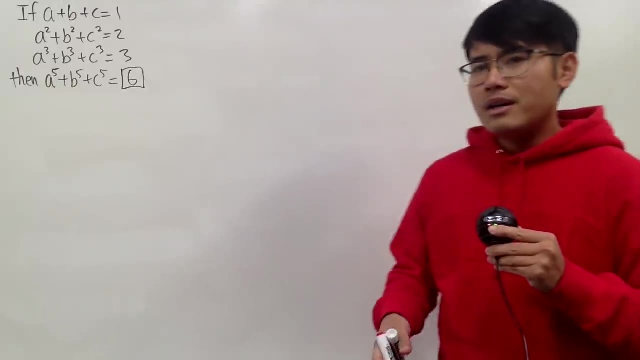 and I can tell you guys a lot of new identities. Maybe you haven't seen it before, but it's pretty cool, all right. Especially, you'll see this in discrete math, in terms of, For example- you guys know about Pascal's triangle. 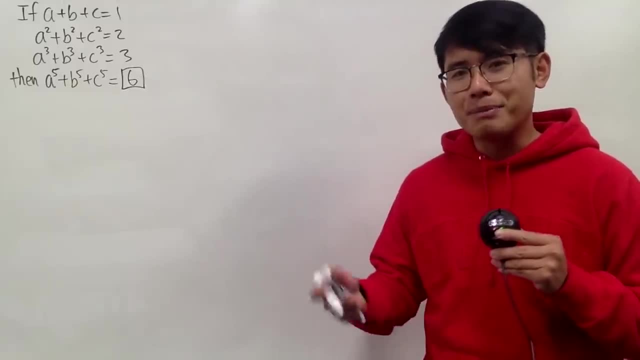 but have you ever seen, Have you ever thought about? do you guys know, what a Pascal's pyramid is Like the 3D version? So I'll go over that right here as well, and we'll just do a lot of algebra right here. 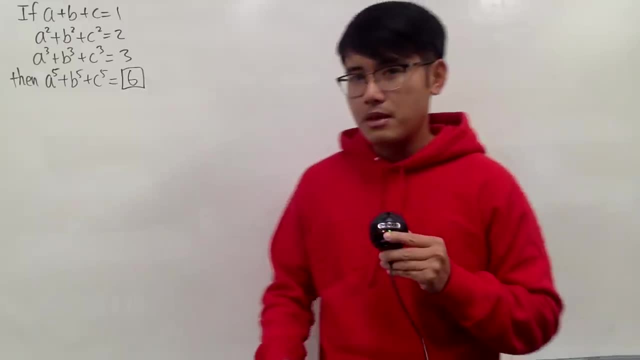 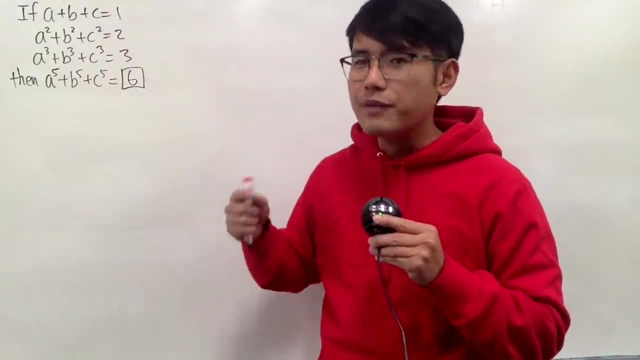 So that's why I call this the extreme algebra question. So here we go. So in your serious business now. okay, to get the fifth power by using this equation. of course, you can look at the first equation and just maybe raise both sides to a fifth power. 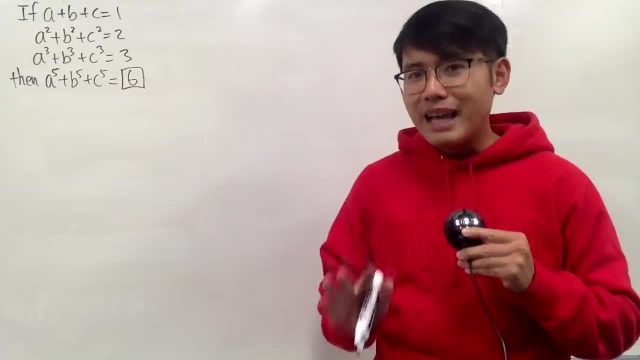 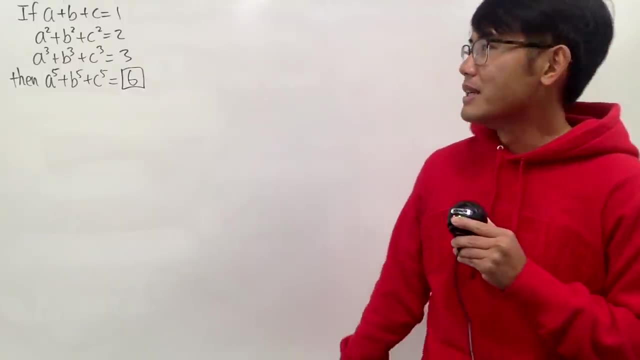 and maybe work something out right, But don't do that. Life doesn't have to be like that. Okay, so if you do it like that, leave a comment down below and let us know how that goes. Another way to produce fifth power is, of course, we can multiply this and that. 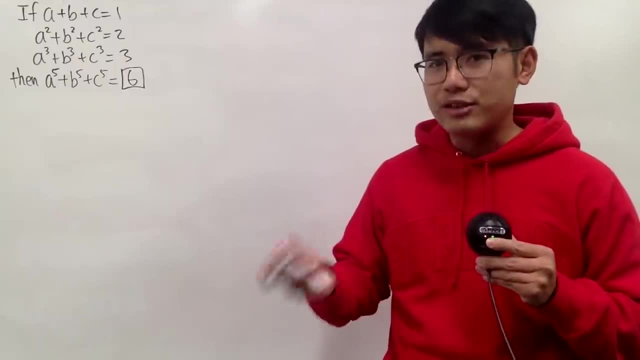 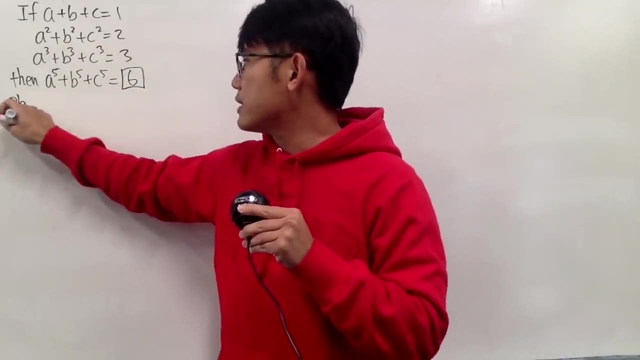 and of course we'll end up with some other extra terms, but hopefully they are not so bad right. So what I will do is I will just actually multiply this and that together and see what will happen. So let's make an observation first. 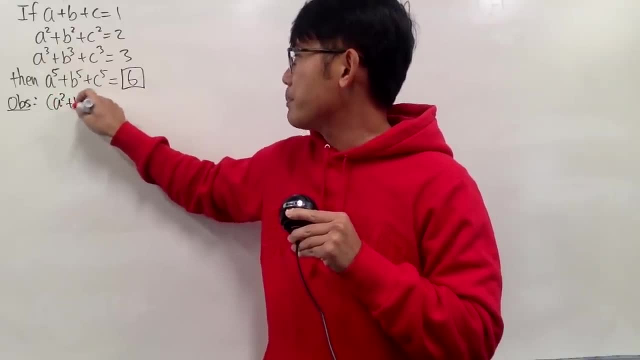 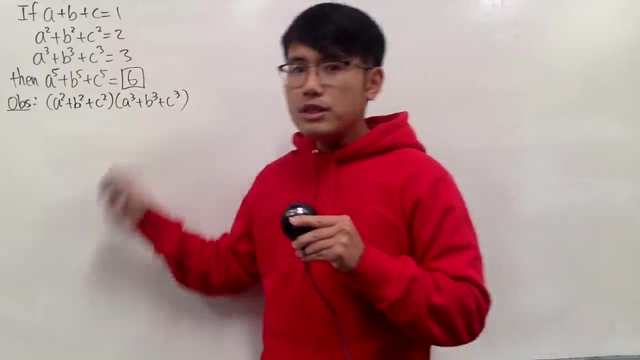 So I will just write down a squared plus b squared plus c squared, and then we multiply it by a cubed plus b cubed plus c cubed. So I will just multiply this out and I will just write down everything. 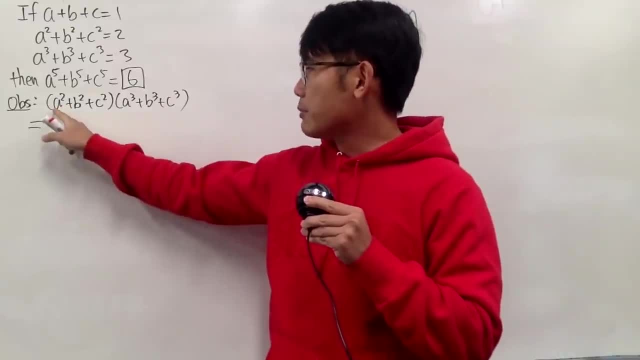 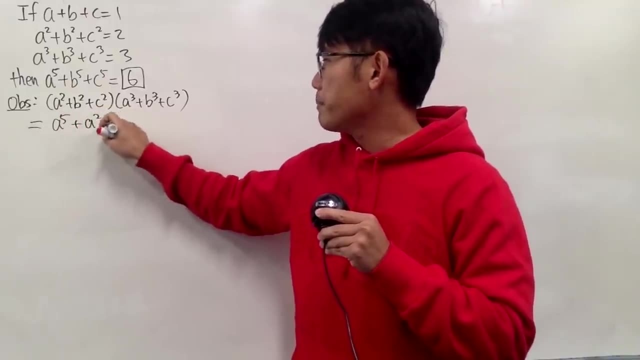 I'm not going to use any of the formulas or whatever. so here we go. I will just multiply this and that. of course we get a to the fifth power, and then we continue. This times, that is, plus a squared b cubed and then a squared c cubed, and then, of course, you do the rest right. 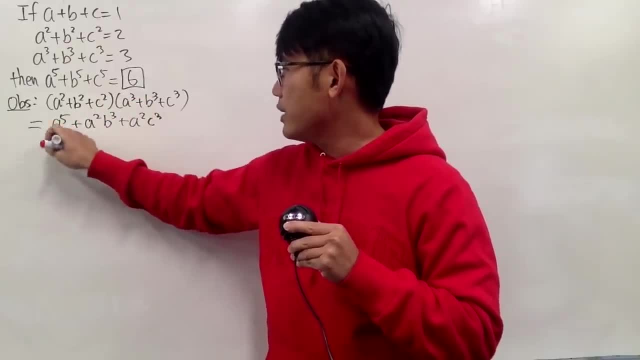 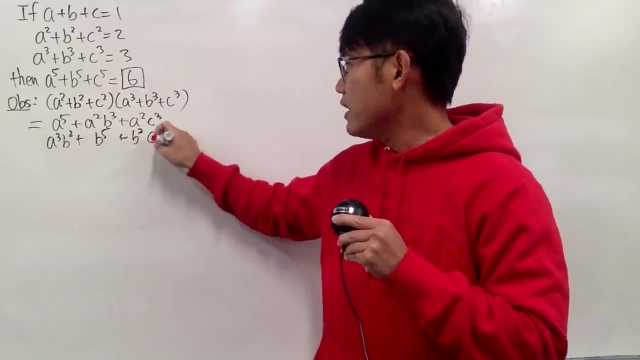 For the next one, it's going to be b squared times that which is a cubed, b squared plus this times that which is b to the fifth plus b squared. You actually see a really nice pattern for this equation, okay. 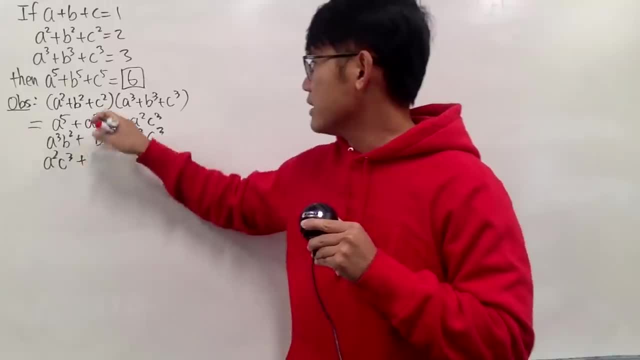 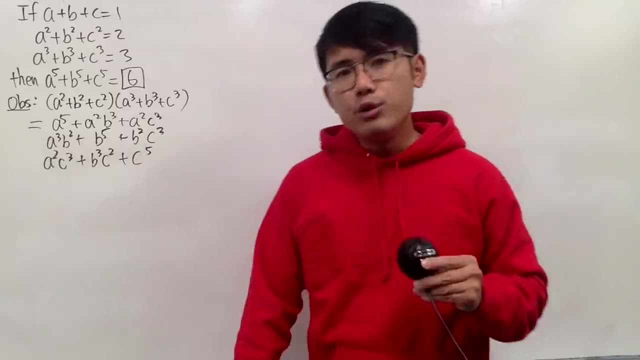 So it's actually no joke, pretty fun. Plus, the next one is going to be b- third power, c squared, plus c to the fifth power. all that It requires extreme concentration for all this as well. okay, But anyway, here is the deal. 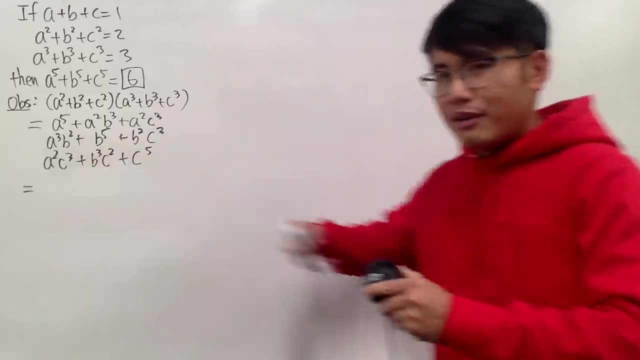 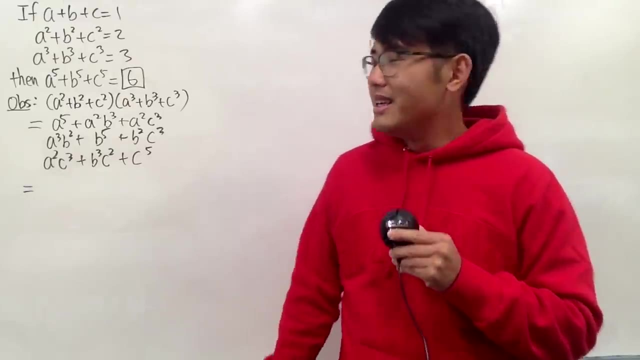 Of course, you can just like write down everything, but like no, that's not how you're going to do it. You're going to kind of organize the terms in a very nice way. okay, Let's see. 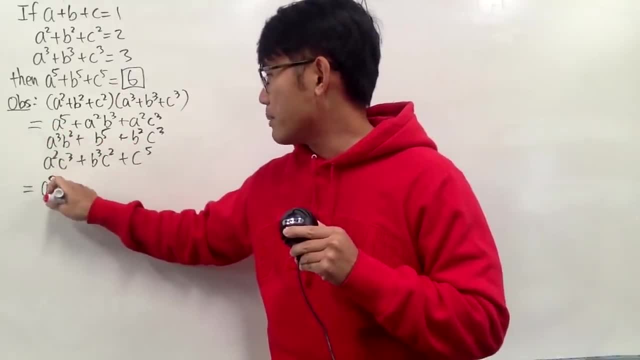 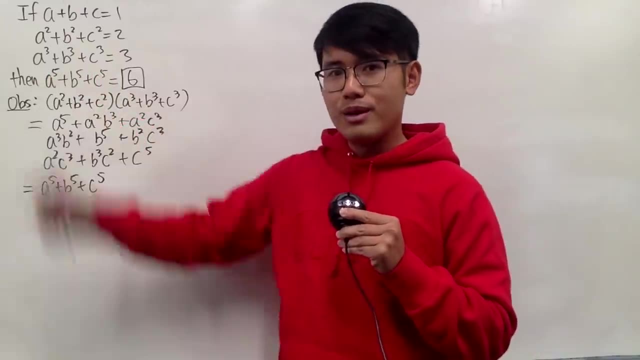 We have the fifth power right here, so that's good. So we have a to the fifth power, plus b to the fifth power, plus c to the fifth power, and that's exactly what we wanted to find right here And notice: if there's no other terms, then that would be really nice, because this is equal to this times that. 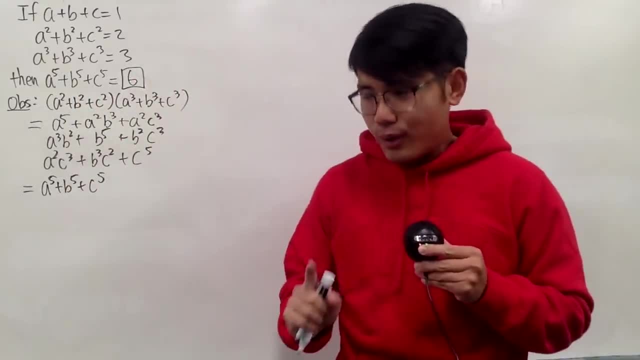 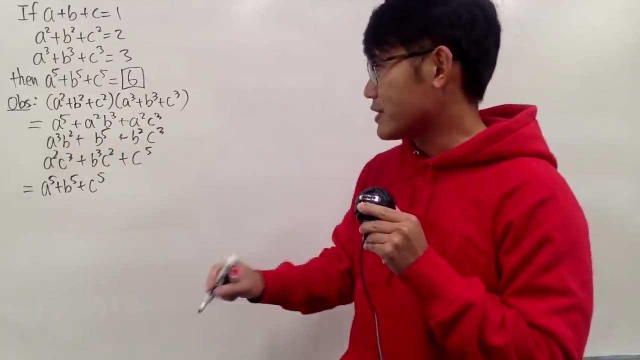 So two times three is six. you're done, But no, not quite. even though you get a six, but not quite seriously, You still have to face the real thing. In reality, we choose all the rest of the stuff. so check this out. 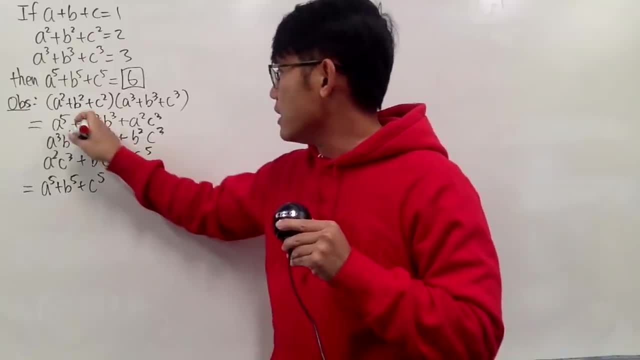 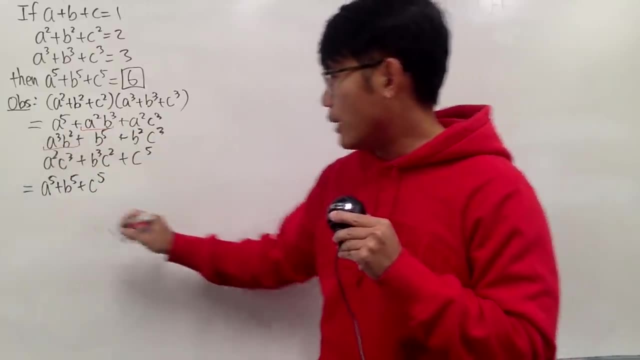 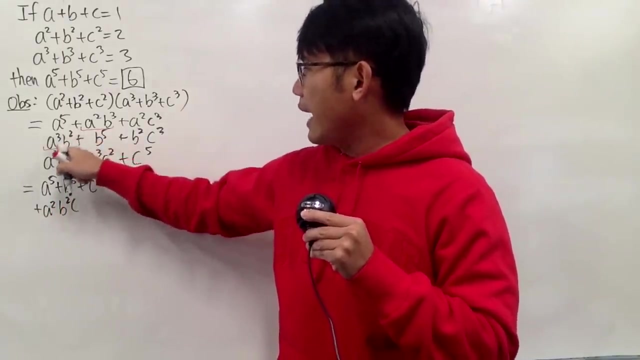 For this and that we can factor things out. So let's see, if you look at this and that we are going to factor out a squared and also b squared, right? So I will just write this down with plus a squared, b squared, and if you factor that out, we will end up with a plus b. 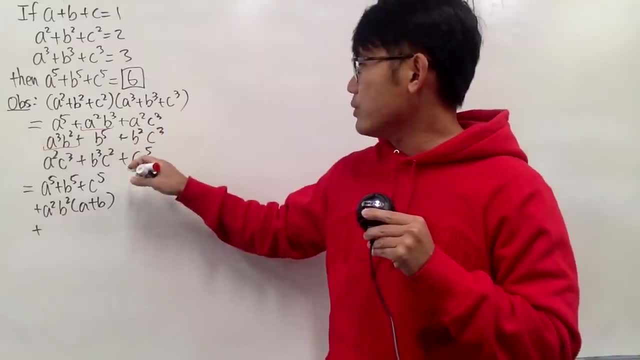 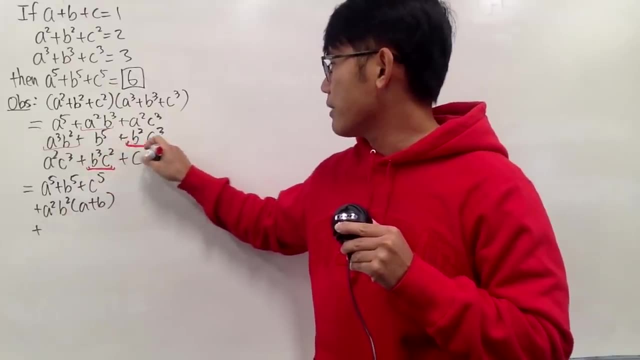 That's nice, it's not that bad. And then next I will do: Let's see if we can factor the b squared which is going to be right here And right here, you see, we have the b squared we can factor out. 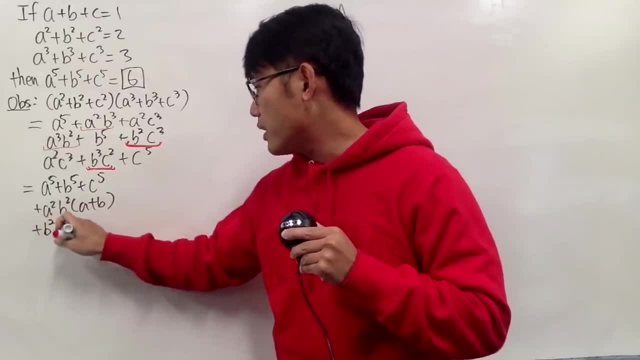 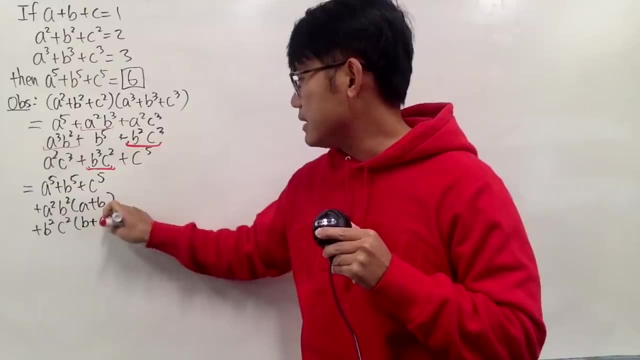 So in fact, the c squared too. so we can factor out b squared, c squared, and with that said, we will end up with b plus c. right Yeah, so we have b plus c. So that's also very nice. 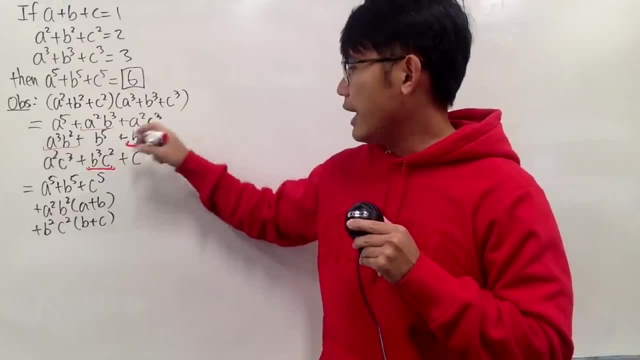 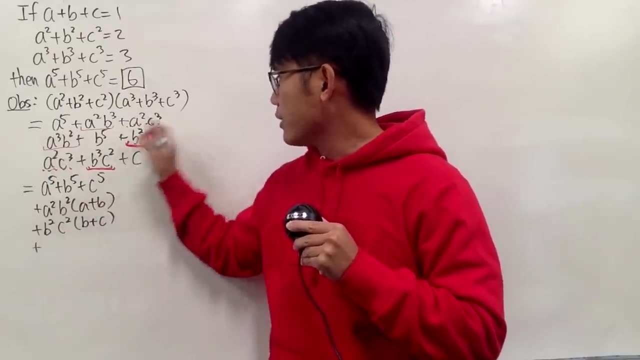 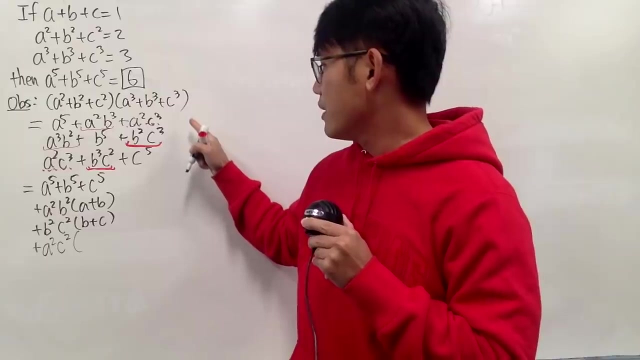 And we have this right here. we can also factor out a c squared, this and that. So the last one right here is a squared and also the c squared. So a squared, c squared and we have a plus c. 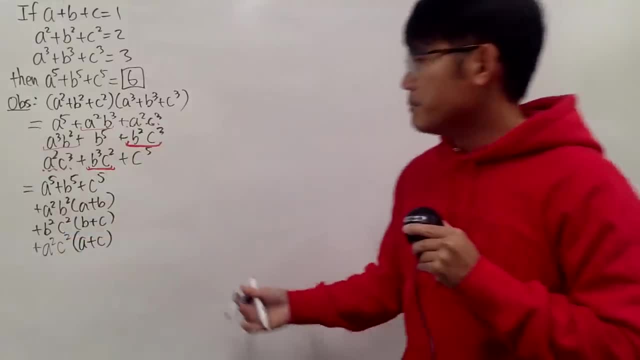 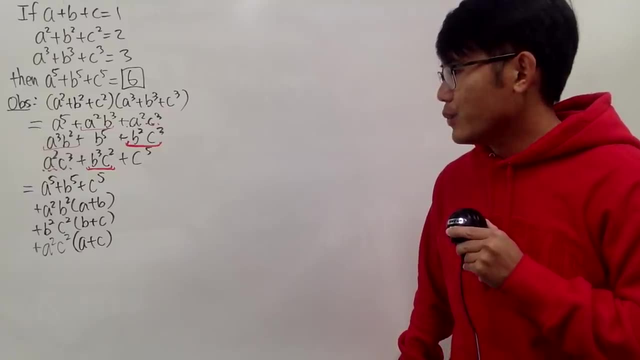 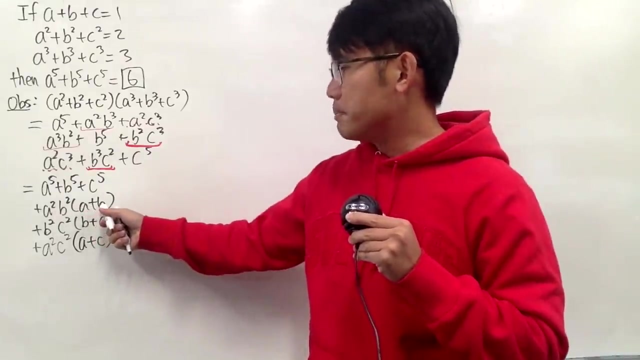 So you do have a very nice pattern, but let's see what can we do next, though We kind of need to figure out more things right here, huh? Well, a plus b, it's actually similar to the original equation, because, of course, 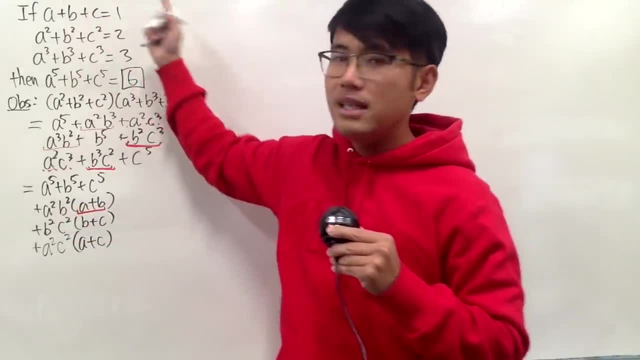 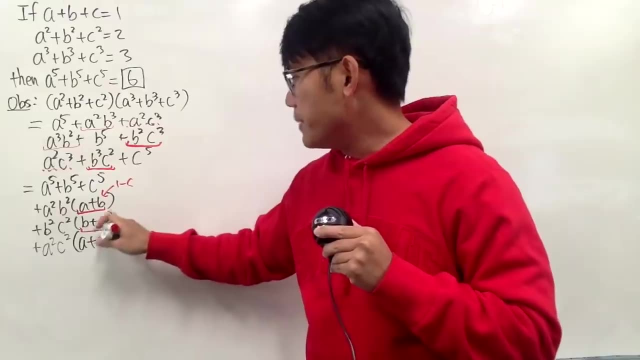 if you look at just the a plus b part, you can minus c on both sides, so this is just 1 minus c, right? So we know this right: here is just 1 minus c. And similarly, if you have b plus c, then we can just minus the a on both sides, so that's actually pretty good as well. 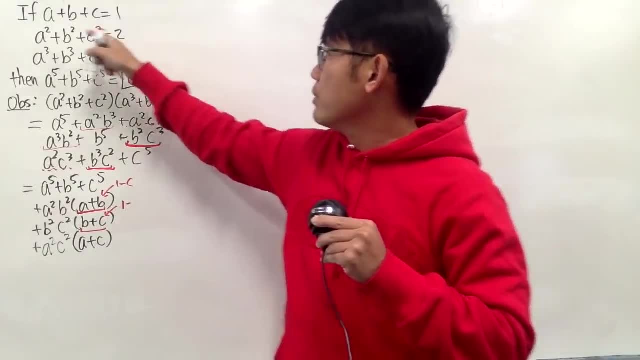 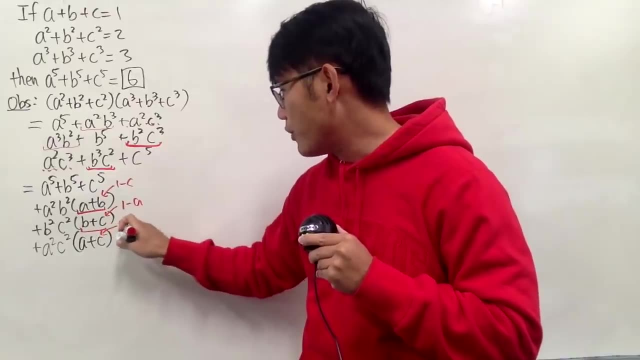 So we put down 1 minus a right, because we minus a on both sides, and then a plus c, we minus the b on both sides. So that is also very nice. Yeah, I think we are doing this right so far, which is pretty good. 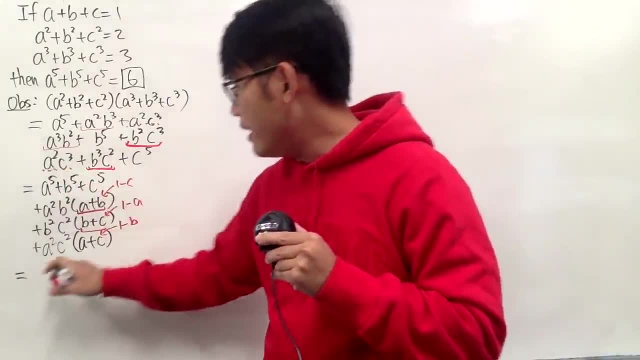 And now let's see, this is equal to, of course we still have the a to the 5th power, plus b to the 5th power, plus c to the 5th power, and all that. And now here's the deal. 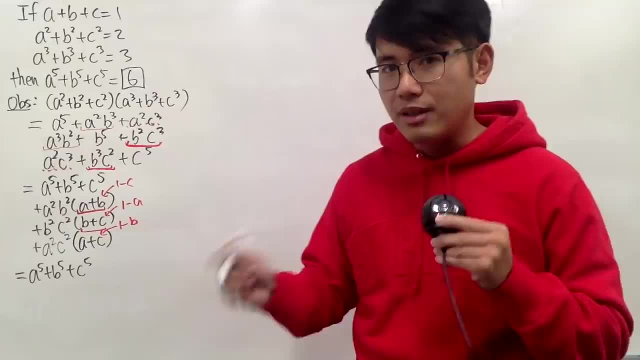 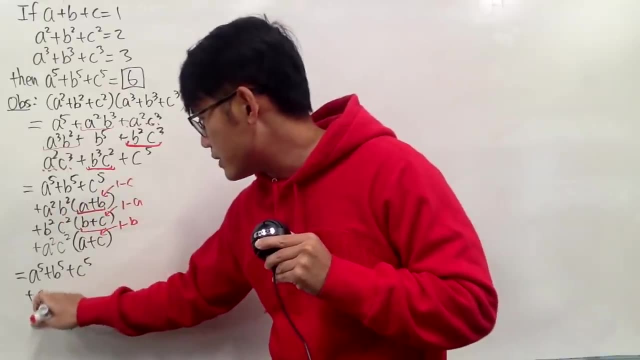 I will just multiply this and that and then we'll distribute to see what happens and hope for the best. seriously, So if we do this times that we get plus a squared b squared times 1, which is just that right: a squared b squared. 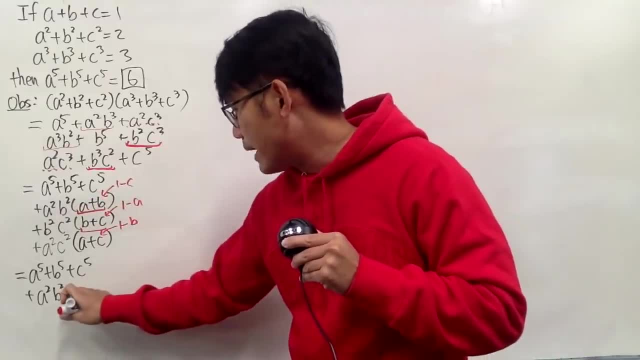 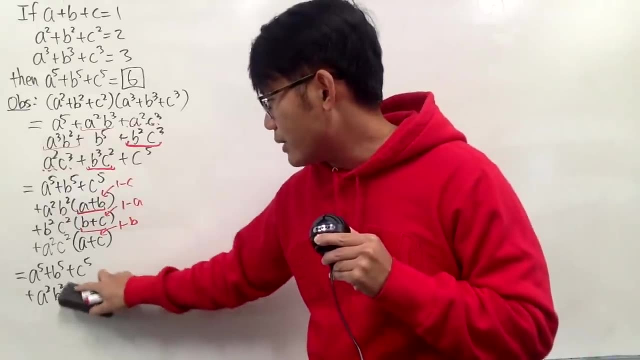 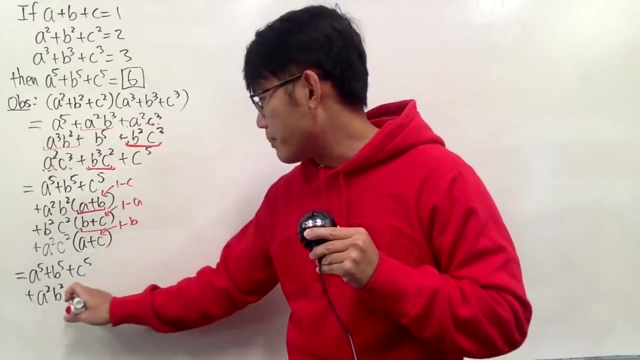 And then we will have this times that, so minus c, and let's see if we can do something in our head first. So let's do that, all the distributes of 1s first. okay, So we have this times 1, so that would be this part and this times the 1, we will have the plus b squared c squared part. 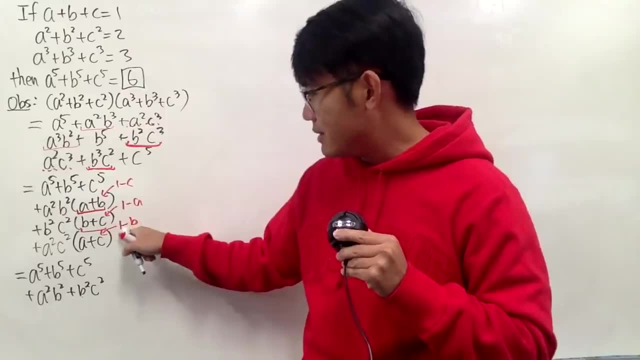 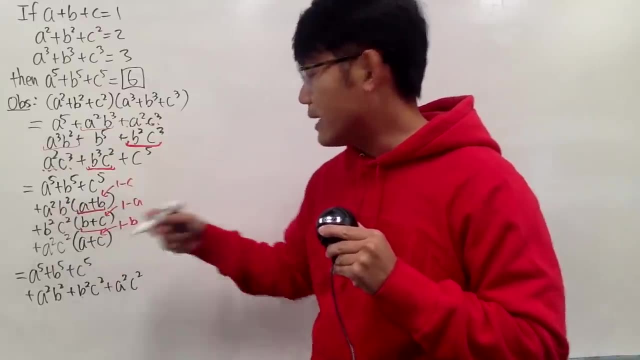 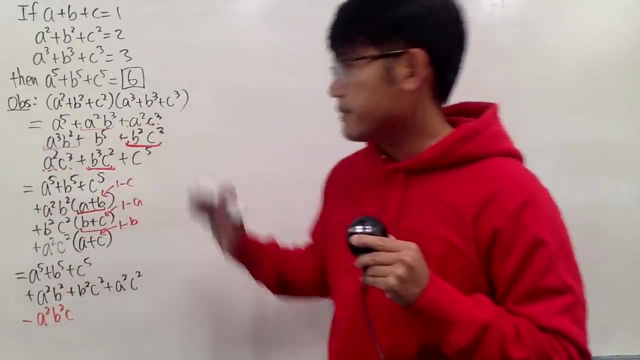 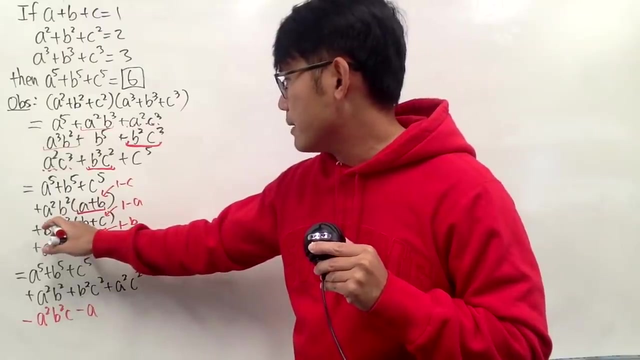 And we have ac squared, times the 1, so we have plus a squared, c squared. so that's very nice. But now we have to do this times that and that's minus, so we have to minus a squared, b squared, c, right, and we have this times that it's minus a, and we have the b squared, c squared. 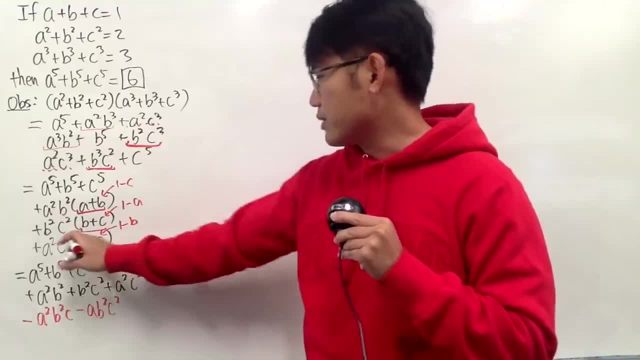 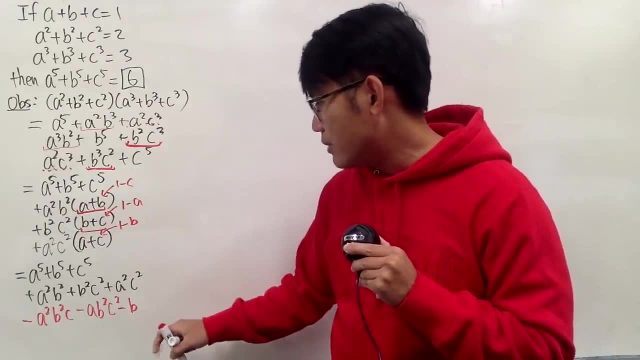 Oh, the a is kind of lonely, but it's okay. The c is only here too, so that's good. And then we have the a squared c squared times the minus b. so it's minus b. Let's put the b out. well, let's do it in order. we know our alphabets right. 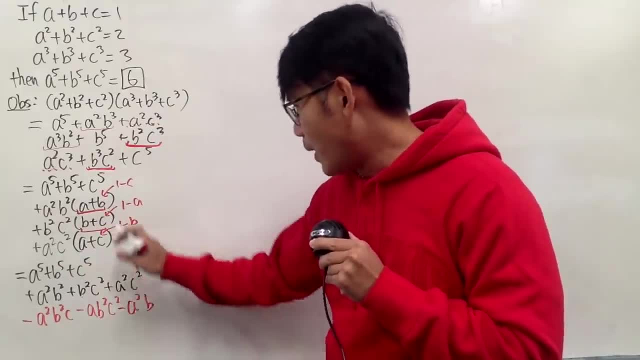 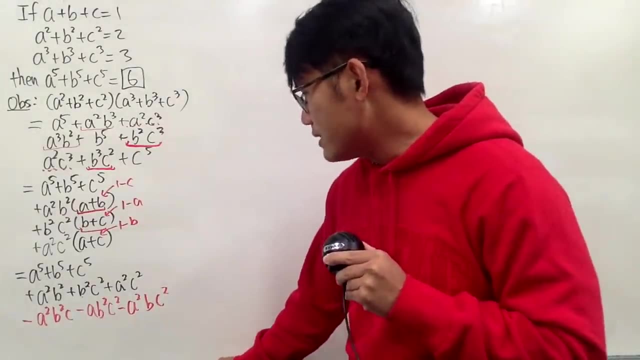 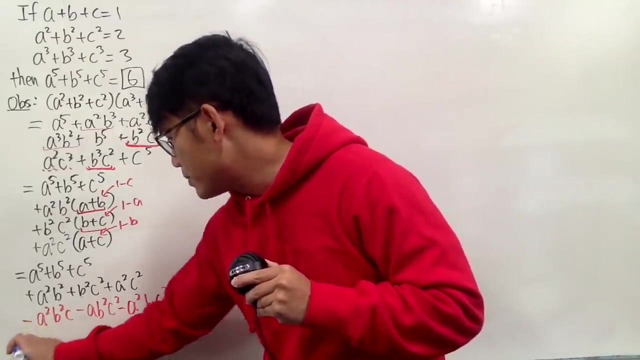 So let's do a squared b to the first power and then c to the second power. so that's what we have, And perhaps, if you just focus on the last part, all right. So if you just focus on the last part, this right here is the same. well, let me just put down this right here. 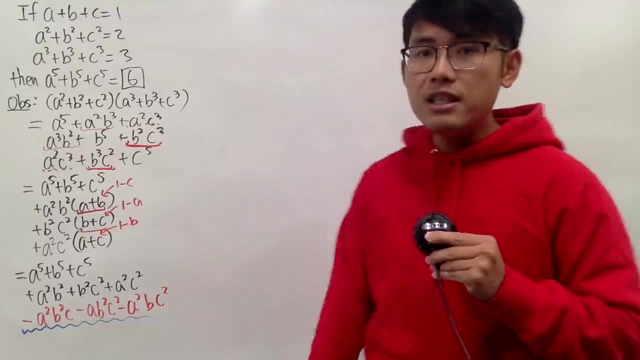 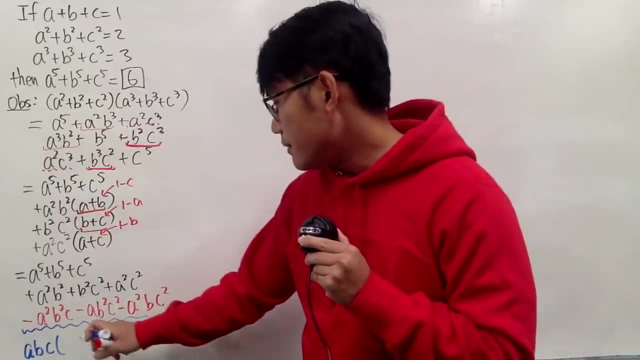 it's actually the same as we can factor out a b c, right? Perhaps I will also title this as a b c equation. oh, no man. so if you factor out a b c, then let's see, we'll have. 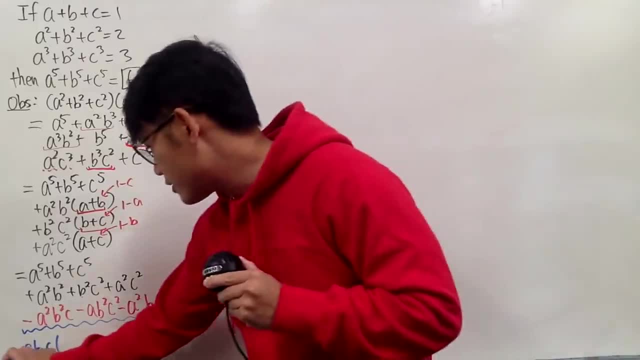 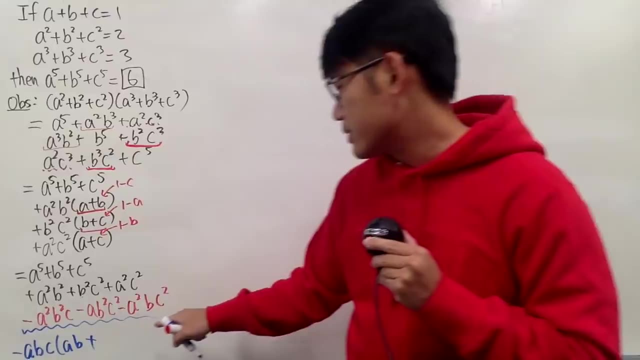 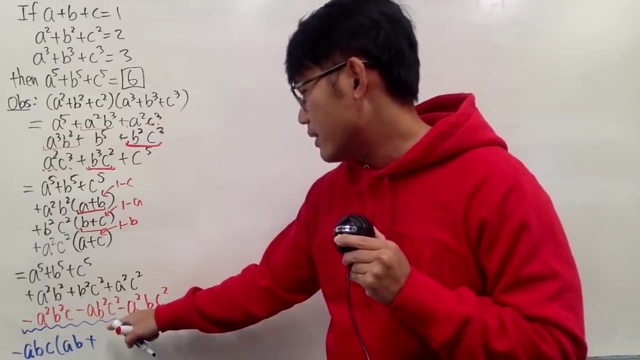 Minus. perhaps let's factor the minus as well, okay, Well, good huh, So minus and we will have ab right here, and then plus we factor out. Yeah, the c's out, and then Oh, yeah, so in this case we factor a, b, c, what Hold on? 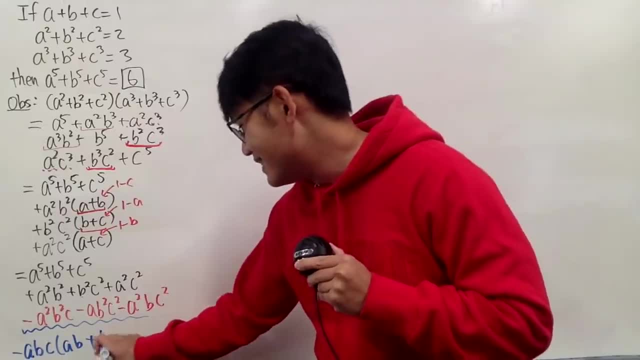 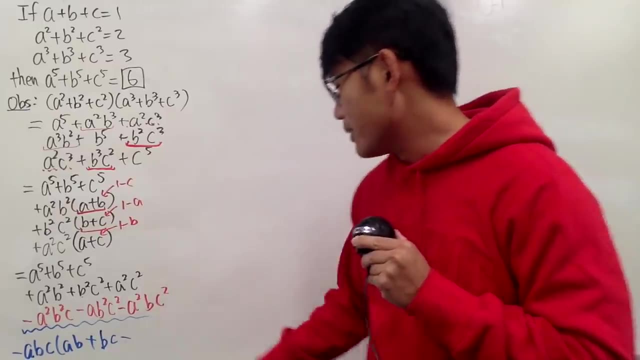 A. Oh yeah, yeah, yeah, yeah. we have b, c, And then next we have minus, and then the ac, A, B, C is out, so we have the B is out, so we have A, C, and then this is the plus, like that. 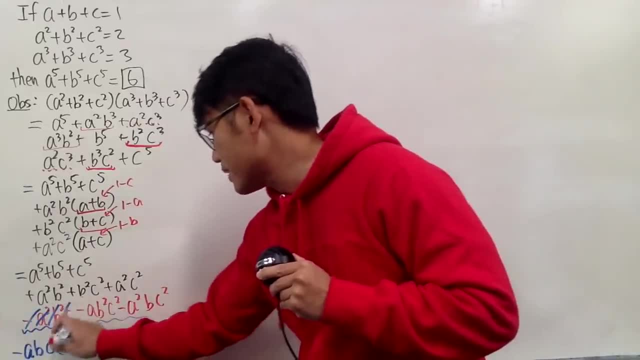 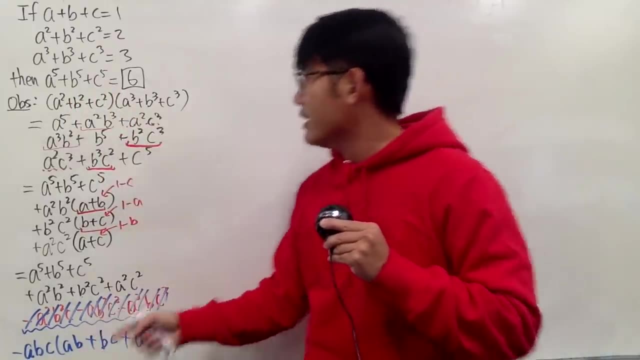 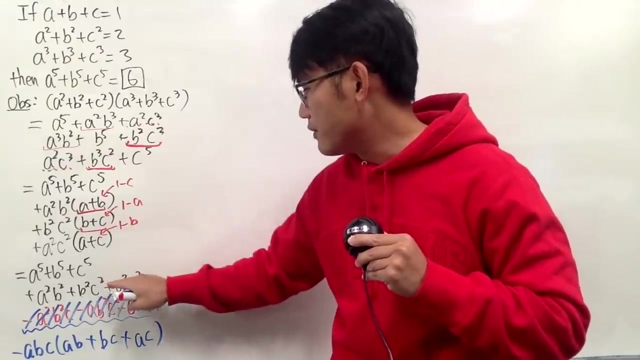 So instead of looking at the red, we'll look at the blue part, because we factored the out already. So now we know that if you multiply this and that we get all this, Let's see we have 1, 2,, 3,, 4,, 5,, 6,, 7,, 8,, 9, 10,, 11,, 12,, 13,, 14,, 15,, 16.. 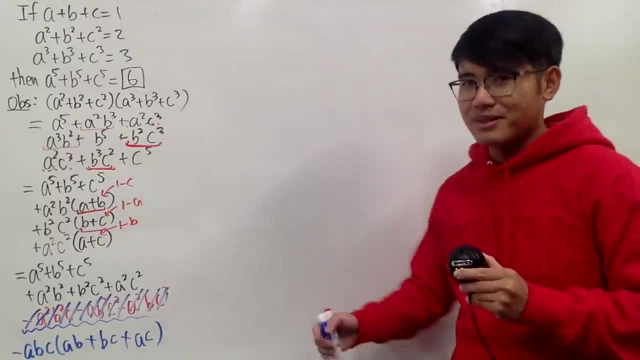 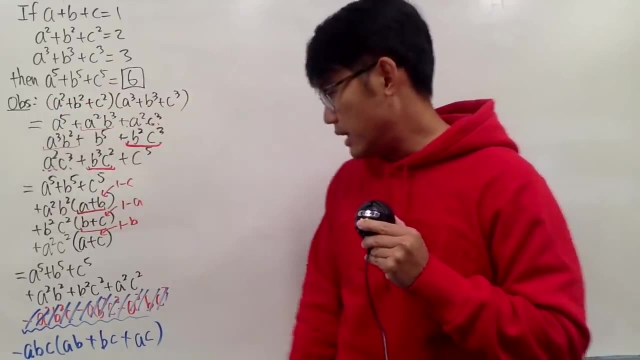 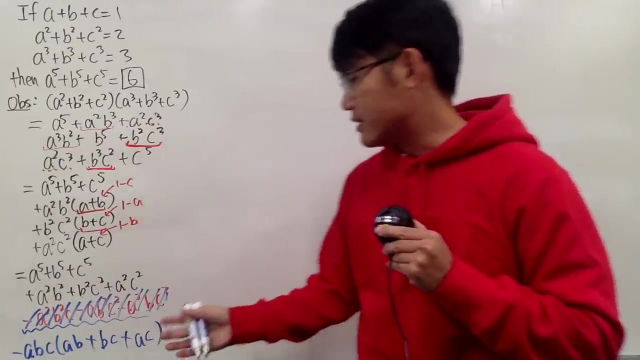 16 times. I think that this is my record, but you know we'll see. Alright, here's the deal. I know the value for this expression is 2,, this is 3, and if we know that, that would be good. but we don't know A, B, C, we don't know this guy, so we have to do more work. 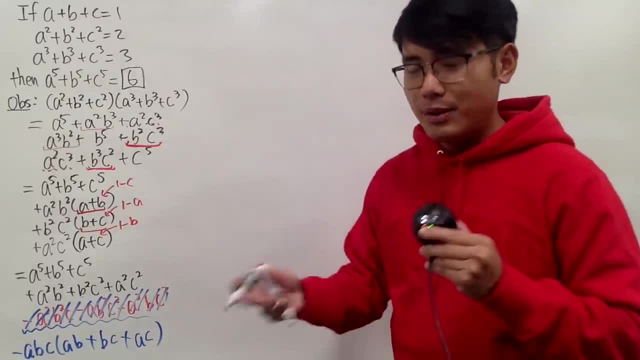 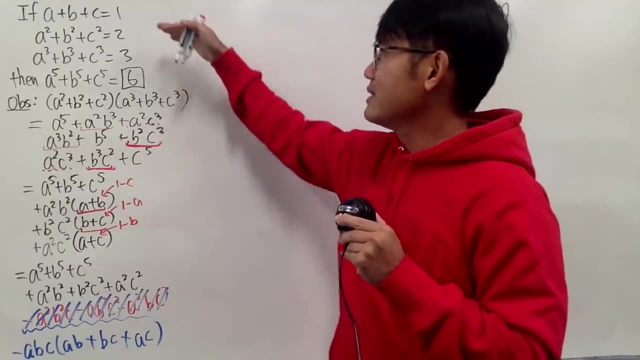 How can we do it? Well, we have to use the other equations and we actually have to do the squares, both sides, And all that, things we also have to utilize. yeah, let's use the first one. so let's see. 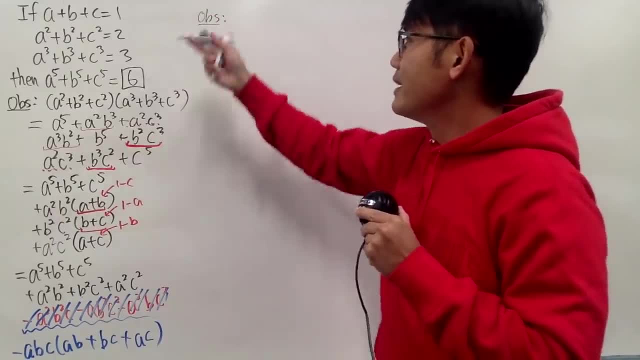 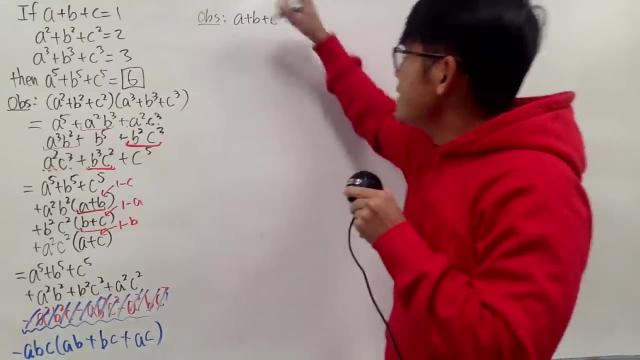 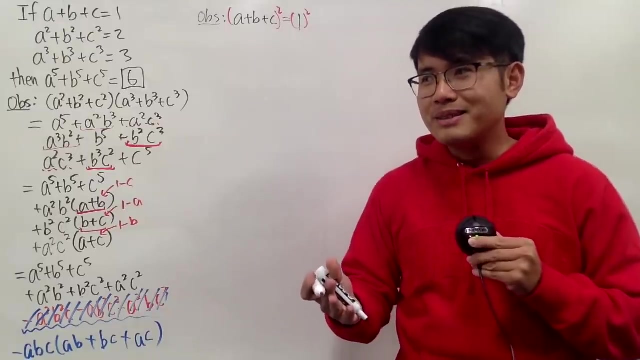 I will look at more observation. right, observe: If we have A plus B plus C equals 1, okay, that's square both sides. and look at, this is the trinomial when you square both sides. In fact, you do have a nice formula. I don't know if I should say nice. 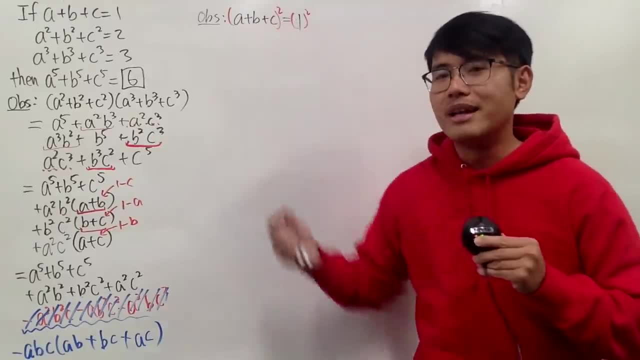 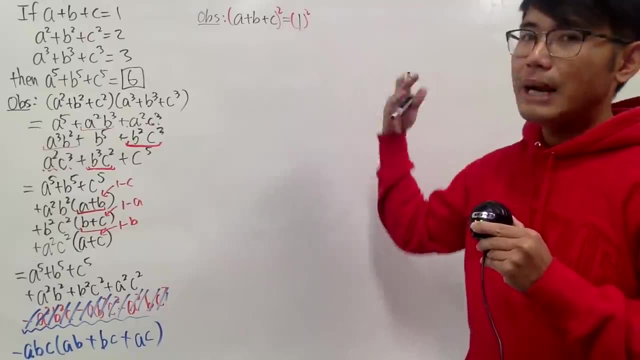 When you have a trinomial to a power, And this is called the trinomial expansion formula, just like the binomial expansion. But for this one it's seriously up to you how you want to do it. This right here is still not that bad, so we'll probably just do it by hand. 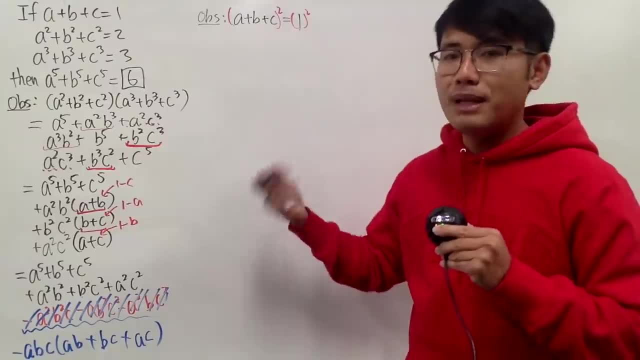 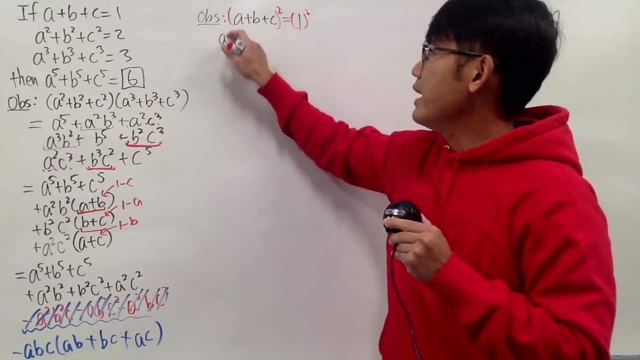 So this is the same as saying A plus B plus C times A plus B plus C. so you can do this in your head and you can just get the following: You will get A squared plus well, it's like A. let me just write it down for you guys. 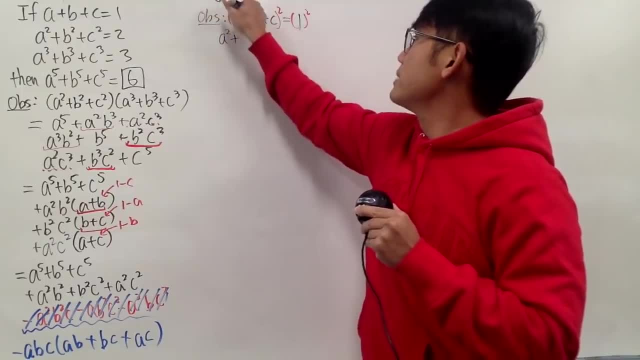 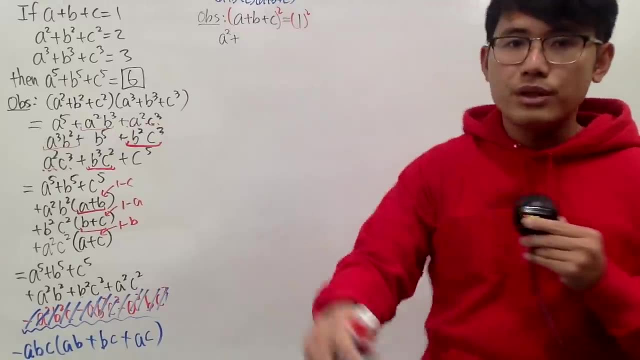 I think you can do it. You can still see it right here. so this is A plus B plus C times A plus B plus C, right? So let me just make sure that you guys can see this right here first. Not really, huh? 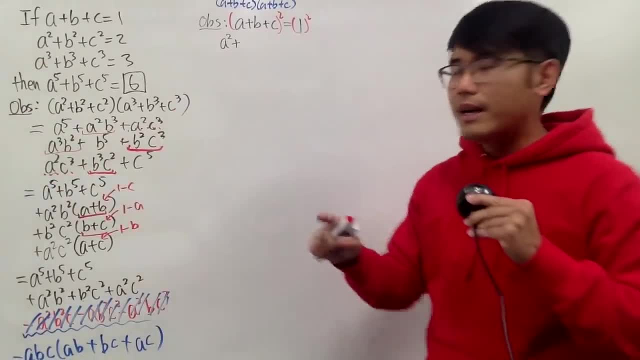 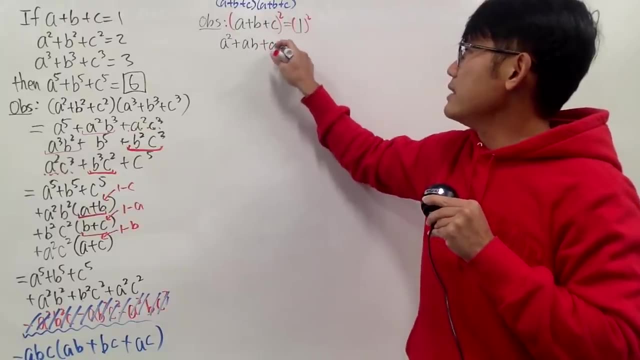 So I don't know, it's just kind of: oh okay, cool, Alright, so you just do this times that which is A squared, and then you do this times that which is plus AB, this times that is plus AC. 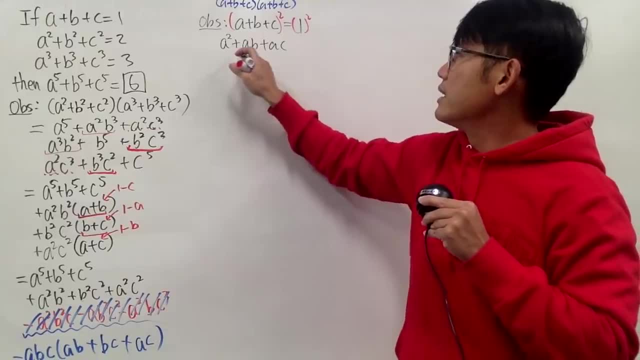 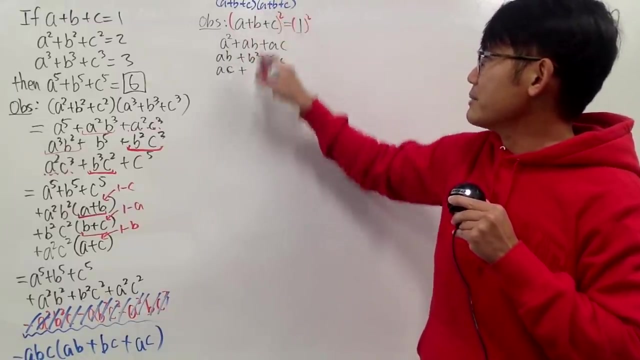 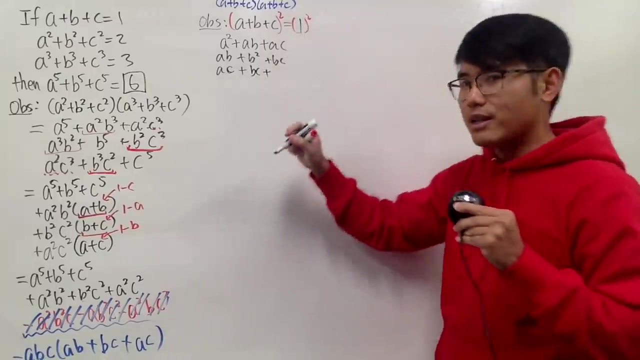 It's really similar to that. so this times that, and you get AB, And then you get plus B squared, and then you get plus BC, and last one, you get AC plus B times. no C times that. so C BC, sorry BC, and plus C squared, like all this. 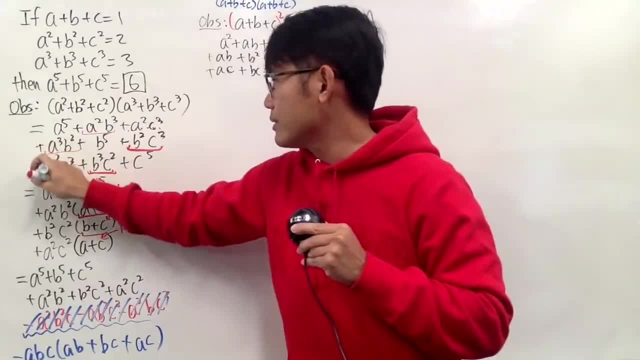 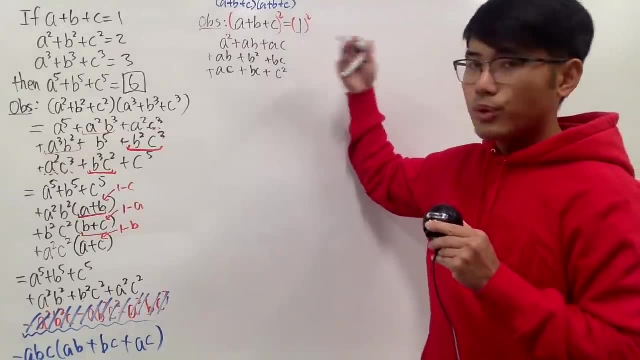 And technically I should put down the plus signs along the side here. I forgot about that earlier, but this is okay now. It's not that bad. This is equal to 1, and the deal is that you see that we have the A squares. 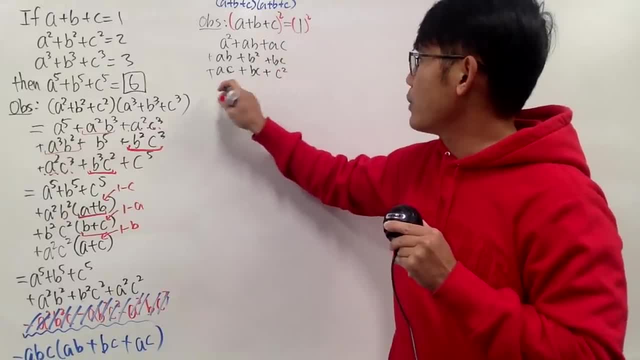 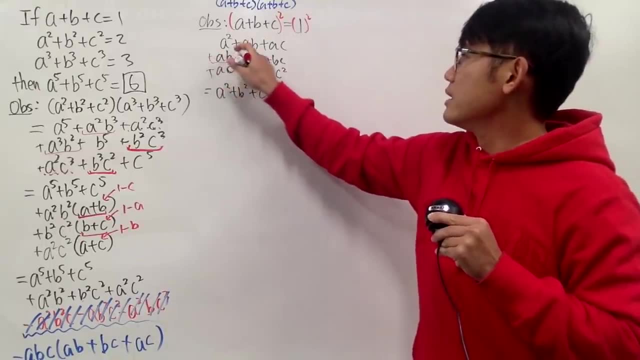 Okay, let's see what will happen. We have the A squares, so I will write this down as A squared plus B squared plus C squared, And you will just see this is, you know, combinable. We will just combine like terms. 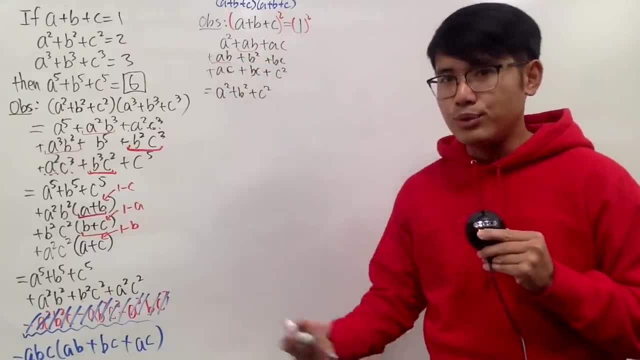 You have two of this, two of that, two of that, Everybody has the two, two, twos, right? So of course we can factor all the twos. so we put down plus two And this, and that we'll just put down the A. 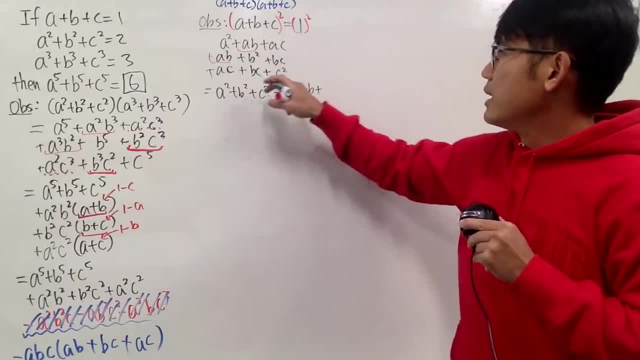 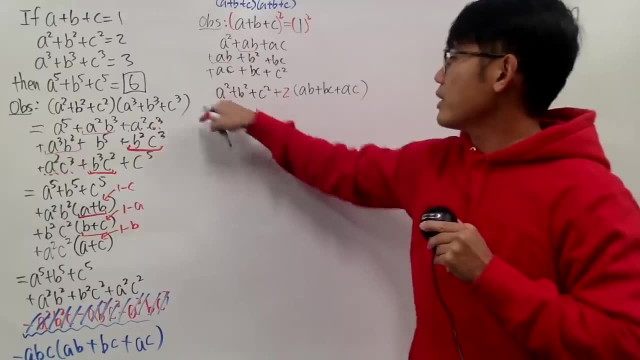 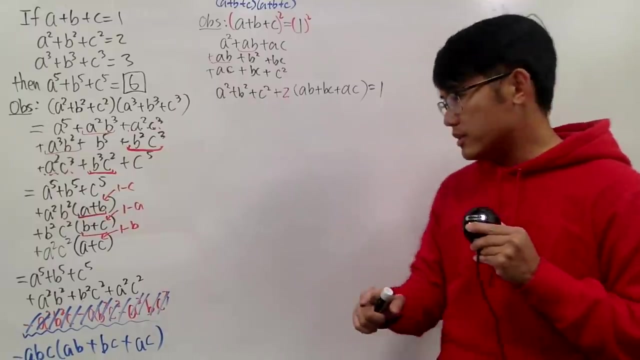 A, B, and the next one is plus BC, and then last D plus the AC, like this, And this right here will still be equal to 1, right, Because this is just the expansion for that. So that's not that bad, because now you can actually solve for this part. 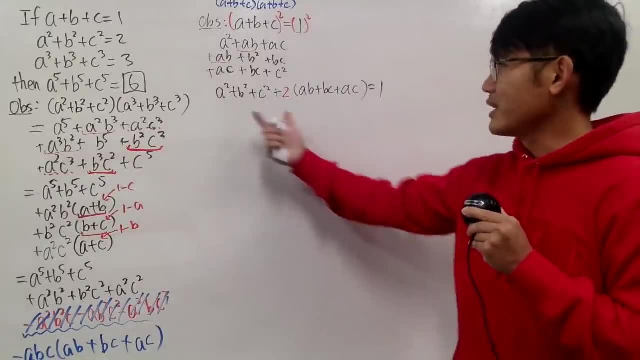 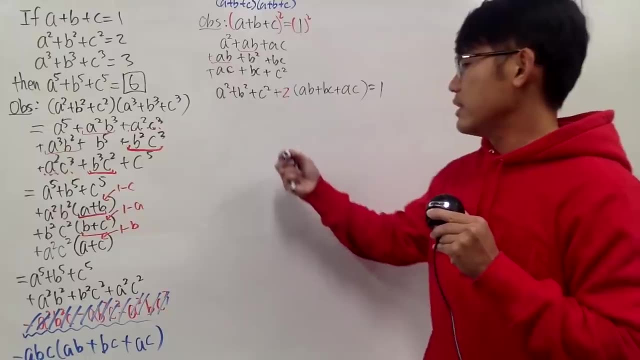 Really cool, huh. So I told you it's just a lot of algebra for that. We know this guy is just 2, so that's nice, Very nice, All right. So this right here is just 2.. Why? 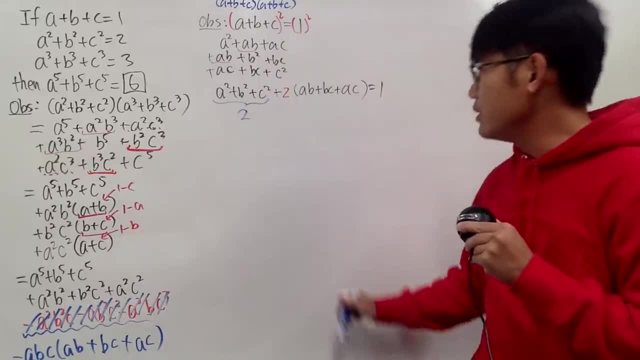 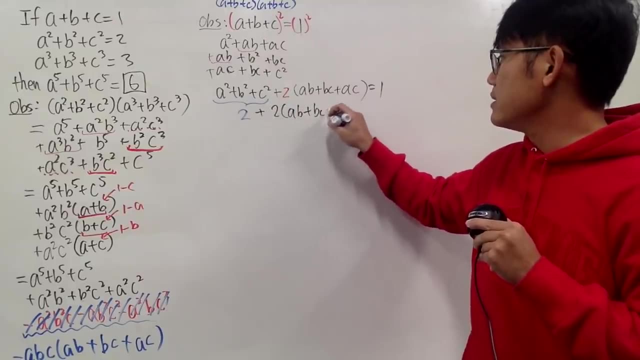 Thank God. right there, the equation gives us just a- 2, which is really really good. And then plus, this is 2 again, because you have to combine all the terms A, B plus BC plus AC, and this is equal to 1.. 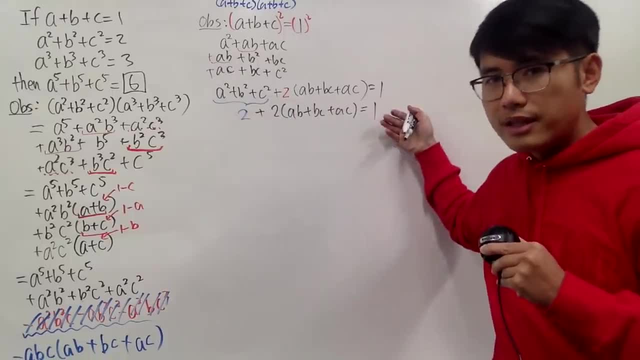 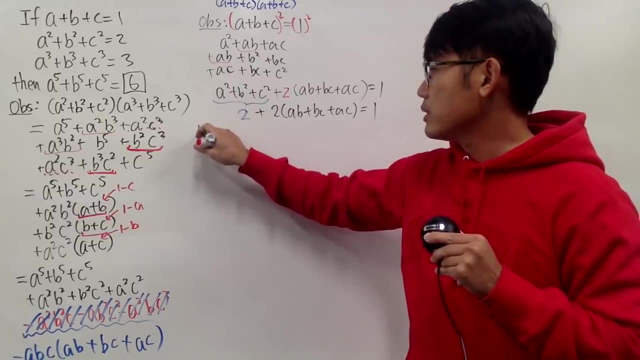 And now let's do a few things in our head. Minus 2 on both sides, you get negative 1. Divide 2 on both sides. so we know, Let me just first put down now. we know, Put down no. 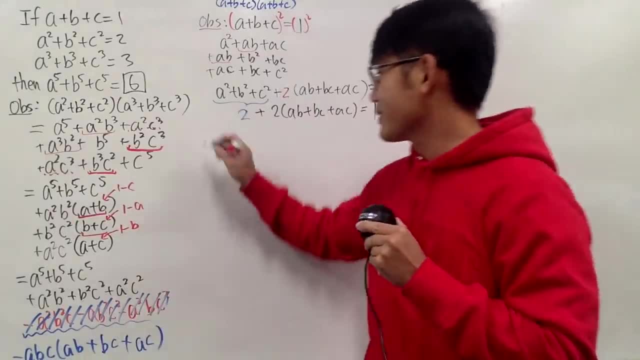 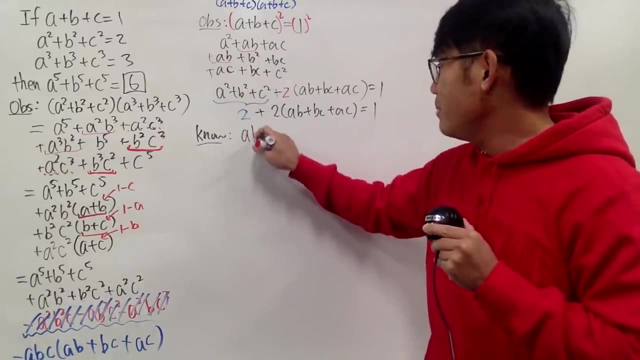 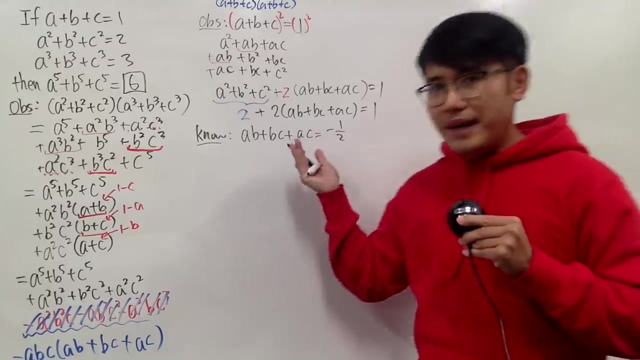 No, I mean I want to put down: we know Now, we know this guy is equal to negative 1 half. Oh my God, A, B plus BC plus AC is equal to negative 1 half. So if I put in here then the last part, I need to figure out just the ABC, then we'll be done right. 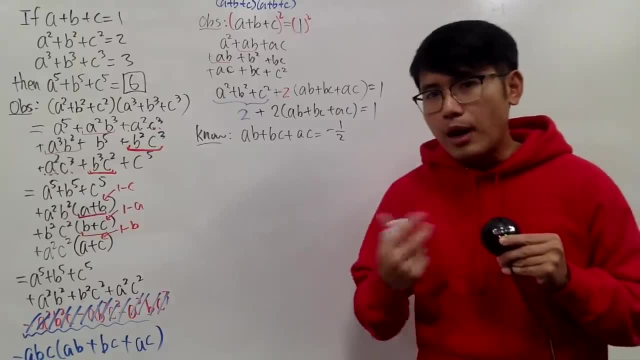 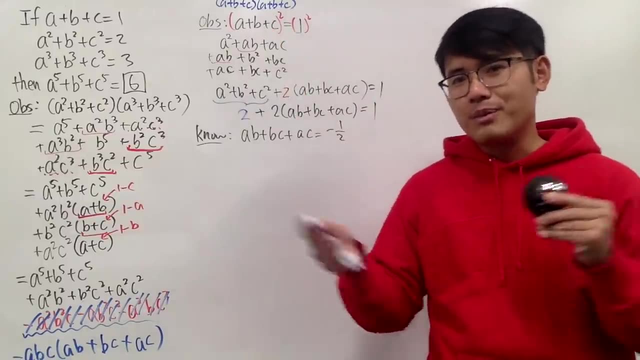 So huh, here is the deal. How can we produce A times B times C? The truth is that we will have to raise this to the third power. That's how we can actually, yeah, get A multiplied with the C multiplied with the B, all that. 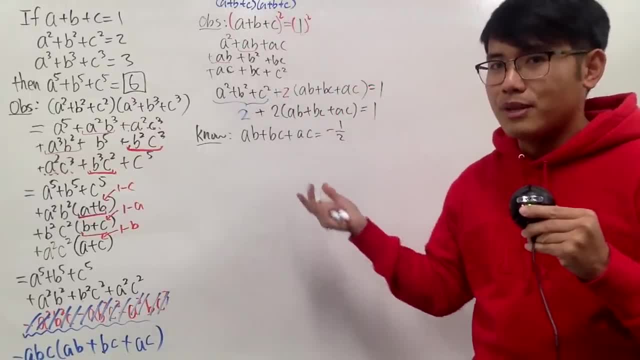 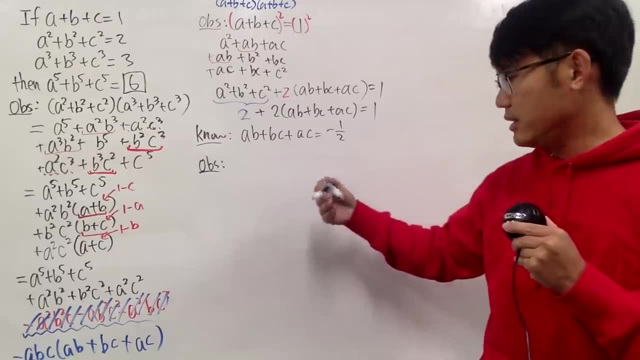 Because if you look at this earlier, it's just actually two-dimensional multiplication. We have to have the three things together. So now another observation. So perhaps I will box this in red. I think this is rather important, so I will box it. 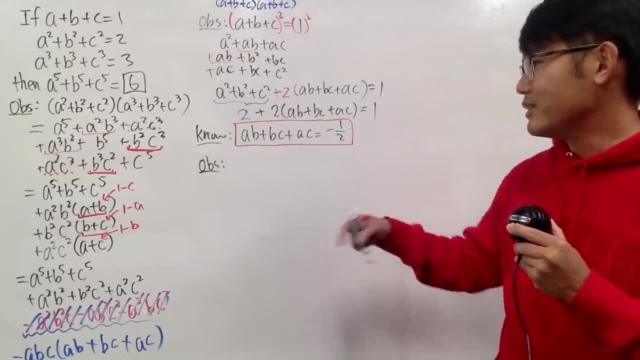 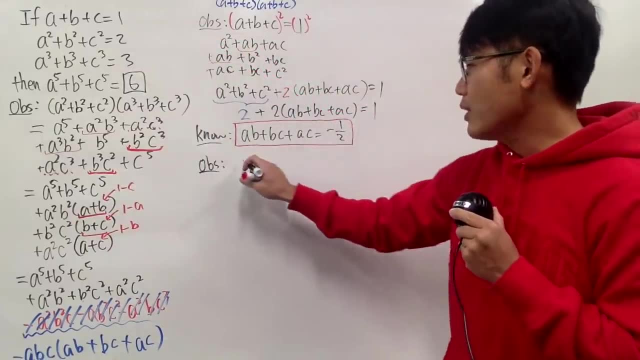 And of course you can come with a lot of identity. It's already, but you know, just show you guys all this. So observation: raise both sides of this equation to the third power, So A plus B plus C. 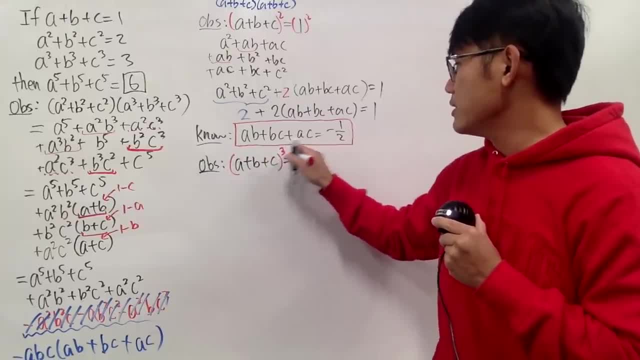 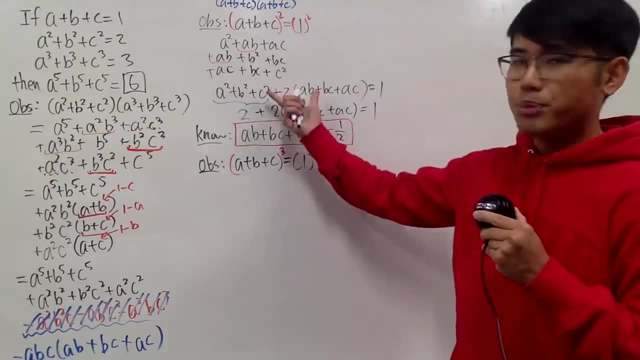 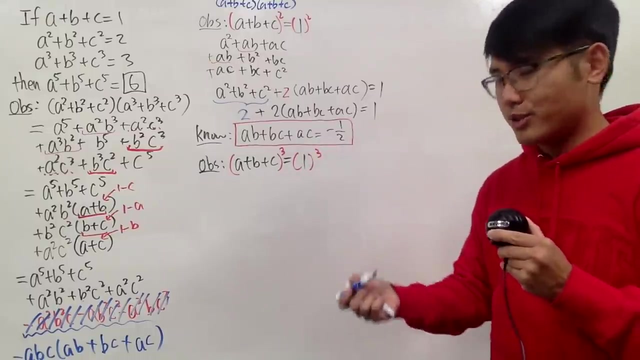 And we know this is equal to 1.. Again, we raise both sides to the third power. Okay, you have two choices. One is you can just multiply this expression by another- A plus B plus C- Or another thing is that you can learn some new things, which is the one I will show you. 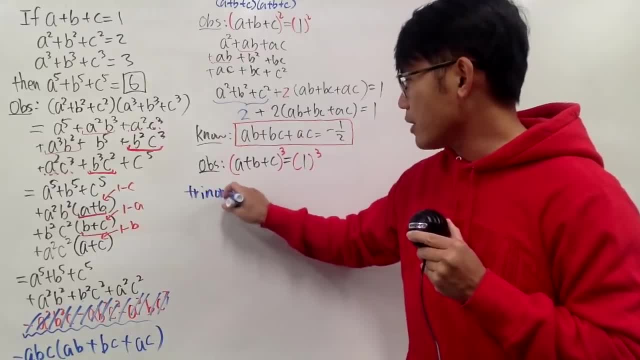 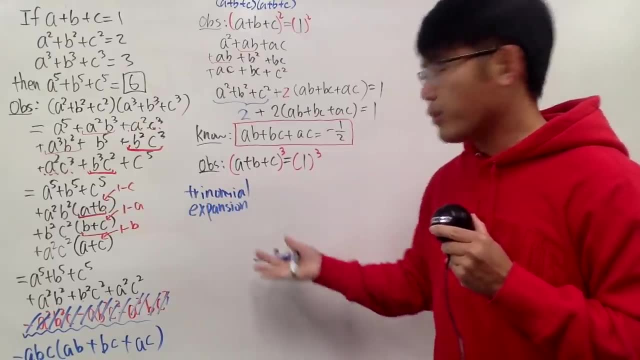 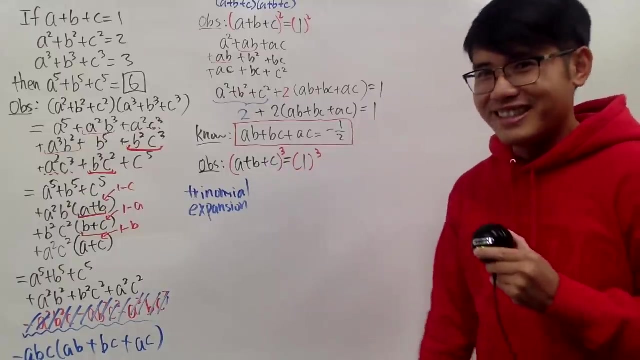 So let's do it. So this is called the trinomial expansion formula. It's really cool, but, to be honest, sometimes maybe you just want to end up with just multiply this three times on your own instead of using the trinomial formula. 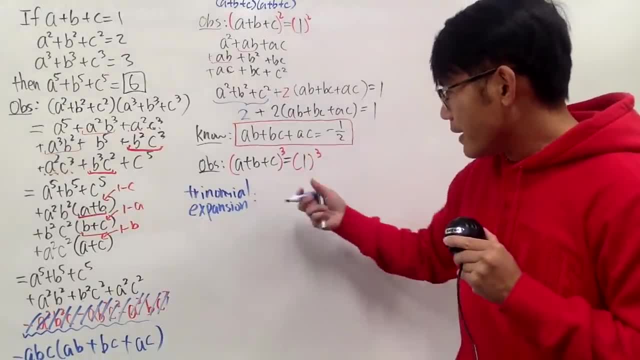 So I just want to be honest with you guys. but here's the deal, okay. So the statement says: if you have A plus B plus C, again, this is just a trinomial right. So A plus B. 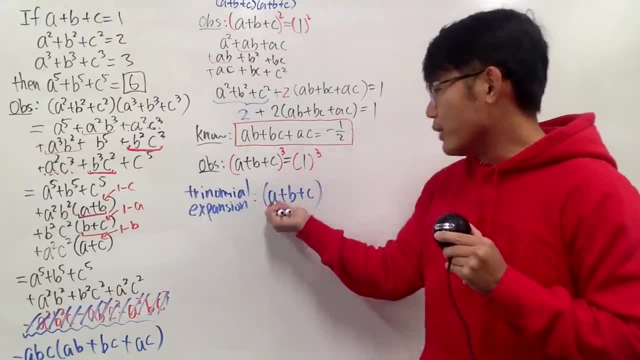 B plus C, And sometimes you may have more things, such as, like you know, 2X plus like 5Y and then minus, like 2Z or like 7Z or something like that. 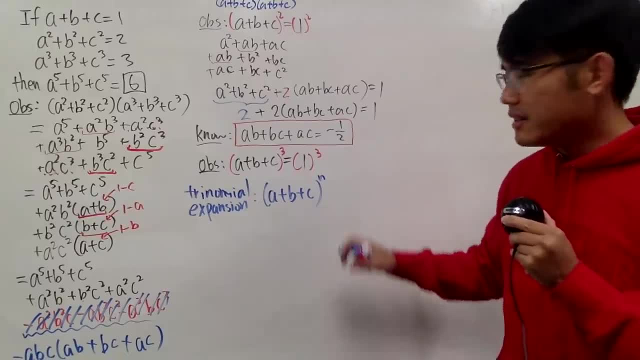 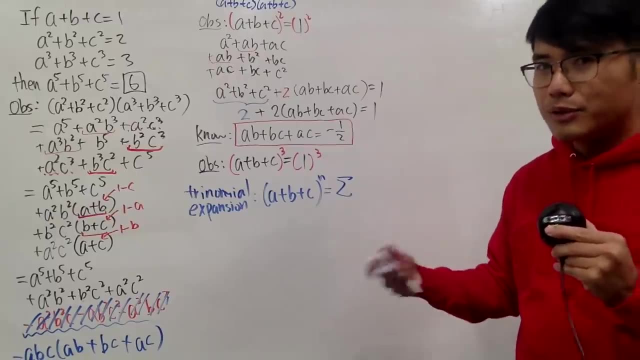 I don't know. Next we have this raised to the nth power. Then in this case we know this is equal to the sum And because you have three things, so you actually have to use like three indexes. 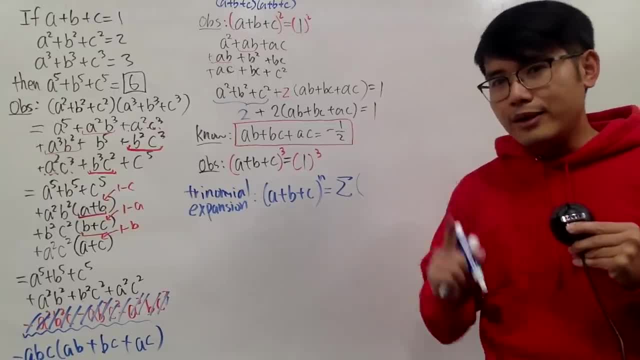 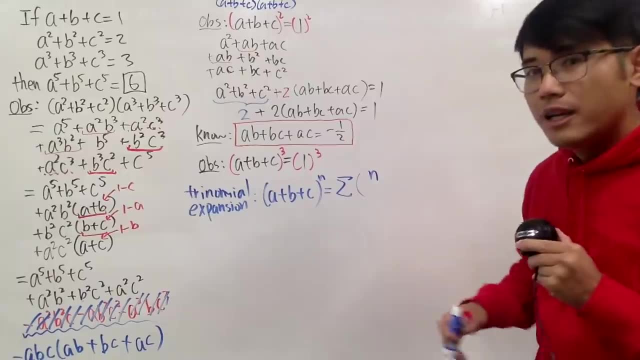 What you're going to do is, first of all, you are going to use the trinomial coefficients- Not the binomial coefficients, but the trinomial coefficients- And what you do is you look at this And again, you are going to use three indexes. 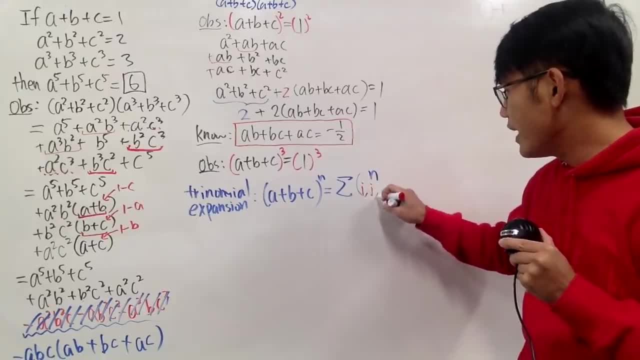 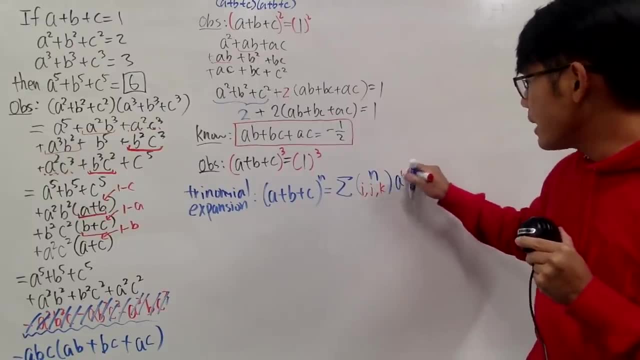 Indexes or however, And I'll just call it to be IJK, Okay, Not IDK, but IJK. And then you are going to have A to the I's power, B to the J's power and K to the no, C to the K's power. 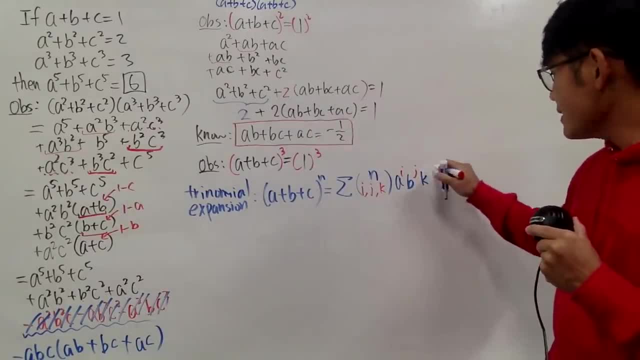 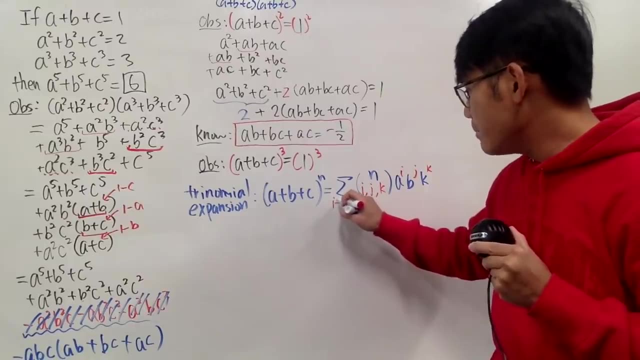 Like all this, Whew, Okay, And what's the connection between A? I mean, what's the connection between IJK? Well, the connection is that A plus J plus K, they have to add up to be N. 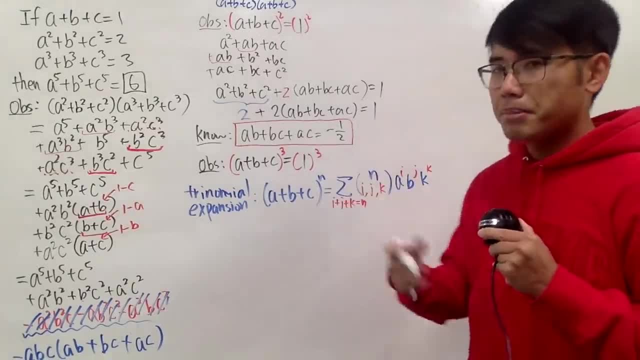 And of course, for now let's just talk about this as N being positive whole number. If N is 0,, that's like the best day ever. If this is 0,, then of course we know the answer. 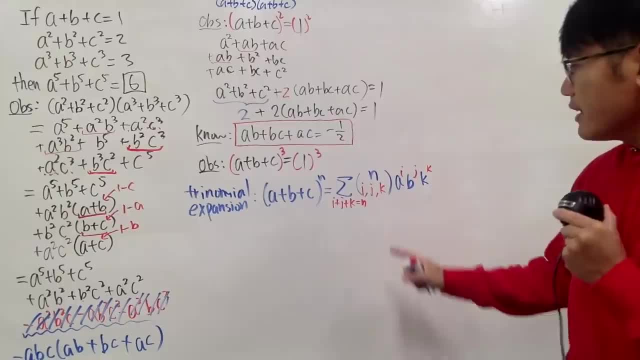 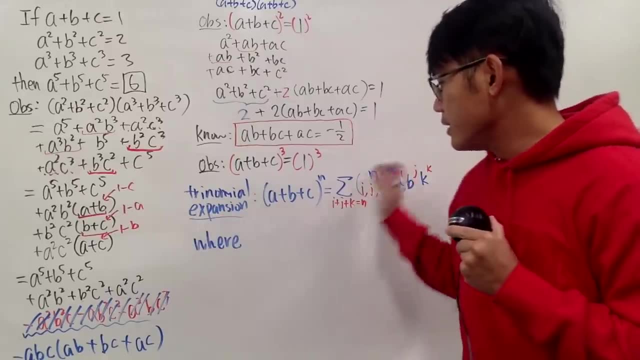 It's very nice, It's just equal to 1.. And let's say it's also 0.. And another thing I have to tell you guys is that: what is this, then, right? So I will have to tell you where the trinomial coefficient is. 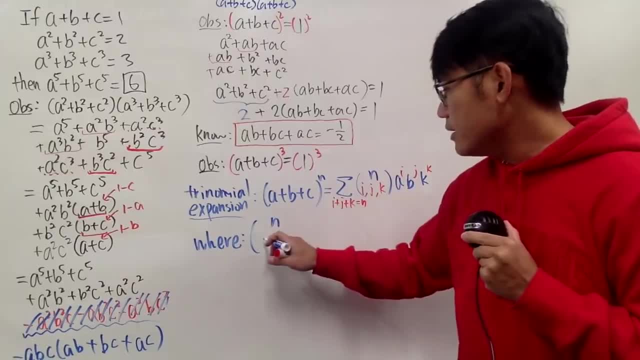 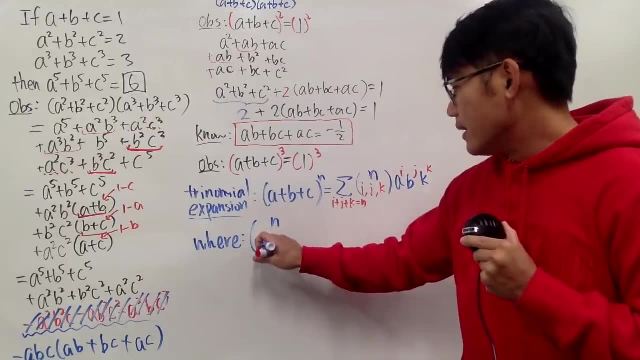 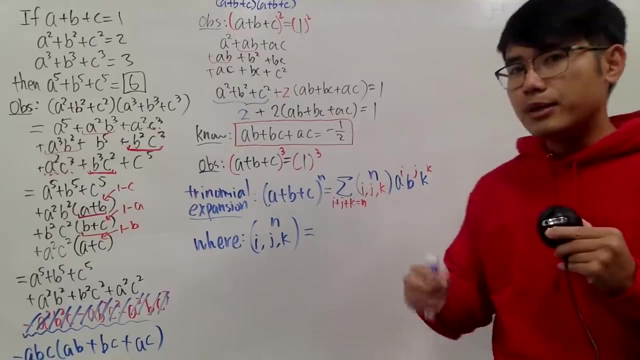 I'll create it as the following way: N- and I don't know how to say this. like N choose IJK, I don't know. But like I'll just put down N IJK. This right here to compute it, it's really similar to the binomial coefficient. 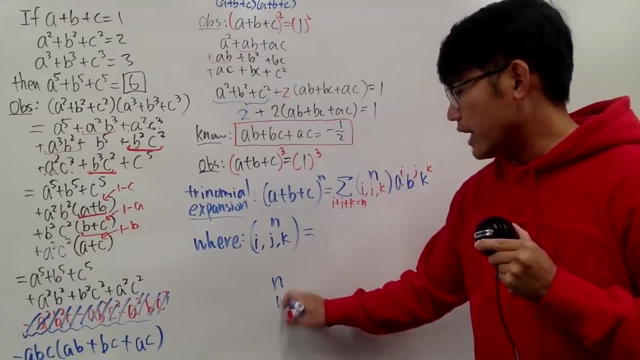 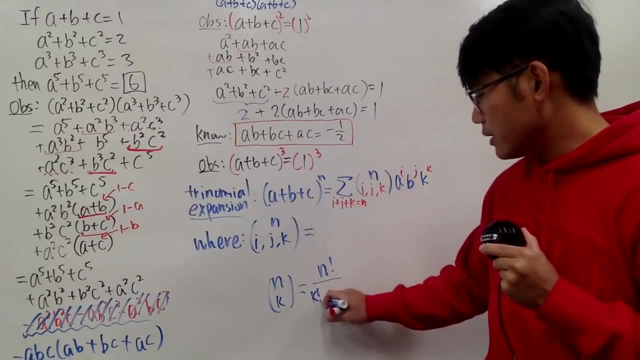 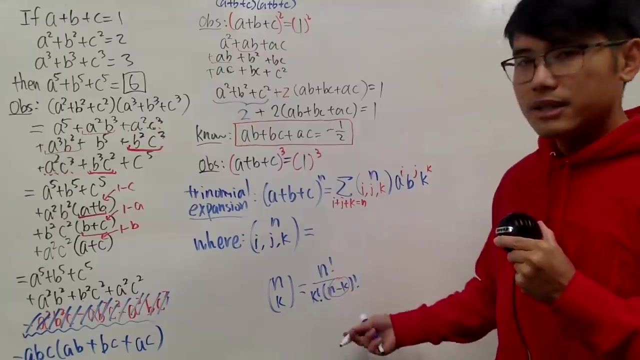 If you look at N, choose K. for example, this right here the binomial coefficient is N factorial times K factorial times N minus K factorial right. But the deal is that if you can code this to be something else, let's say you have a J. 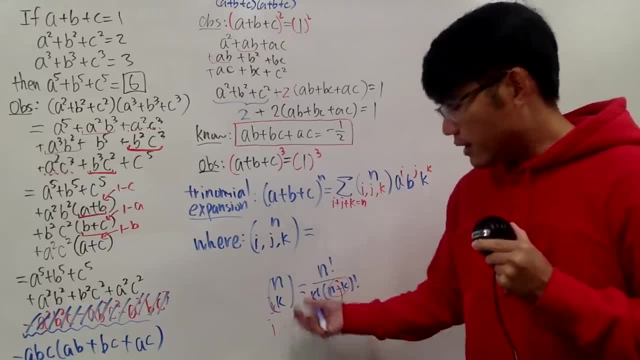 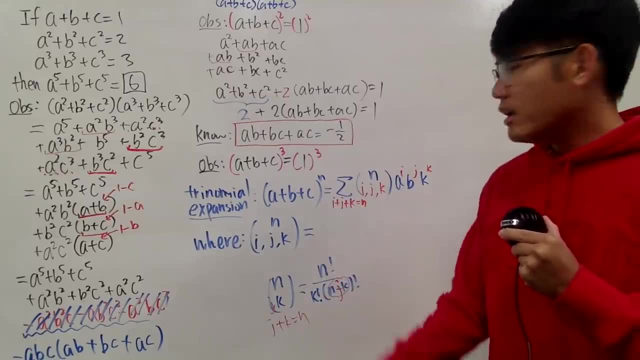 So you can code this to be J, where J is well the number, so that J plus K is equal to N. Then it's just N factorial over J factorial times, K factorial. Now you have three things. It's the same idea. 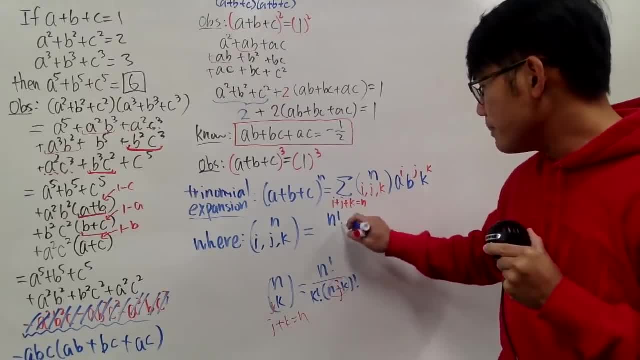 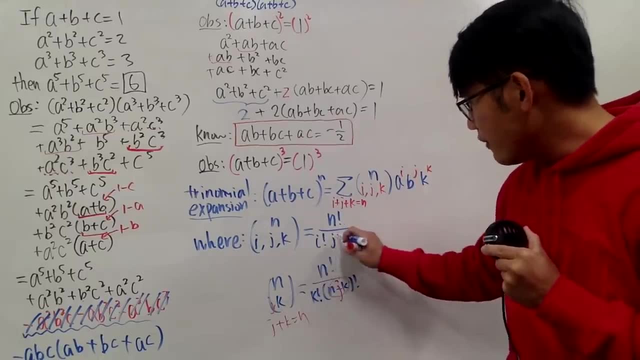 You are going to do N factorial divided by I factorial. Of course this is not the imaginary number I, so don't get too excited. And then you have the J factorial and then the K factorial. okay, So that's how you compute it. 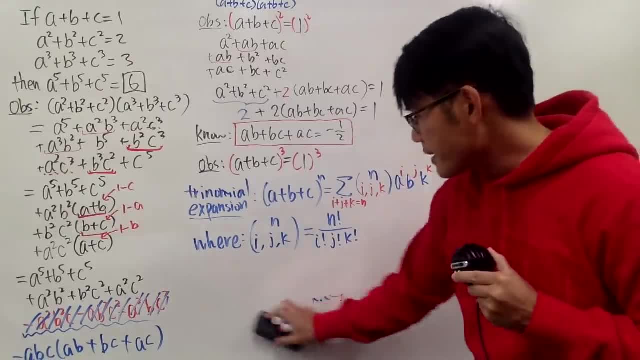 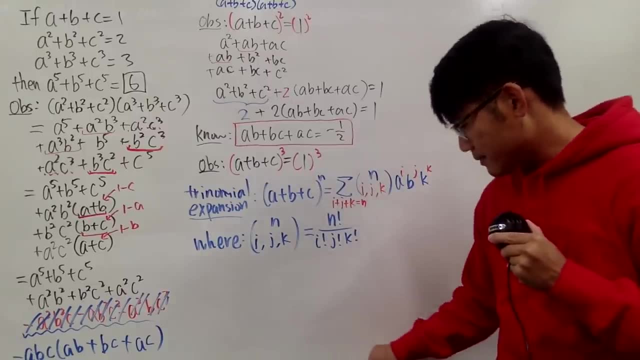 Very similar to the binomial coefficient if you look at it this way. Okay, Now, how exactly are we going to do this, though, Let's see, Calm down first, Because, seriously, we need to. let's see, let's see, let's see. 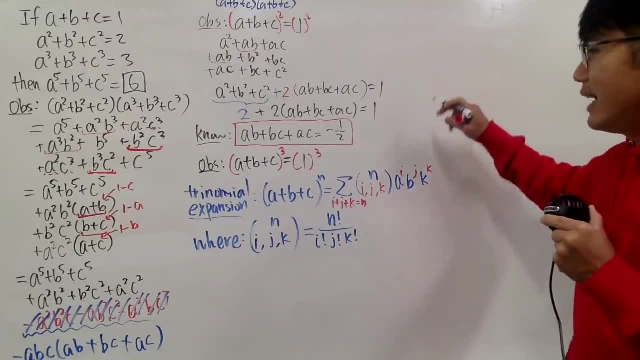 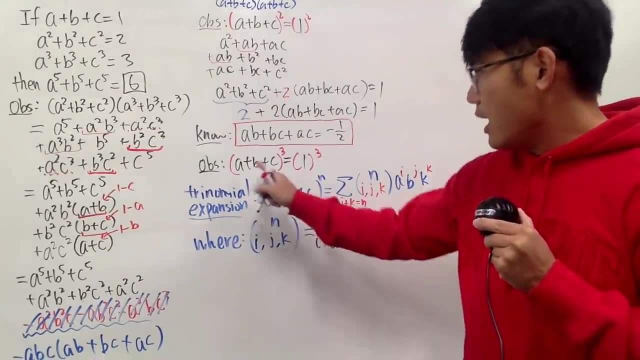 I think I have to write it down here. I will say I actually no, I don't know. Let's see what we can do here. okay, So perhaps I'll just continue working here. In our case, of course, N is three. 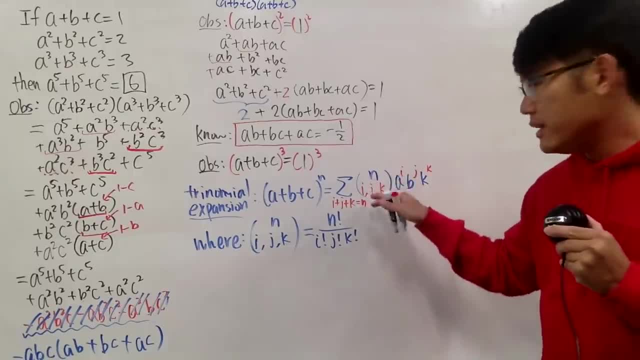 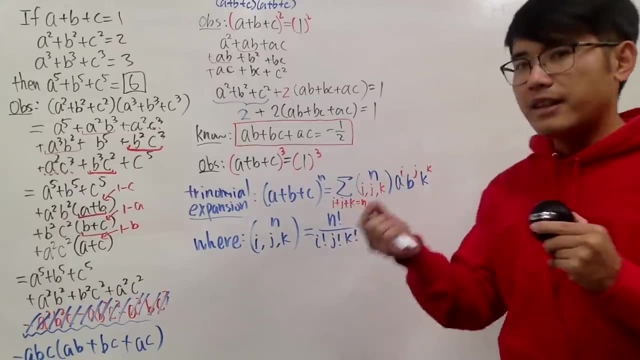 And the sum is you have to just vary the IJK and you have to make sure that all this IJK add up to be N. And perhaps the best way is you're just going to fix a number and keep it to be a number and then just kind of vary this. okay, 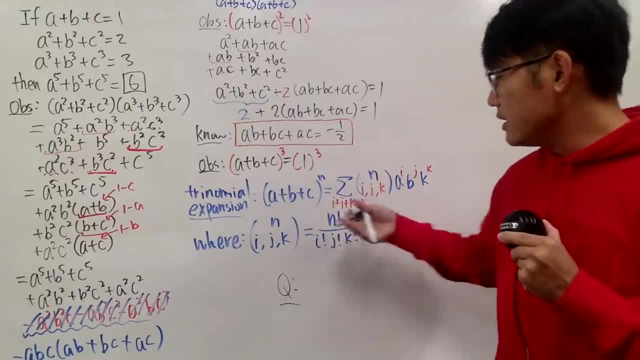 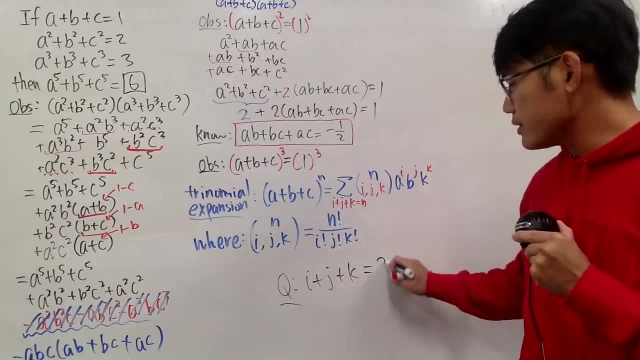 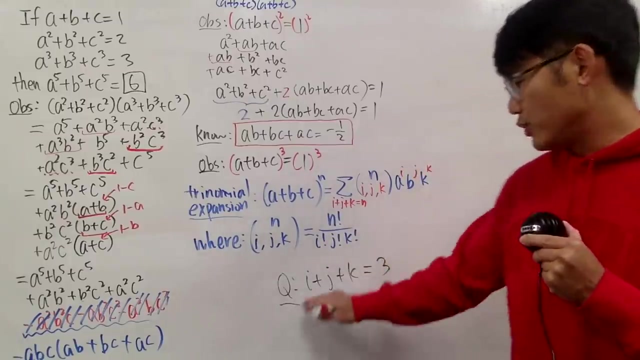 Another really interesting question is: okay, our case is N equals three And I have to look for I plus J plus K equals three. How many solutions do we have for this right here, Non-negative integer solutions to this equation? IJK. 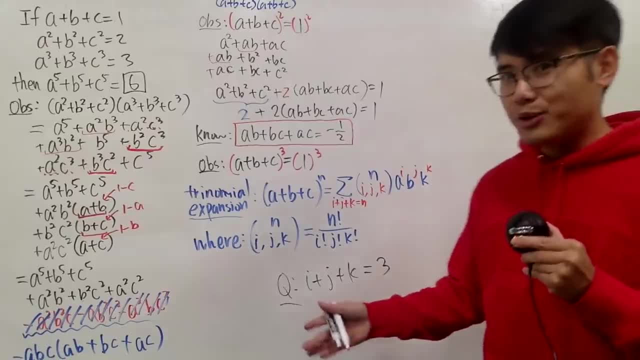 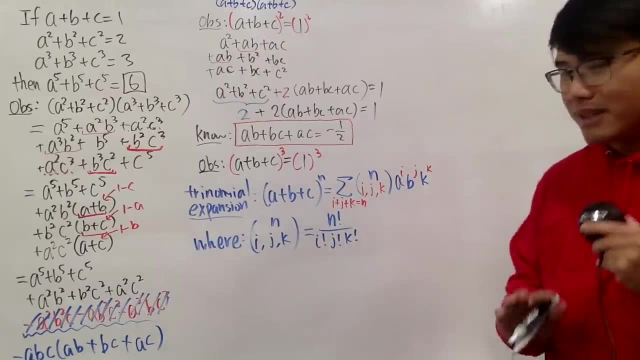 Okay, so this is also a very interesting question. You can kind of just count which. we are going to do that because this question is for the next video. For the future video, you can talk about it by using the generating function. but, as I said, 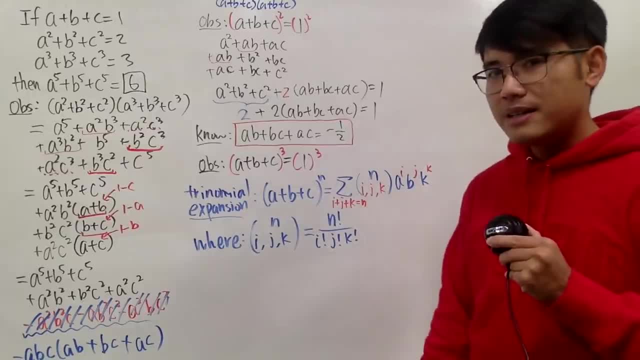 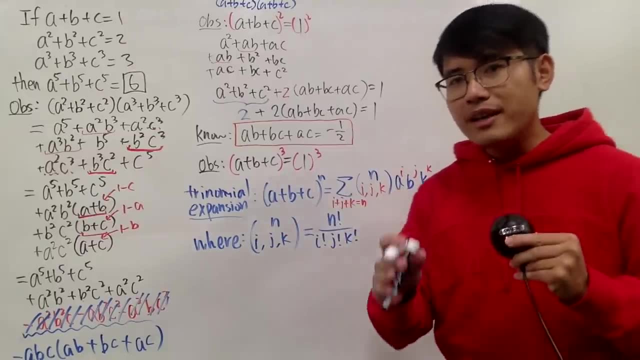 that's for later on. Now here's the deal. I will just keep the K to be zero first, and I will write down the coefficients for you guys. And this is how you get the Pascal's Pyramid entry right. So this is how you can do it. 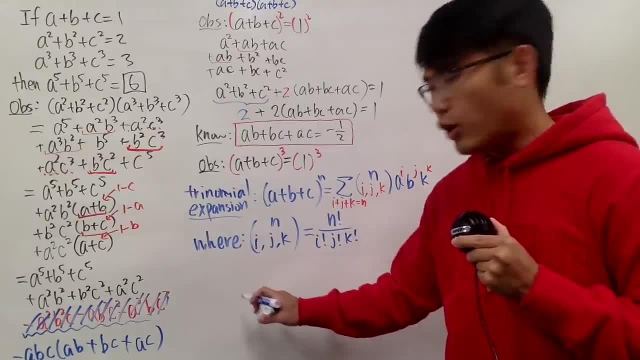 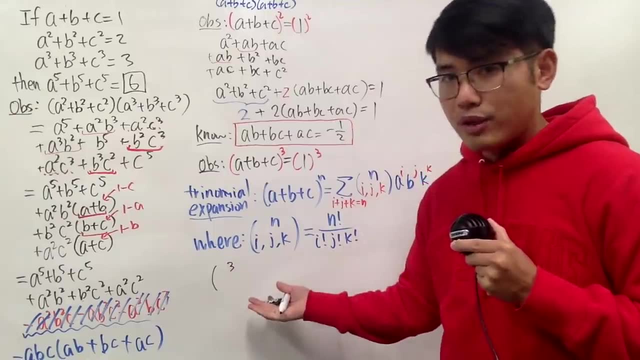 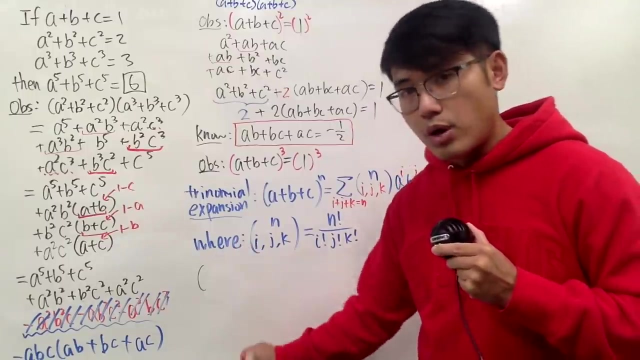 Let me write it down here. I hope we have enough space, right? So the first one is that I will have the N being three, of course, And, as I said, I want the first row to be where K equals zero. so we have three and you have zero here. 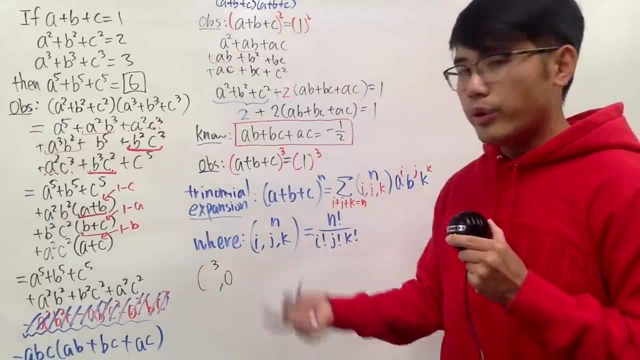 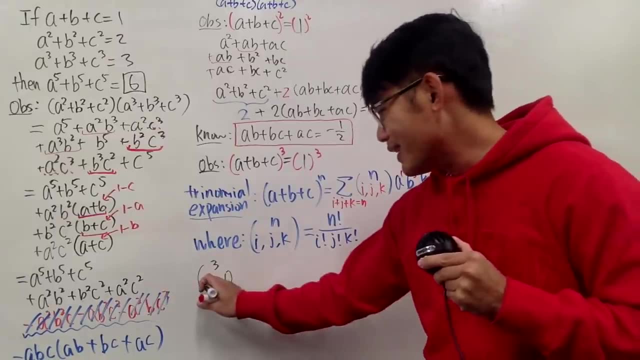 And now you have just I and J. You have to think about what plus what is equal to three, right Plus zero is going to be zero, I mean to be three, So you can do it as three times no, three, zero, zero, right. 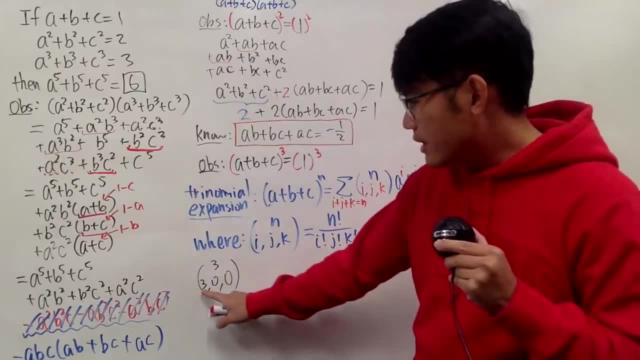 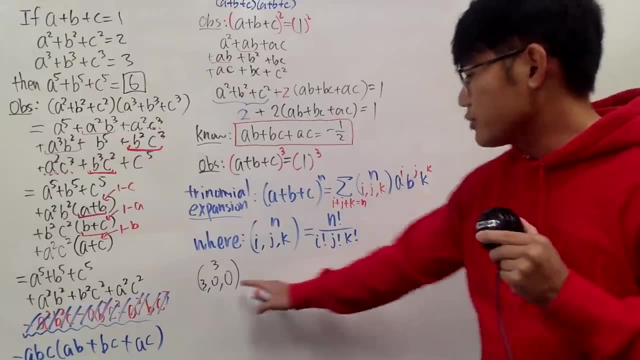 This is the first one, And when you put this down again, this right here tells you the power for the A, and this right here tells you the power for the B, and this right here tells you the power for the No. I still put it down wrong. 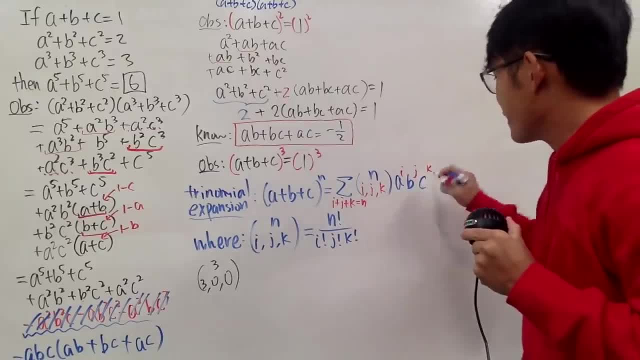 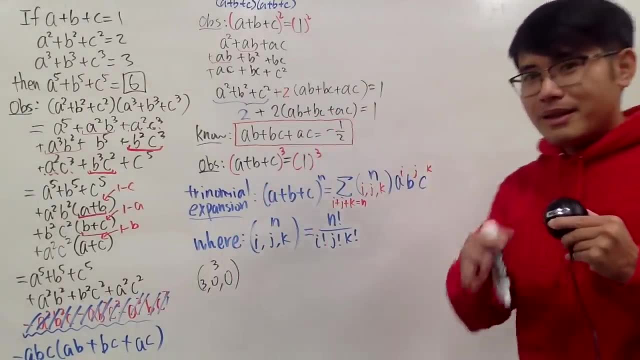 Sorry, I did fix it okay. So if you comment it, let me just tell you I'm in number, I'm in a minute twenty. okay, I did fix it. Anyway, this right here tells you the powers, right. 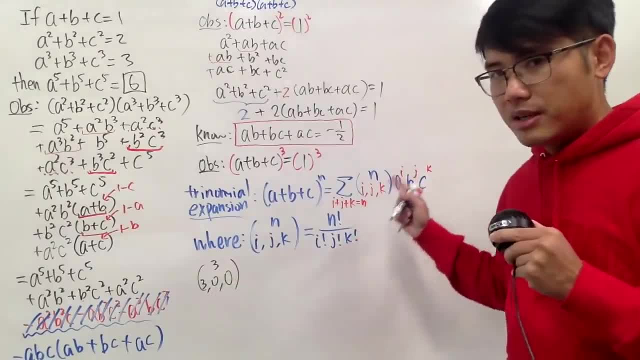 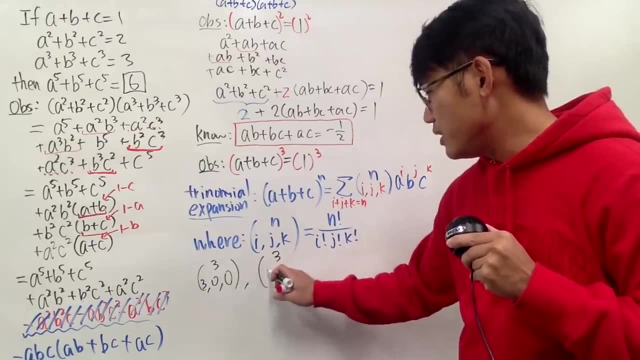 Okay, And I'm not going to write it down Seriously, just kind of keep that in mind. So this is the first entry and the next entry is going to be three, and then again I will keep this zero, so perhaps I can. 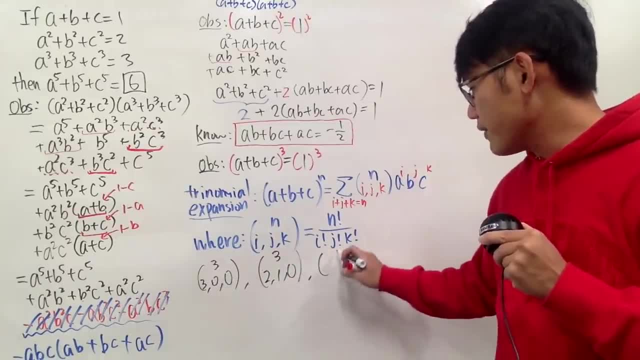 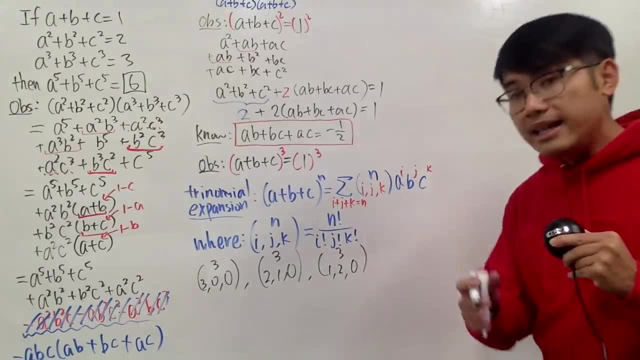 make this two, one right, And then next I can have three and then zero, and then maybe I will do one, two, Like that. so that's pretty good, And I can also do three and then zero. 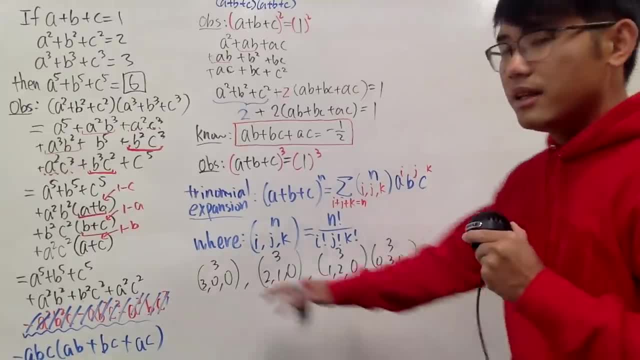 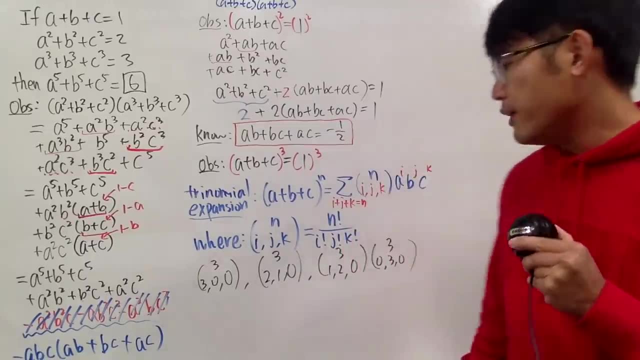 three zero, isn't it? Yes, it is, of course. That's the first row where the k is zero. Now the next row is, of course, where the k is equal to one and you actually will have one less entry. 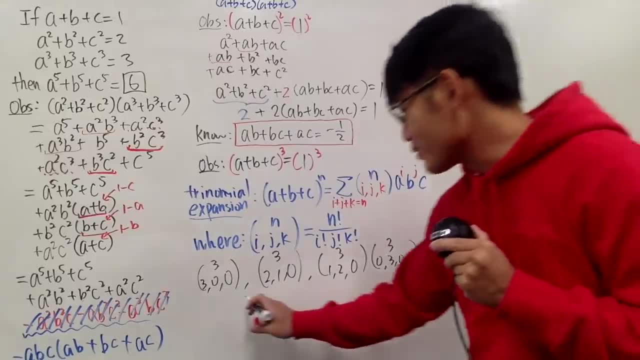 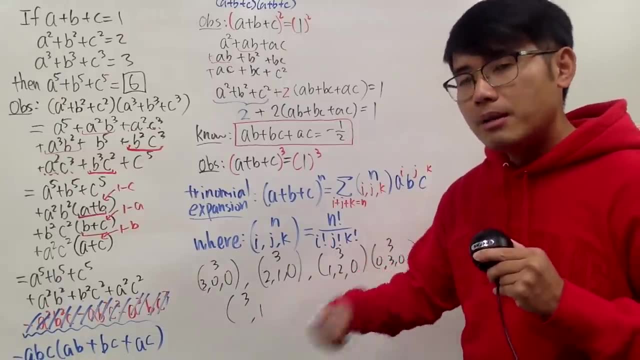 because right here you have four, Now the next one you have three. It's really similar to the Pascal Triangle, But anyway, three k is one. and think about it. how can you do it? You can put down one, one, one. 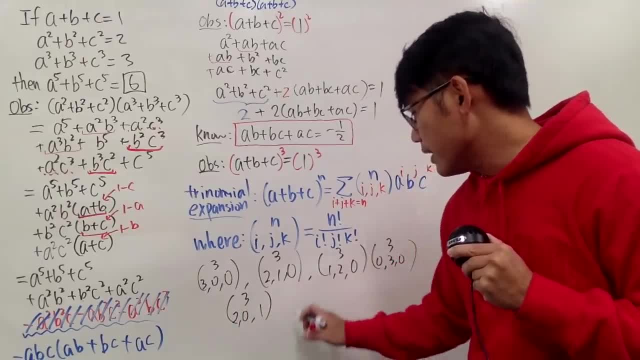 but let's keep it in your next order. I will start with the bigger number, two and then two zero one right, And then the next one. I will just put down: okay, three and then one, one one. 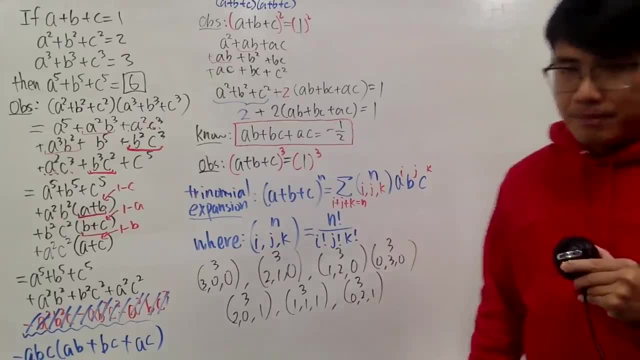 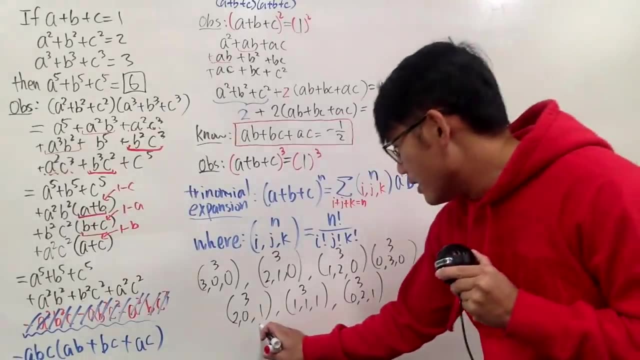 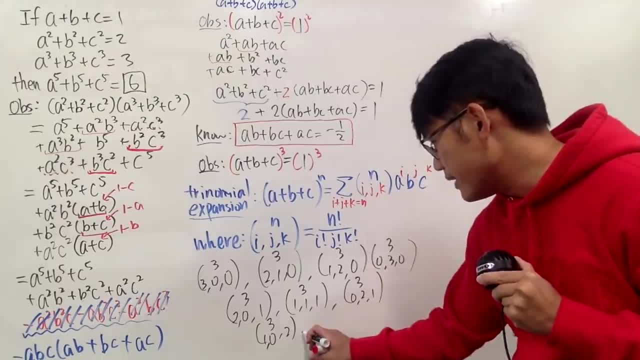 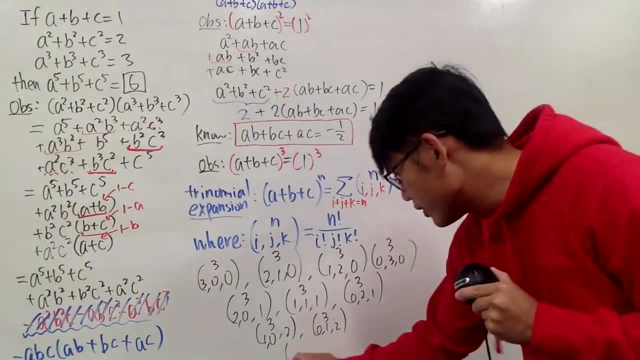 So I may have one zero, two, right, And then the next one is three, zero one, two like that, And the last one is just three, and then the k is three and then zero, zero, like this: 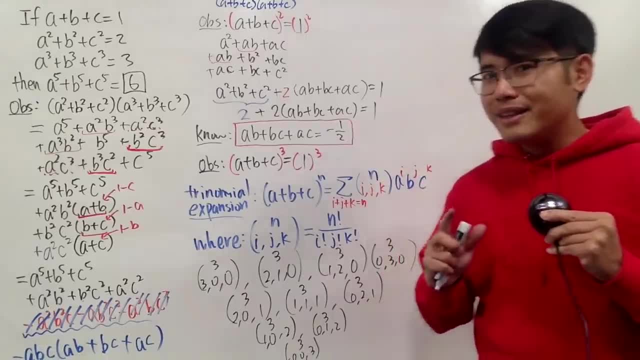 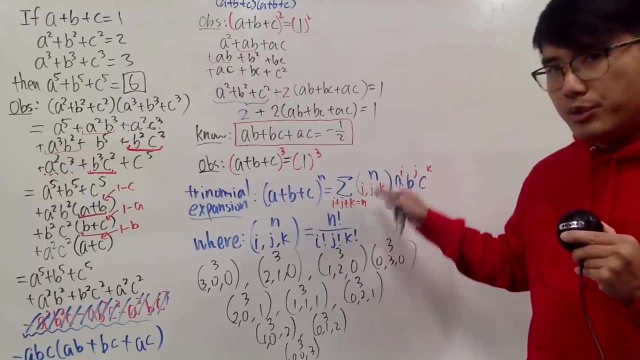 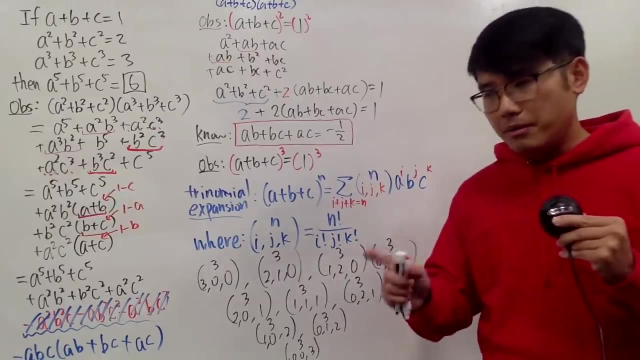 So you have a total of ten terms. Yes, earlier. the question is, if you have i plus j plus k equals three. in fact you have ten ways to make that happen. Suppose you have, suppose the order matters, and also non-negative. 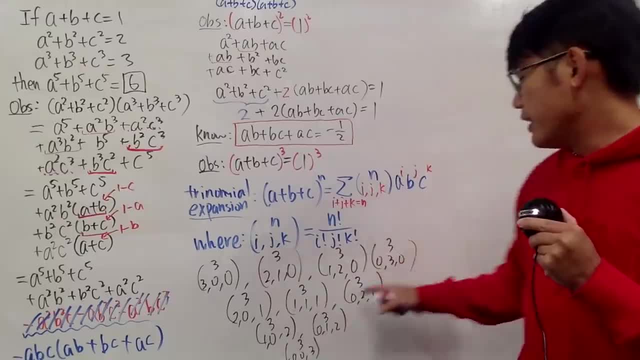 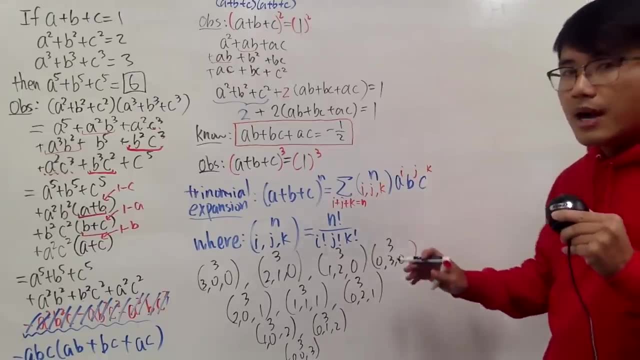 integers right. So three zero zero is different than zero zero three right. That would be considered different solutions. Okay, so now I will write this down: We're not doing integrals, but I know this is just like. 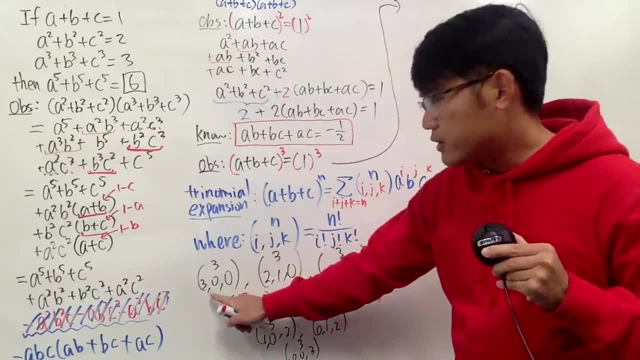 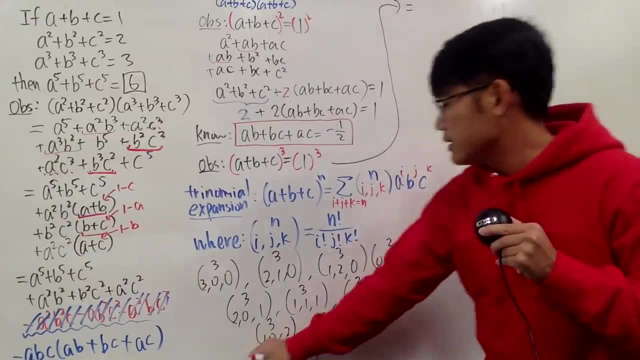 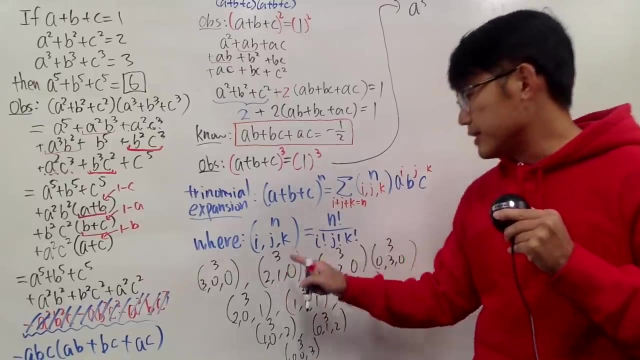 a new cosine: When we expand this right here, first you will have this guy as a to the third power and let's see we get a to the third power here. right, And this right here. okay, let's do this in your head. 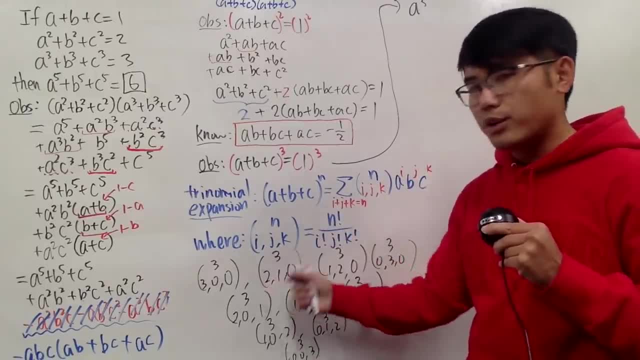 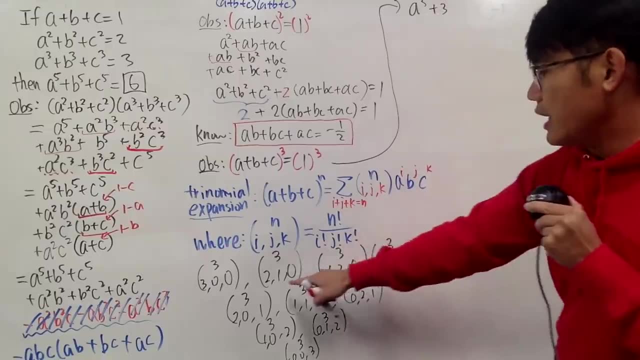 Three divided, three factorial, which is six, divided by two factorial, one factorial, you get three. In fact, this is three, this is also three. So you have plus three, a squared b squared. I mean a squared b to the first power. 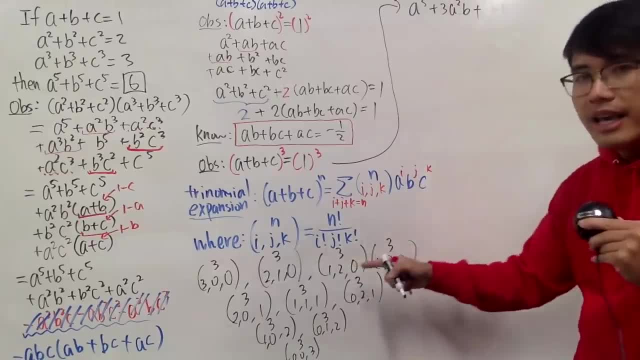 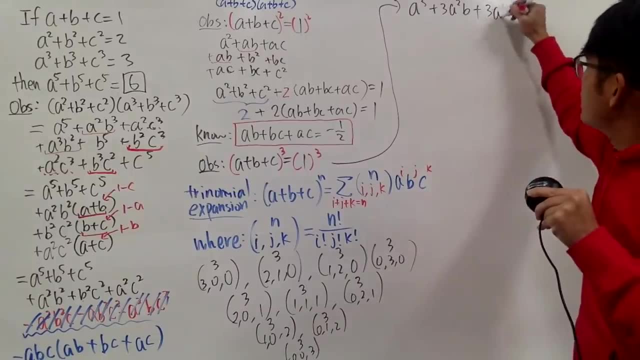 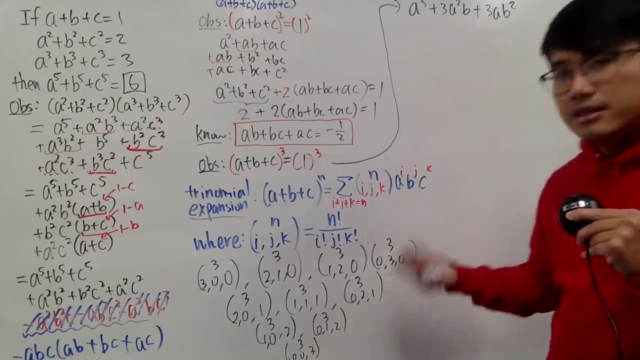 Right Plus, and this right here again, three factorial divided by one factorial, two factorial. in the denominator you get three, and then this is a to the first power and b to the second power. This right here corresponds to b to the third power. 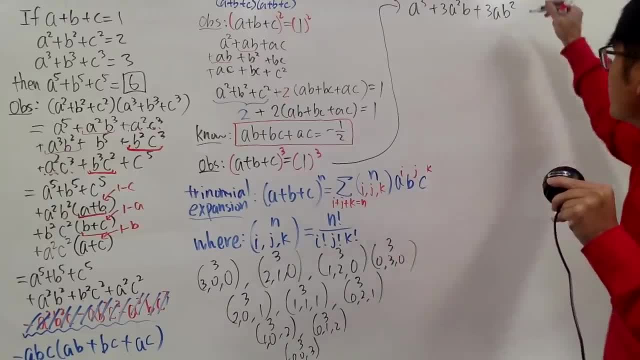 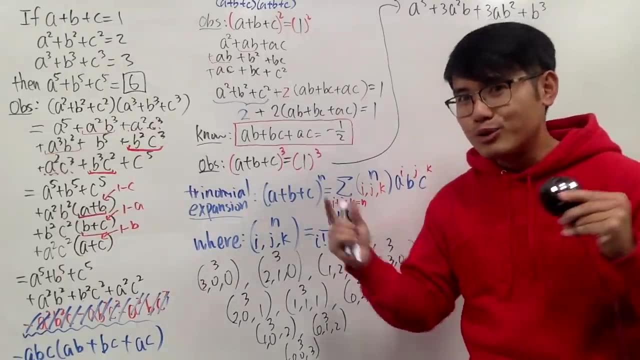 and three factorial. divided by three factorial, you get one. So I will just put this down right here. and then we plus b to the third power. And this right here should remind you guys about the usual binomial expansion: a plus b. 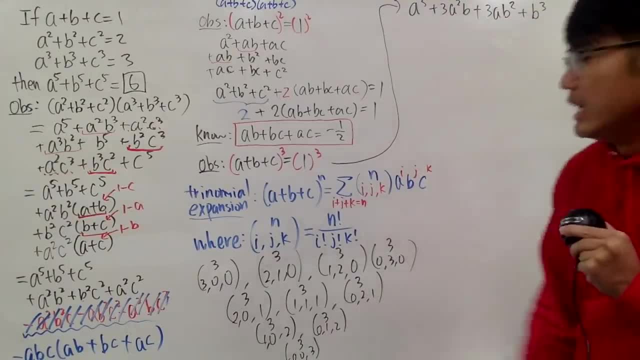 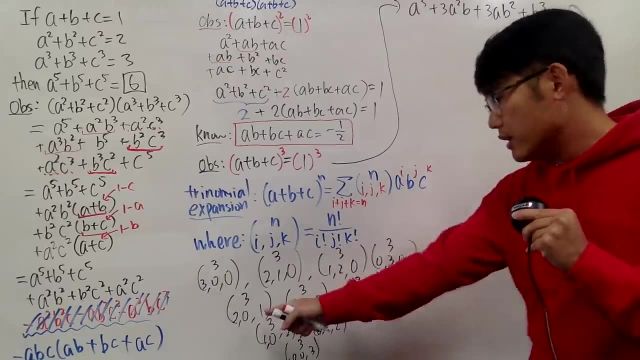 to the third power. Really cool, huh. Now c is coming in right, So we have the c term, because k is one. now, So right here again: three factorial divided by two factorial and one factorial is three, so we will. 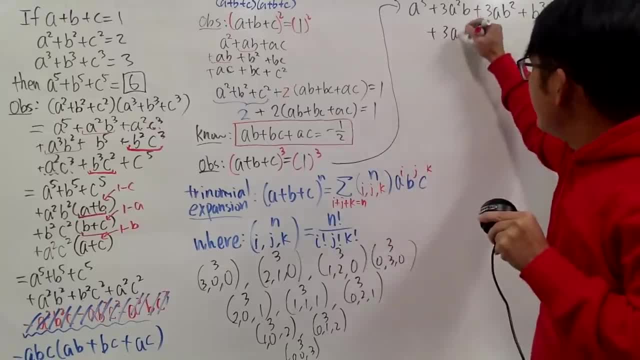 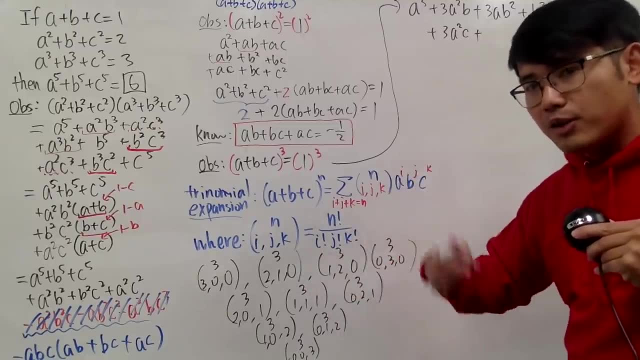 have to add the three here, and then this is a squared, and c to the first power, and we add this right here is cool because it's three divided by one factorial, one factorial, one factorial which is going to be six. So we have six. 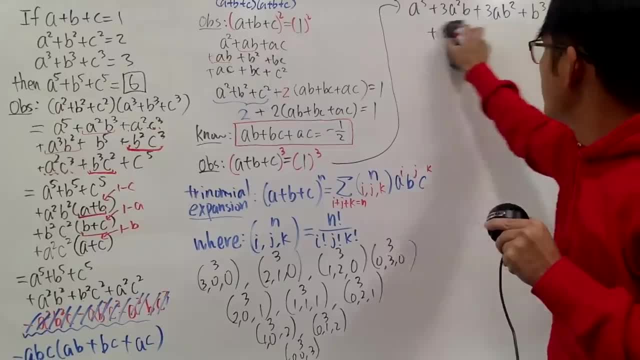 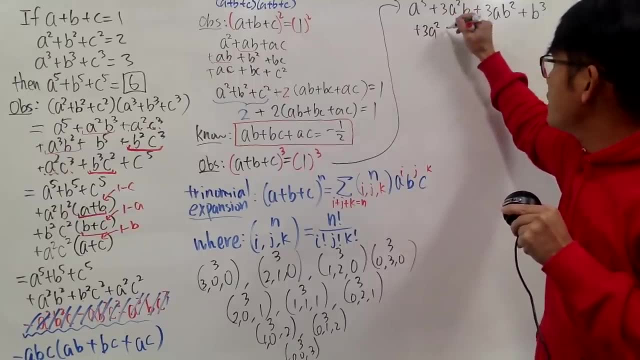 And then we have to have a, b, c, And in fact let me write it down better right here: So this is plus three a squared c to the first power earlier, and then this one gives us six: a, b, c and the next 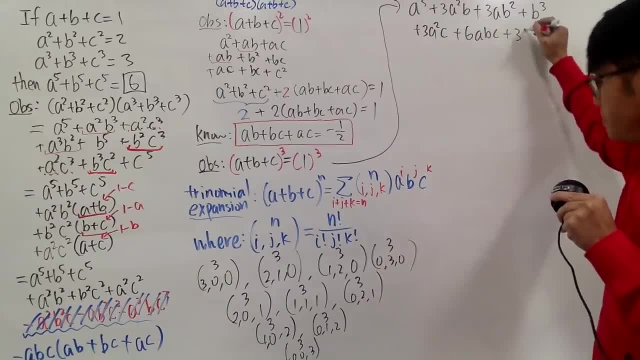 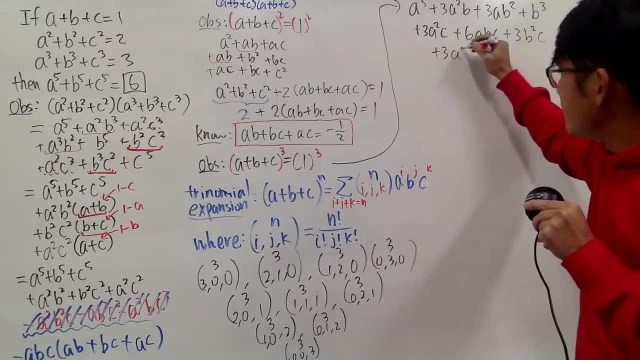 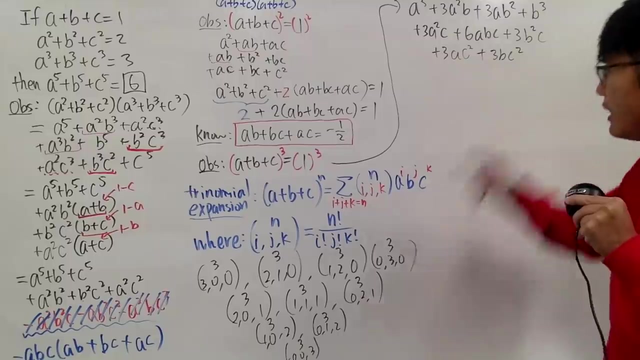 one: this right here gives us three b squared c. alright. And then we continue. This right here will correspond to plus three a c squared. plus this right here will correspond to what Three b c squared, and lastly, oh my goodness, plus. 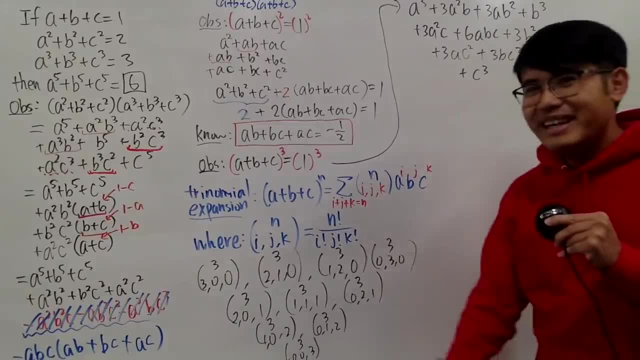 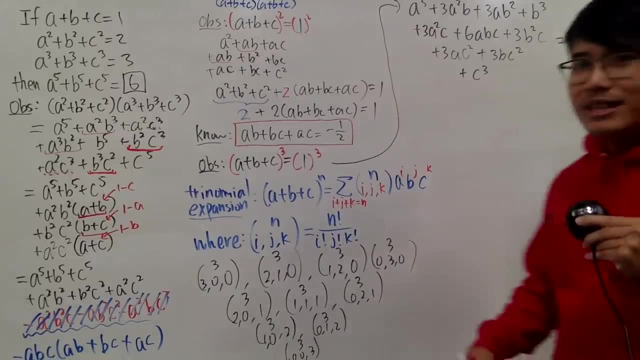 c to the third power. All that, So all this stuff, they will add up to one, believe it or not. So all this is equal to one. And, of course, now this is the time for us to do some factoring and all that stuff, So as we can. 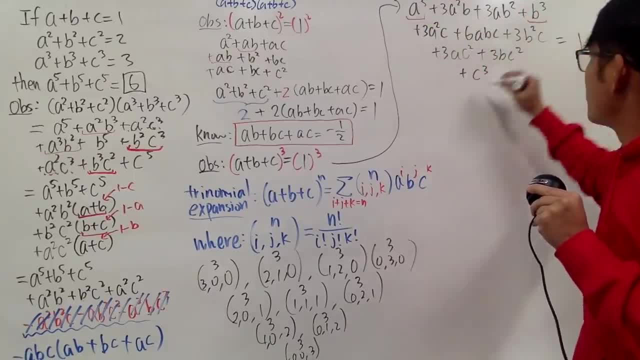 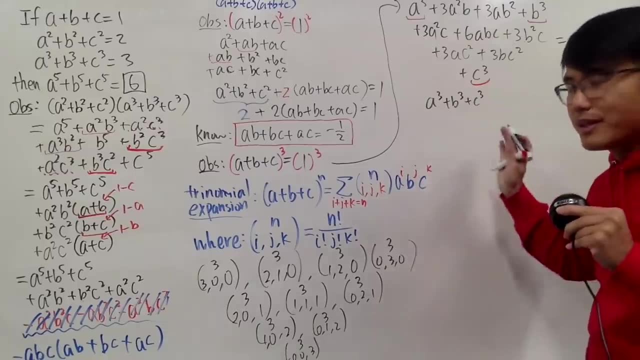 see we have the a to the third power, b to the third power and c to the third power. so we know, a to the third power plus b to the third power, plus c to the third power is no, not yet. we have a lot more to go, of course. 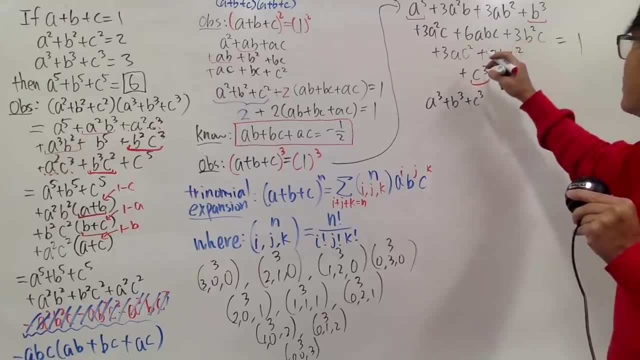 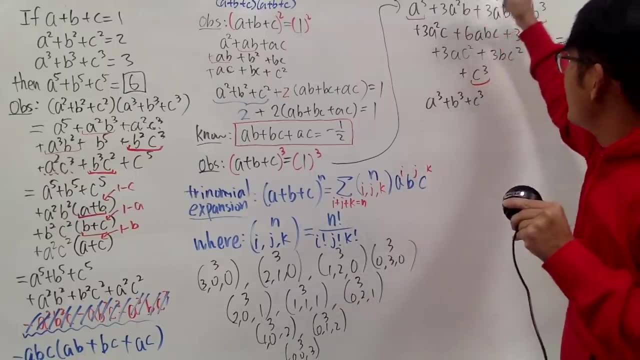 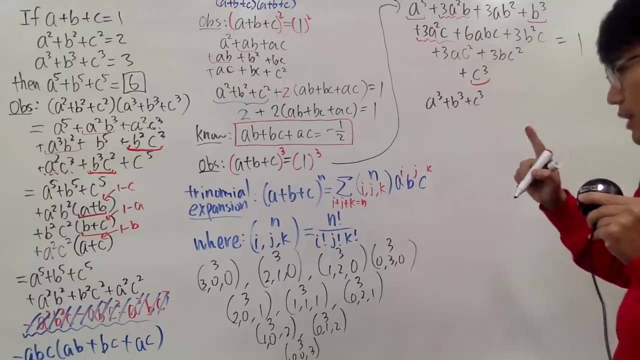 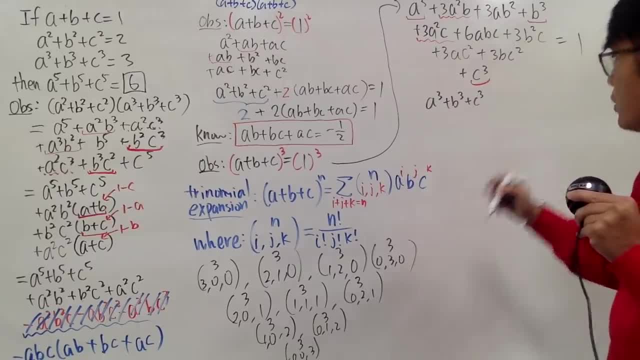 somewhere we should have another problem with a squared. Actually, we don't have another a squared, so I will just factor the a squared right here. so we have, plus let's factor out the three. Let's see. check this out. 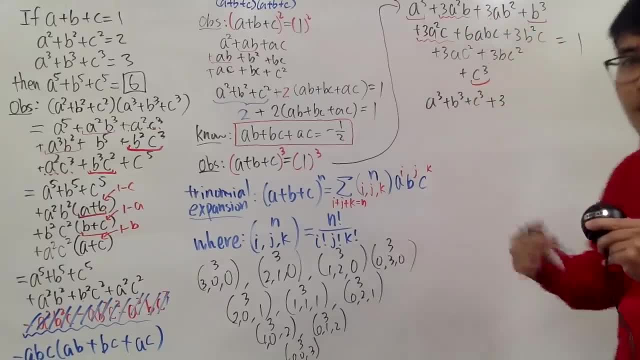 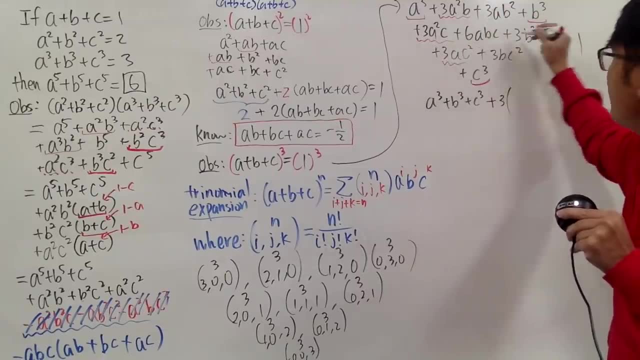 Three, three, three, three, three, three. They all have three. so I will actually factor out three for a lot of things, alright, So this guys right here, they all have three. so that's very, very nice. 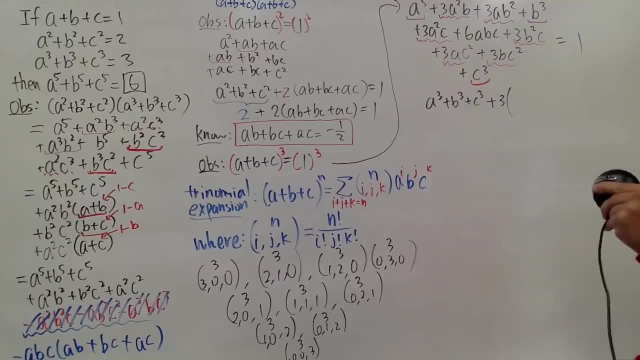 Alright, And sigh, sigh, sigh. If I factor out a squared right here, I will get a squared and then b plus c. yeah, So I'll just do that right here. I don't know what's happening, but like I'll see what. 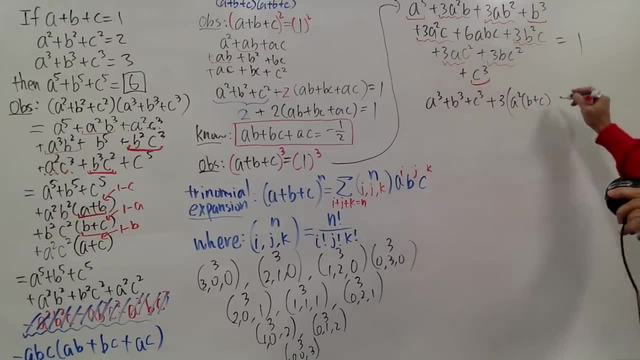 will happen. And then this: right here I can factor out the b squared, so I'll put down plus b squared, and then this will give us a plus c. Okay, And uh, this too, huh, So I can factor out the c squared. 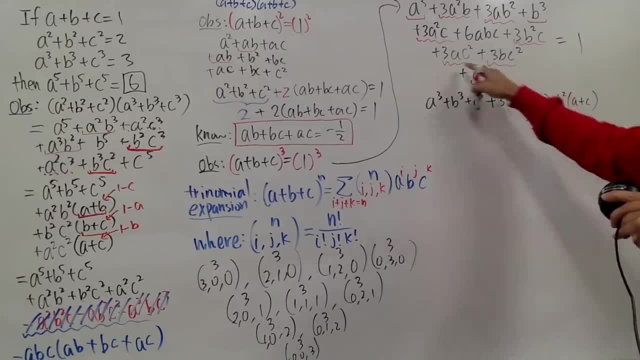 so I'll put this down right here: plus c, squared, and I will get a plus b. That is kind of nice, and this is still equal to one Sigh. Yeah, let's see what happens. It's really interesting actually. 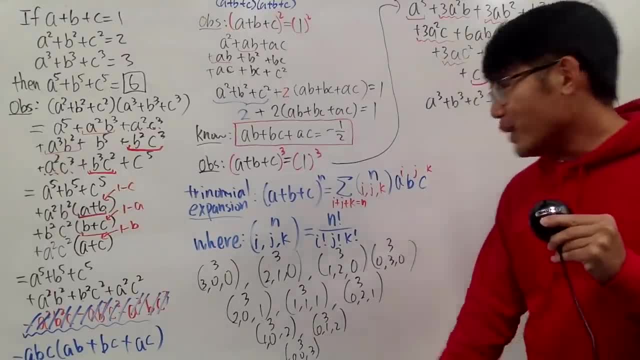 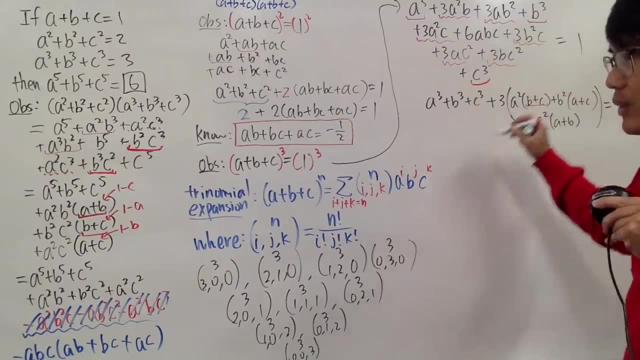 And oh my god, I think we have to do this trick again. huh, Because we noticed that we have the b plus c, which is the same as one minus c, because we can use the original equation over there. So this right. 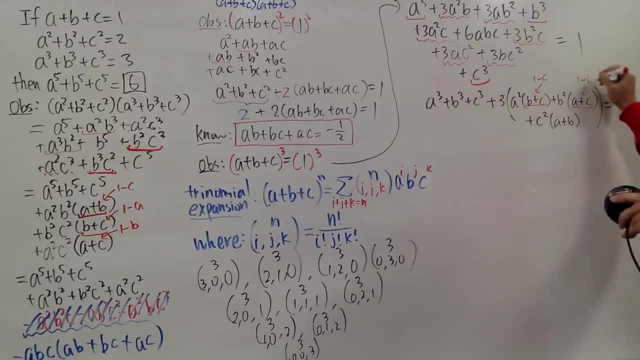 here is one minus c, this right here will be one minus b and this right here is one minus c. Sorry, this right here should be one minus a, because I will have to minus the a on both sides. Yeah, So this is one minus c. 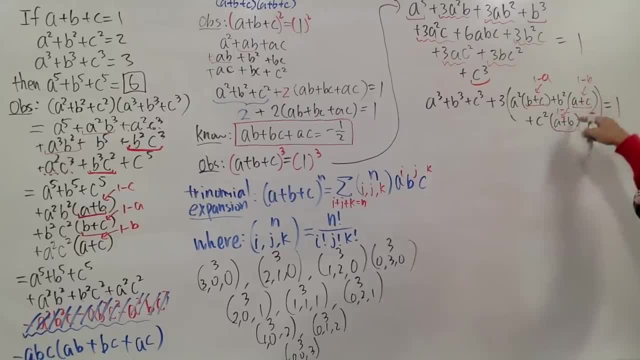 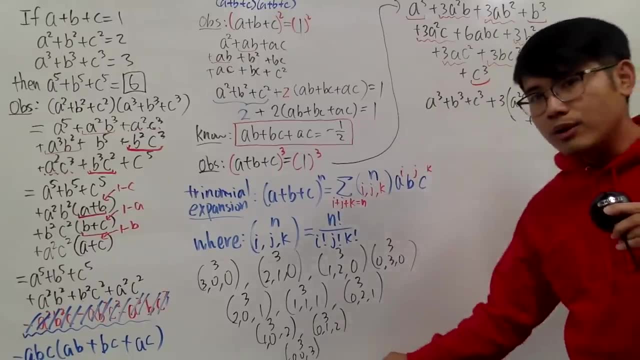 one minus c right here and all that stuff. Okay, so distribute this, guys. oh god man, But we do know this part is equal to three, So I just put down three right here for you guys. So 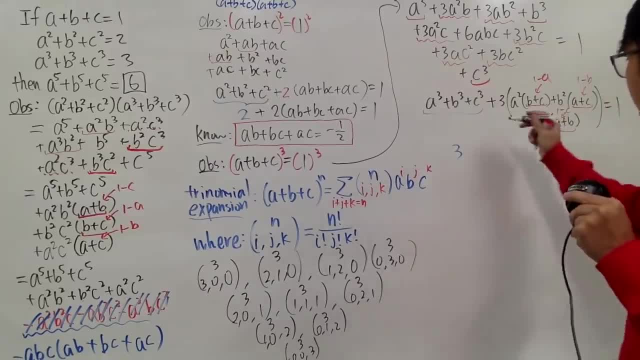 this right here is three, So that's taken care of already, And right here we have to add: we have another three right here and let's see a squared times. all that, okay, we have the a squared. 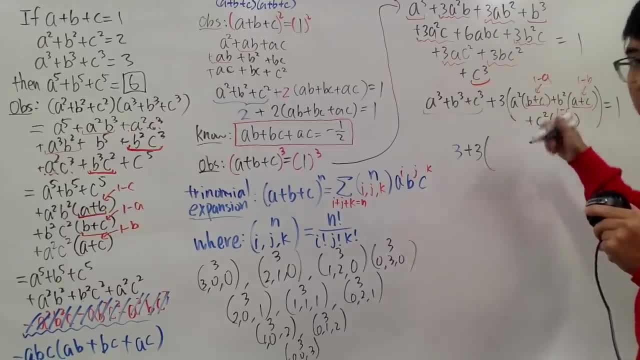 So we have the- let's do the first part- in black. We have the a squared right here, right a squared and then b squared, plus b squared, and then the c squared, of course, plus c squared. Hey, we got the a, b, c. 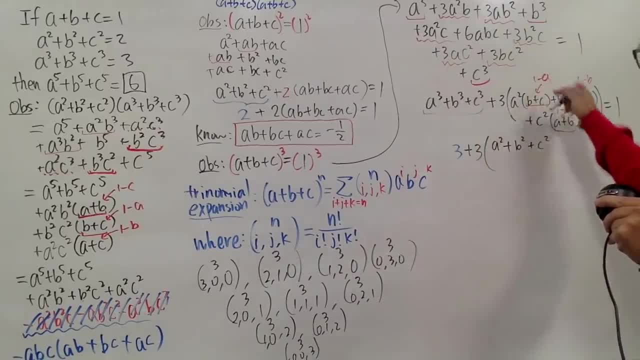 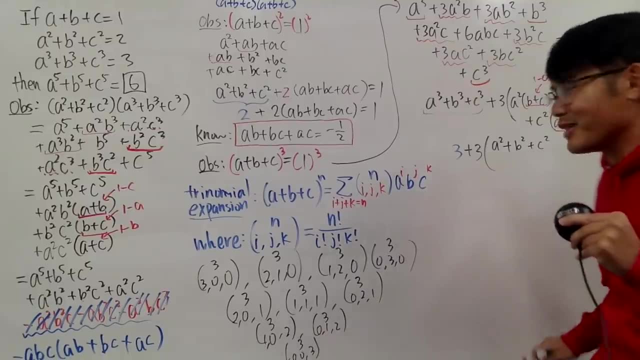 somewhere, right? No, this is still the where's the a b c, though. Oh yeah, I was still. oh, I forgot to write down a b c. I forgot to write down six a b c. sorry, And let me just put that. 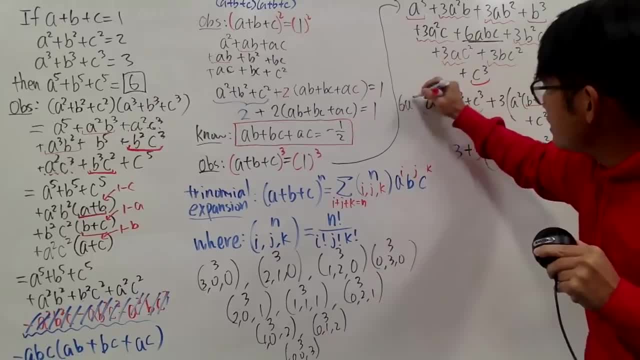 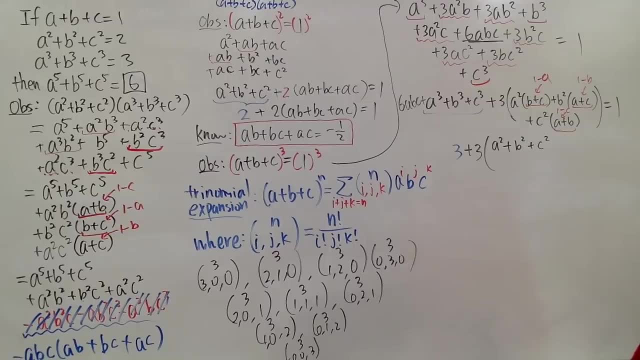 in the all the way in the front, This right here, it's plus six a, b, c, Right, so all that, Yeah, cool, okay, So all that, and then you have to have the minus and that's the a cubed. 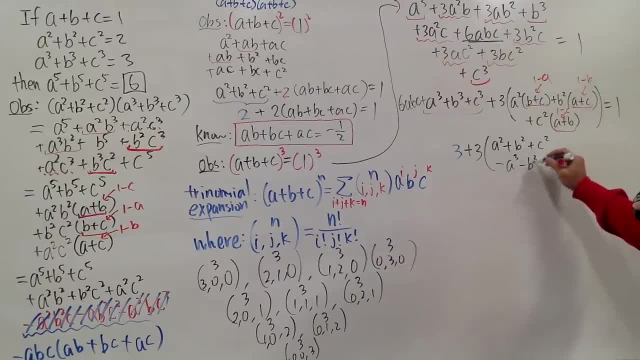 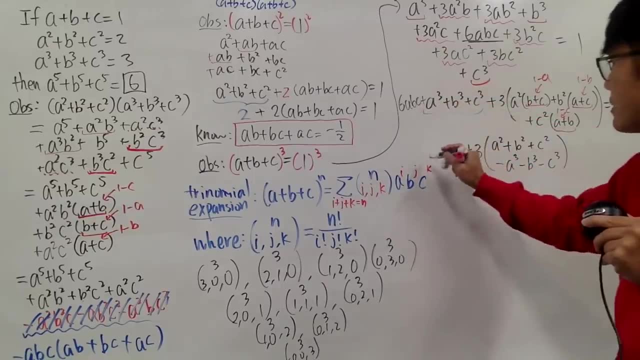 and then you have to minus the b cubed and then you have to minus the c cubed. Cool Like this. And earlier I forgot the six plus. let's close this guy. We have to put down the six a, b, c plus. 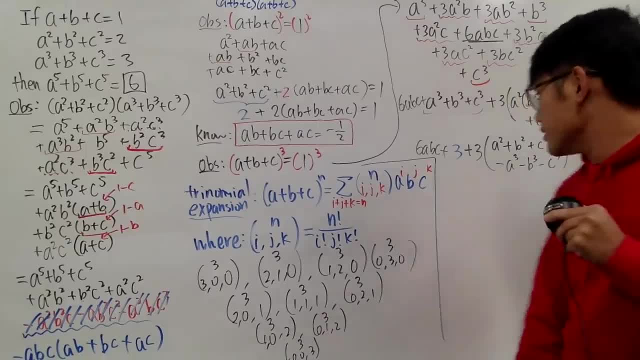 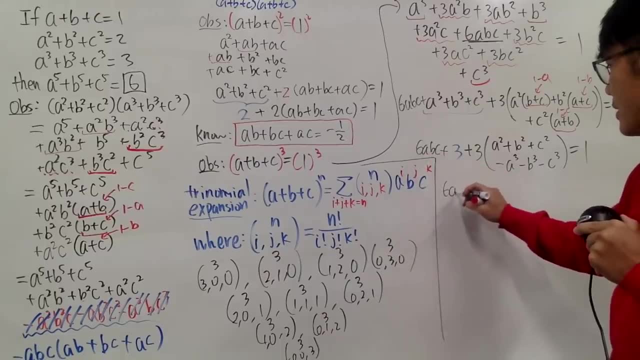 all that right, So this is still equal to one. So now let's see. Okay, So I will keep the six right here, and with the a, b, c, of course, I will minus three on both sides. so keep that in mind. 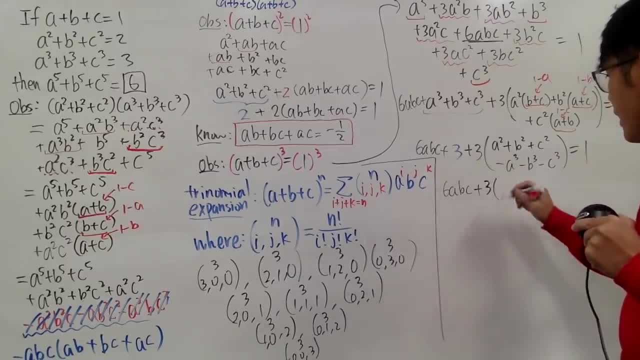 minus three on both sides. okay, So I will put down this three and let me just indicate that: Minus three on both sides. so this is out: a plus a squared, plus b squared, plus c squared, this is equal to two. Finally, we 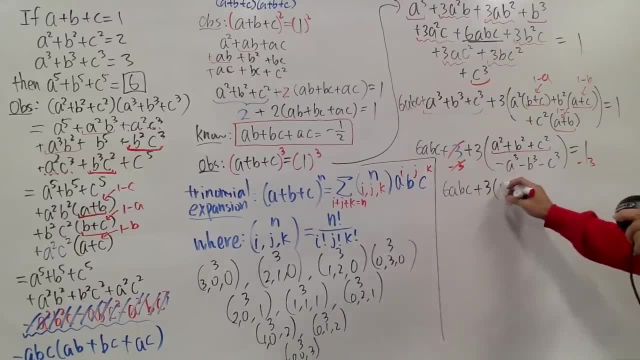 use the two. Huh, Oh, actually we use the over there, not in that setting, sorry. And then minus this, and of course we can factor out the negative. and then all this part right here, the cubes is the three, so we can. 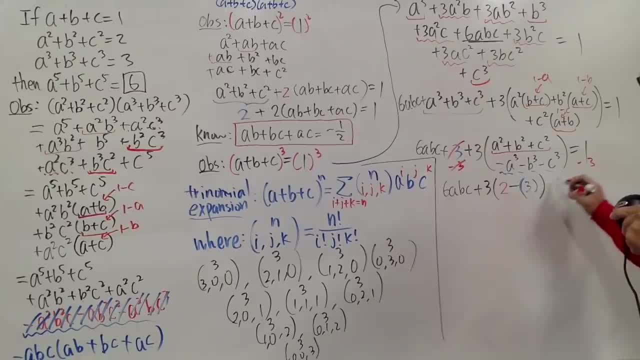 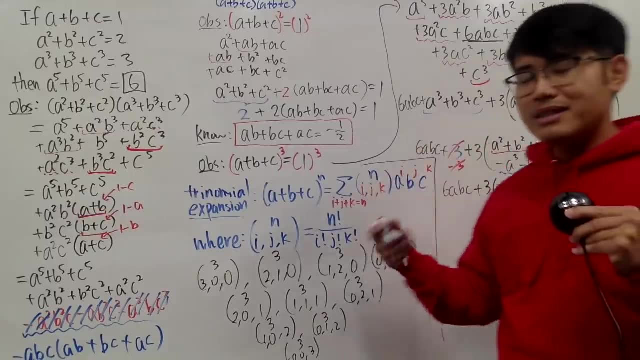 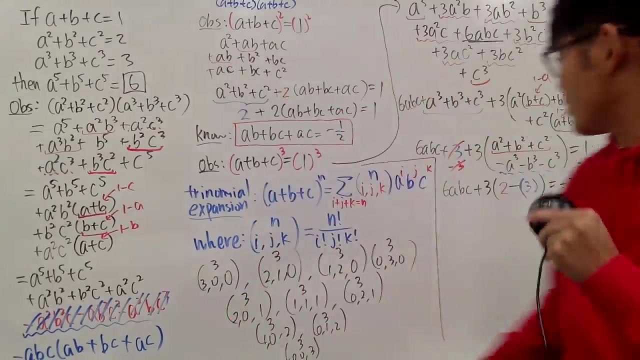 minus the three right here, and this right here is equal to negative two. Sometimes, in fact, if you remember the formulas, the identities, you can actually just write it down all that. but again, this is extreme algebra, extreme algebra. 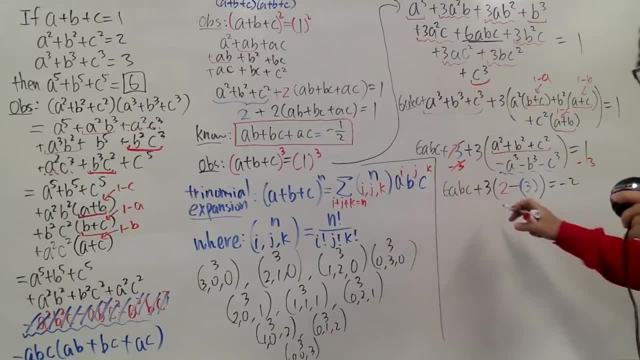 question. all that, Let's see, And here we have the six a, b, c. Let's do this in our head: Two minus three is negative one, so here is negative three. So six a, b, c minus three. 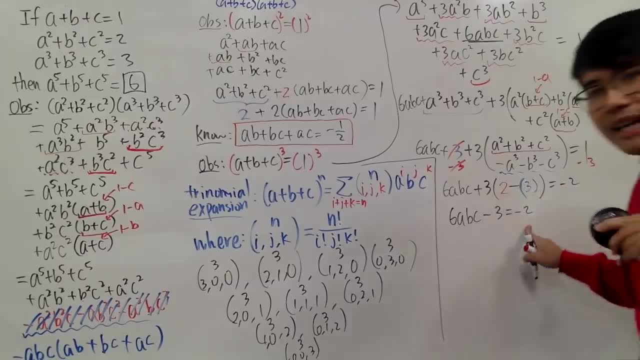 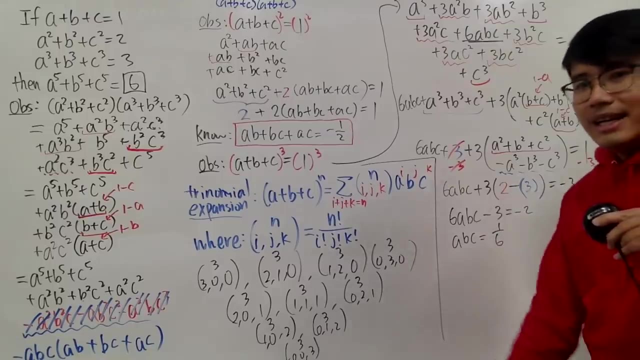 is equal to negative two. So we add a three on both sides, so that will be positive one and divide six on both sides. So a b, c is equal to one over six, Like that. Okay, so now we know this much better. So a b, c is equal. 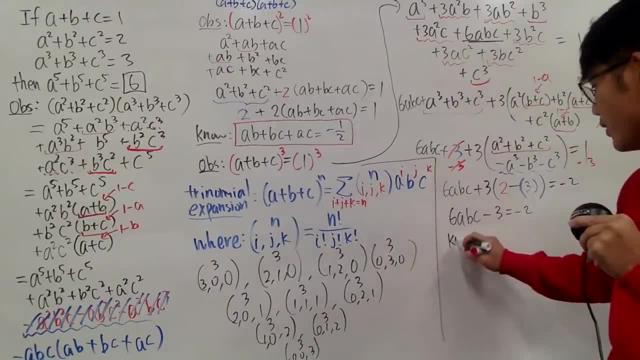 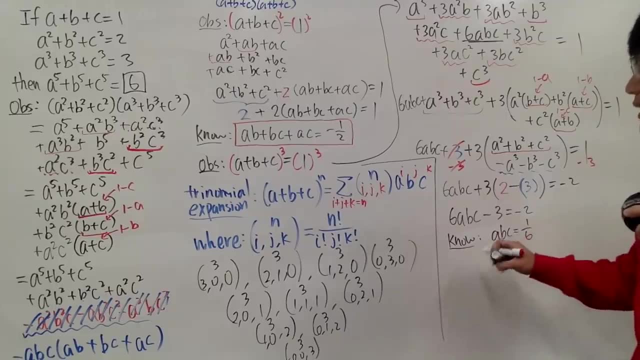 to one over six. In fact, this is a really famous, well-known question, Right, Really famous, really well-known question. a, b, c is equal to one over six, But we are all adults now. We are all adults now, so we are going to do the. 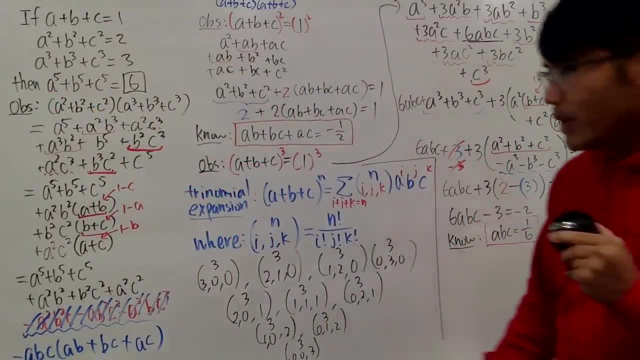 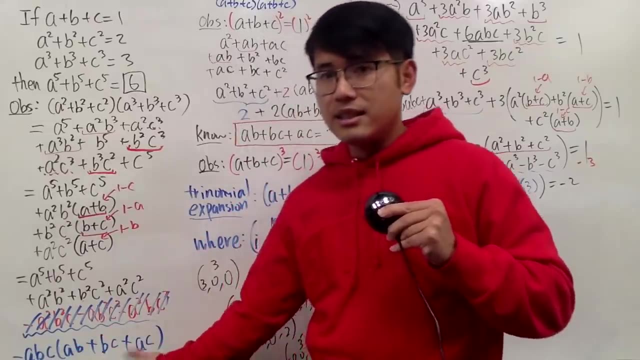 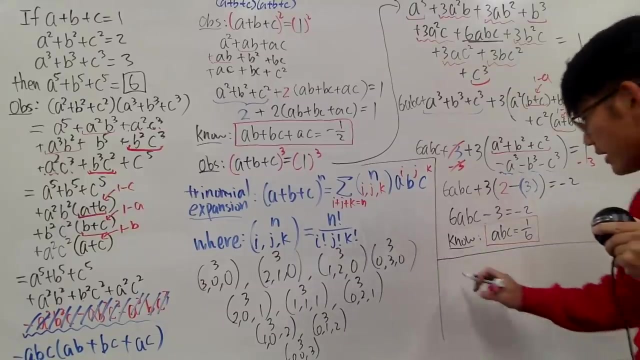 fifth power. Okay, Well, well, well, a to the fifth power. all that minus a, b, c times. this is equal to this times that. So in the end, we just have to do the following: Okay, So let's do this in our head. 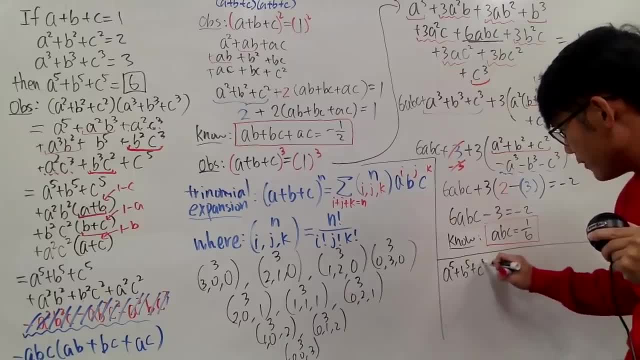 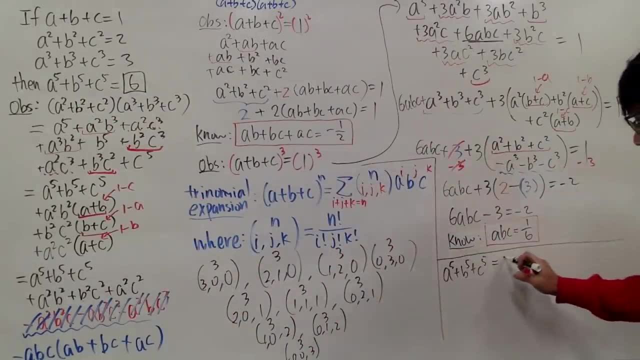 a fifth power, plus b to the fifth power, plus c to the fifth power. This right here you have an identity. You can just move this to the other side. That's not identity. We did hard work for that. This right here is equal to: 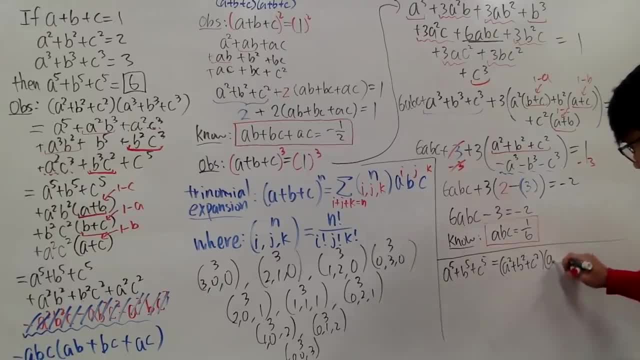 a squared plus b squared plus c, squared times a third power plus b to the third power, plus c to the third power. And you add, let me just put down, we add, let me just write that We add a, b, c times a b plus b c. 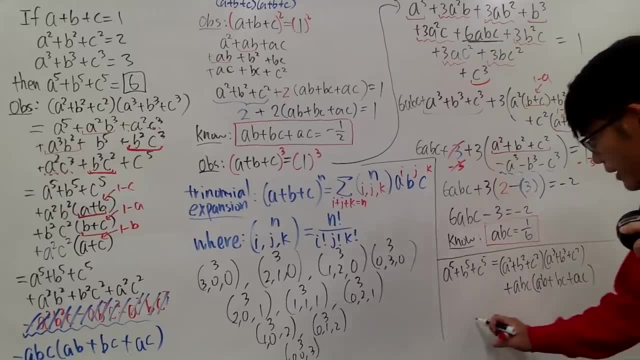 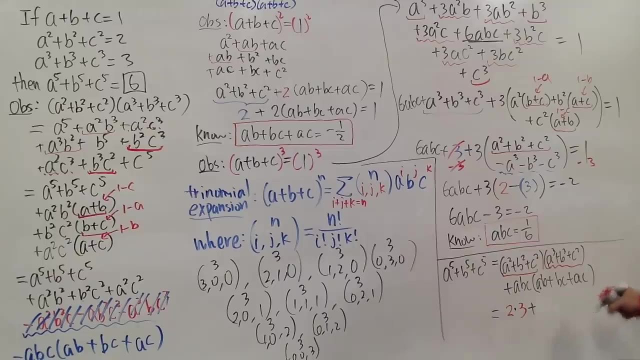 plus a, c, like that. So let's see what do we get? Alright, a squared, plus b squared, plus c squared, this is two, And we multiply by this right, here is three, right, And then plus a, b, c is one over six. So we have: 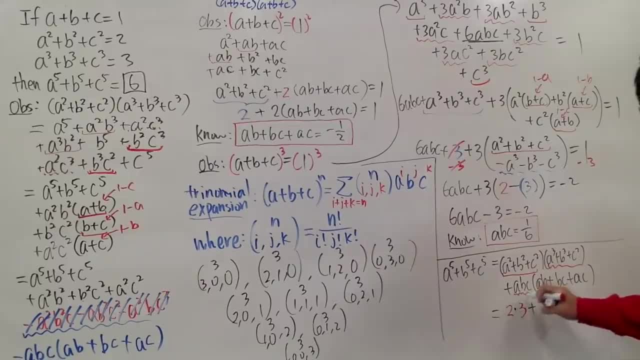 that right here, This is perhaps, oh, just something red One over six, And this part right here is a bunch of dot like this. This right here is equal to negative one half. So we multiply by negative one half, Like that. 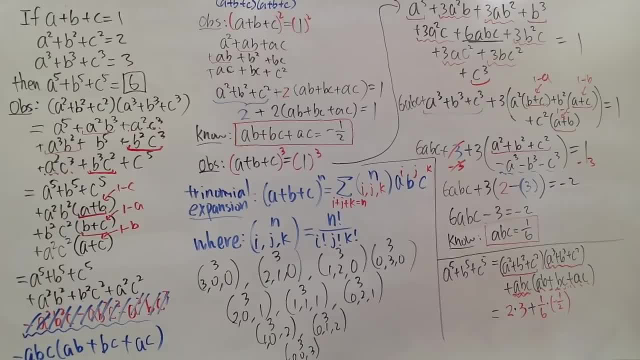 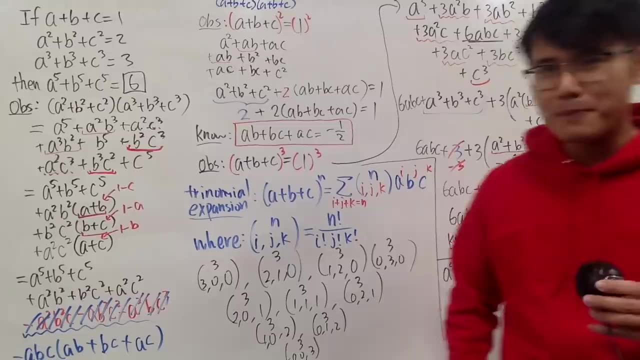 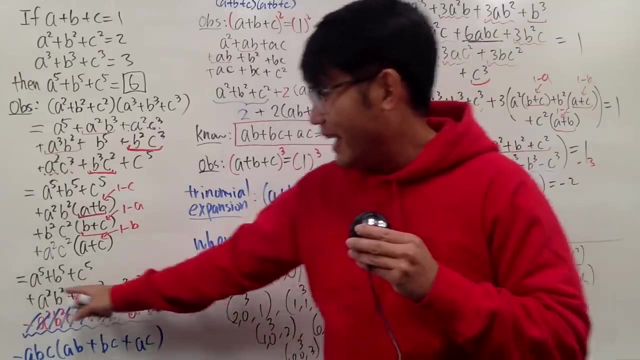 Shit, Something's wrong. Okay, So I'm not going to lie. I pause the video and double check. And I forgot This guy. Sure, a squared plus b squared, all that stuff. So, and to work on that we will have to. 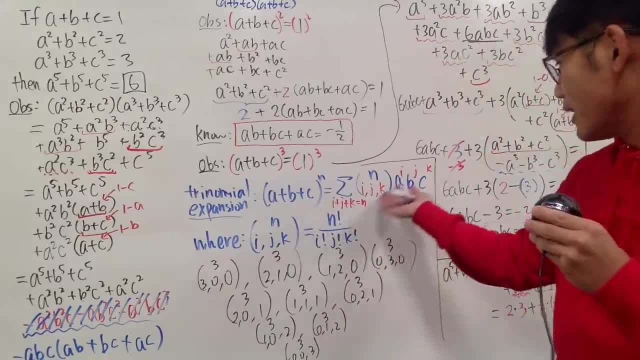 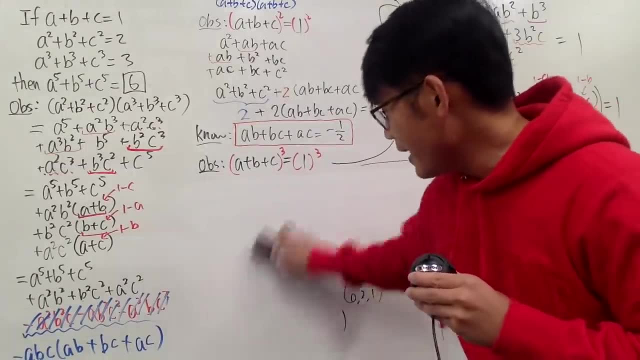 look at this and square both sides, And by now you guys should have enough time to look at this already. So I will erase that And hopefully I can have enough space to fit in everything in here And we'll figure out what that expression is. Okay. 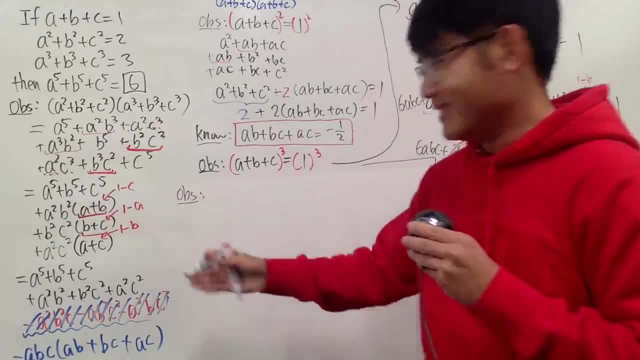 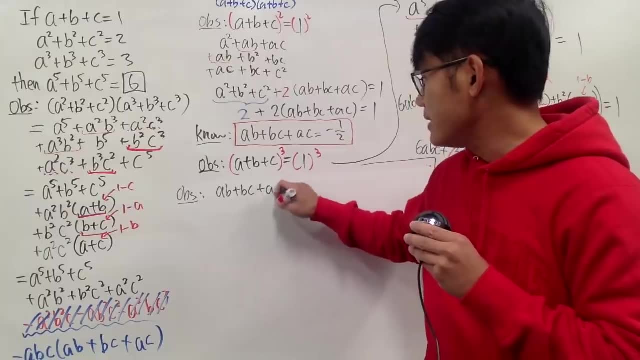 So, again, let's make an observation for this expression, And to do so again, we will have to square both sides. Let's take a b plus b c plus a c equals negative one half, Not negative one over twelve. Okay, And the reason that you take this and square both sides? 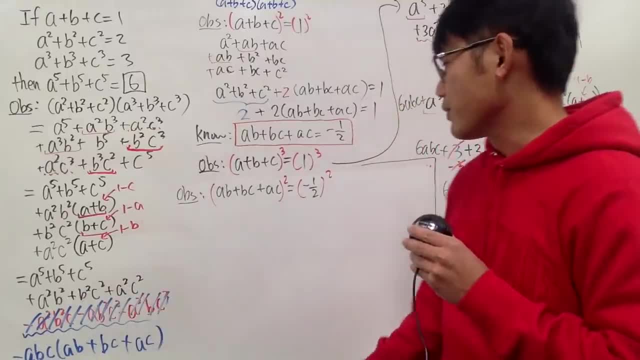 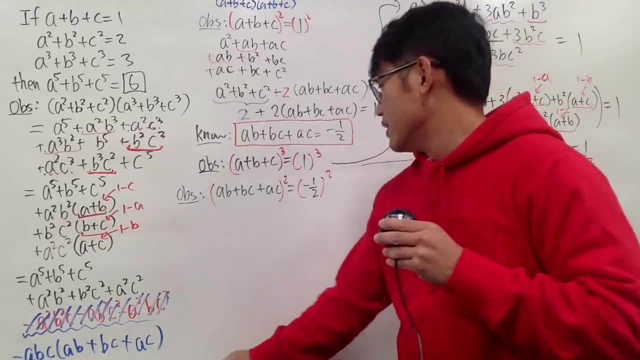 is because that's how you can produce the a squared, b squared and all that stuff, Of course. So we will pretty much do the same thing as what we did earlier, And if you would like, you can just write it down twice Right, And then just kind of. 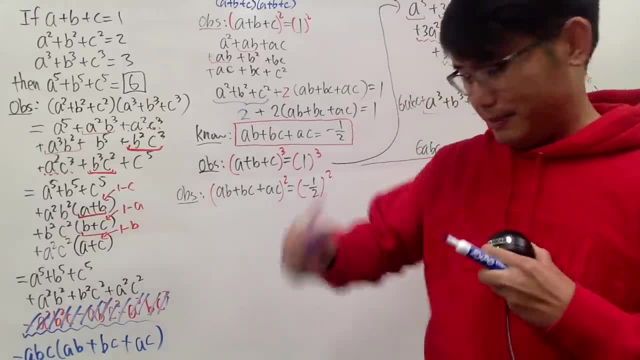 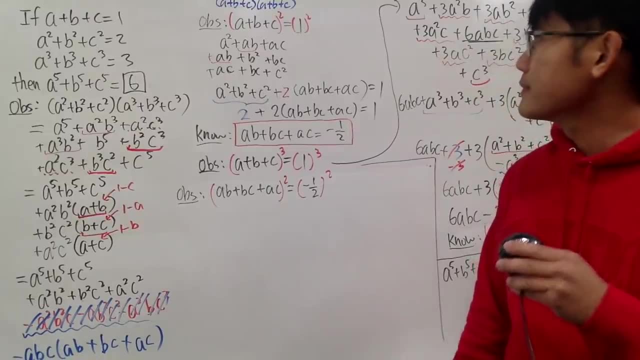 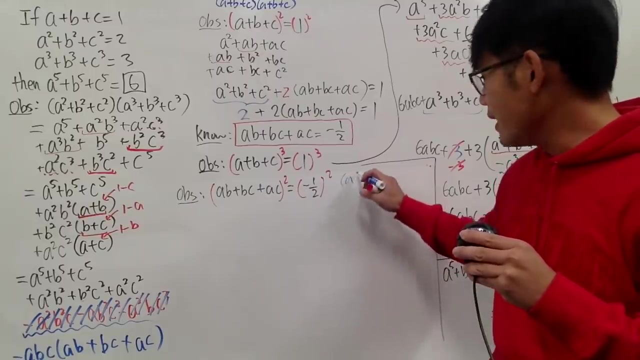 multiply it out by hand and all that stuff. So let's see, Okay, I will just write it down twice for you guys, to make things easier for you and for me. Okay, So I'll just put down a b plus b c plus a c. 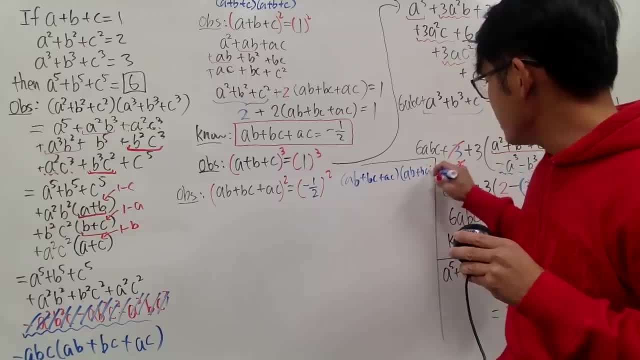 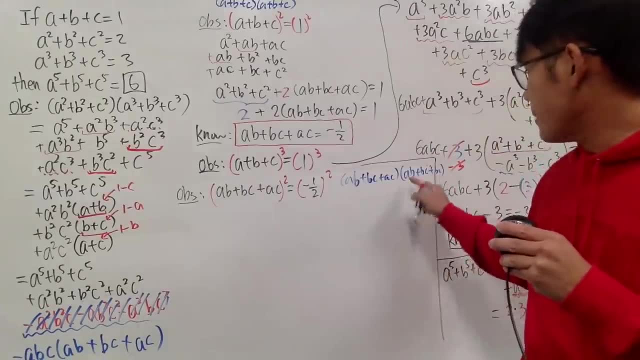 and then another a b plus b c plus b c, Or just do it on your own Right, One over the other. Anyway, here we go. So a b times a b. of course is a squared, b squared, And that's exactly. 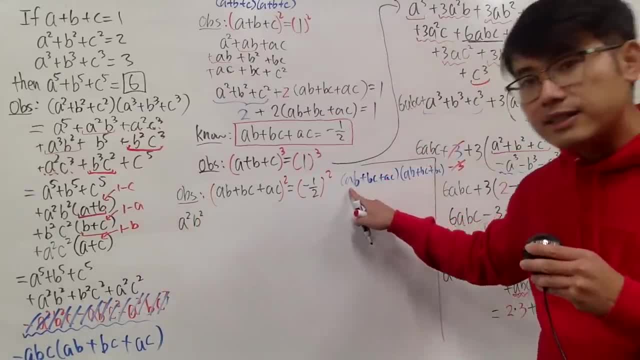 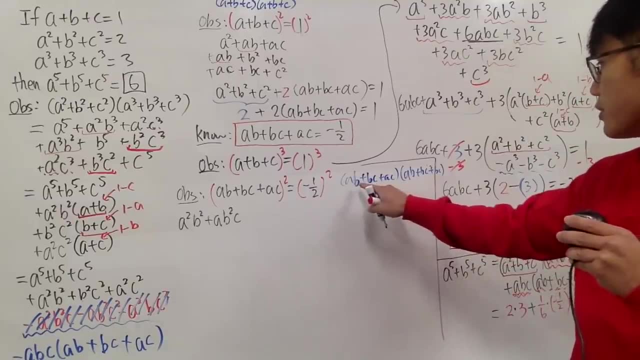 the first term that we have over there, So that's good. And the next one is a b times b c, So it's going to be plus a b squared c, And then the next one is going to be, this times, that which is going to be: 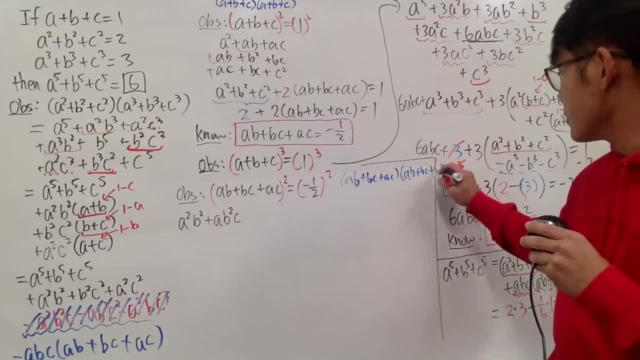 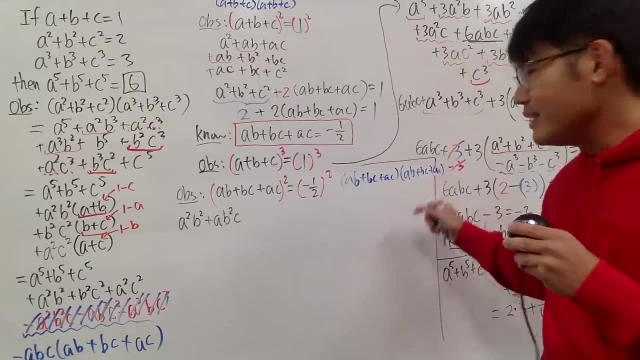 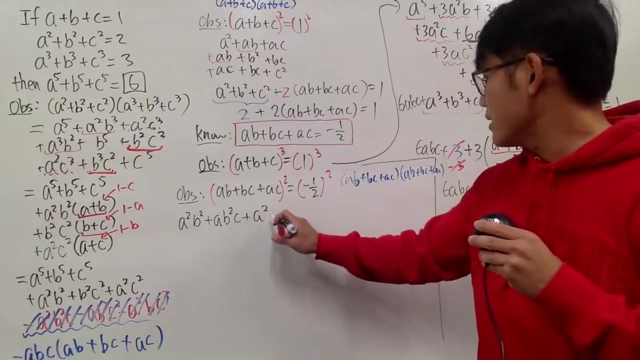 a c. This is supposed to be a c, right here, Right. And then the next one is going to be a b times a c, which is going to be plus a square b c, like that. Okay, So again, you just write this down twice on the. 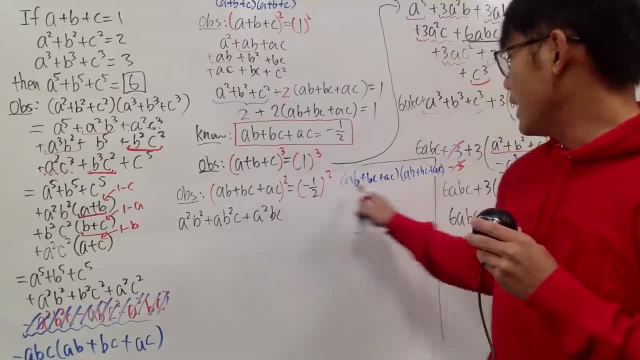 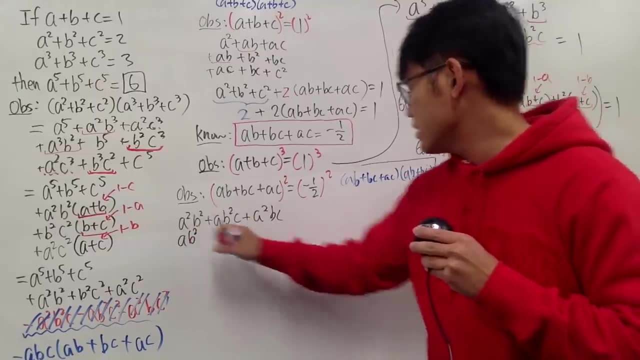 side and then just multiply all that stuff. Okay, Next we have to take b c times this, which is going to be a b squared c And, uh, no b c. So a with a c right, b c times this is b squared, and 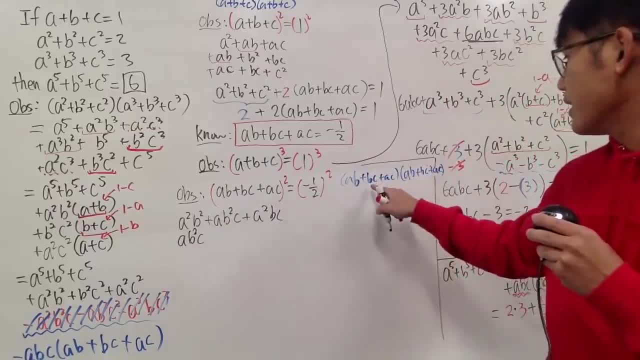 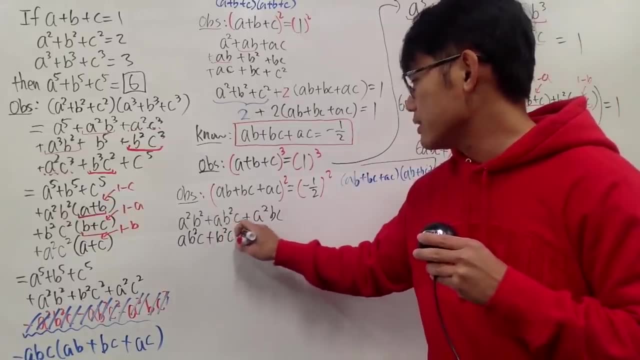 a, b, c, a, b squared, c. And next you take this times that b is being squared. and then you have the b- c, Both of them being squared- b squared, c squared, which is nice. And now you take this times that you get. 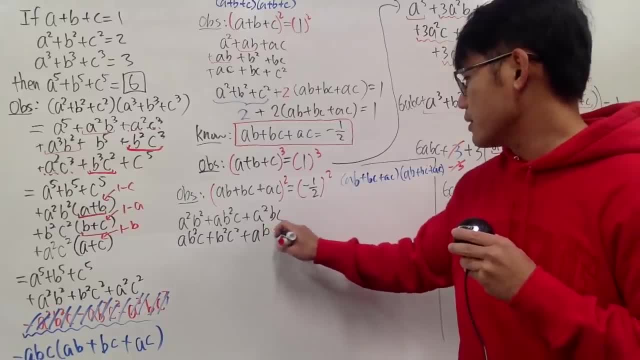 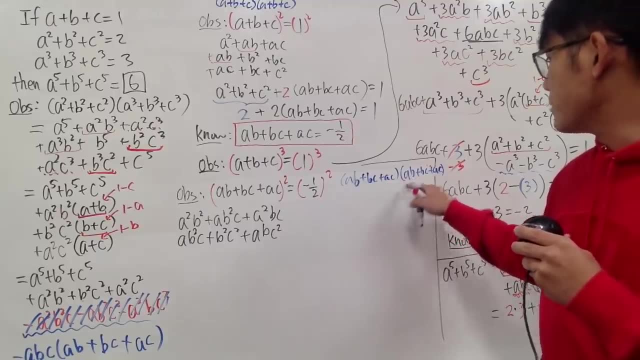 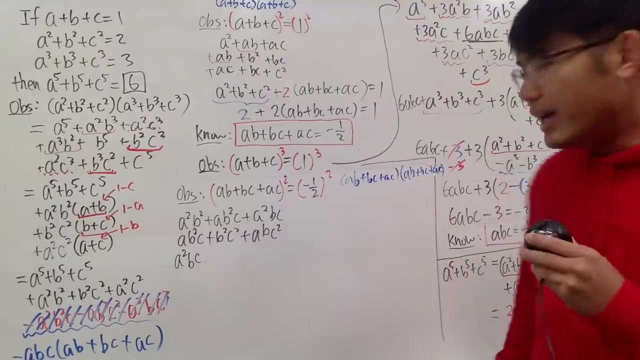 a, b c squared Like that. Right This times that, Yes. And lastly, you take a c times this. you get a squared b c, Like this, And you will have this times that which is a b c squared. 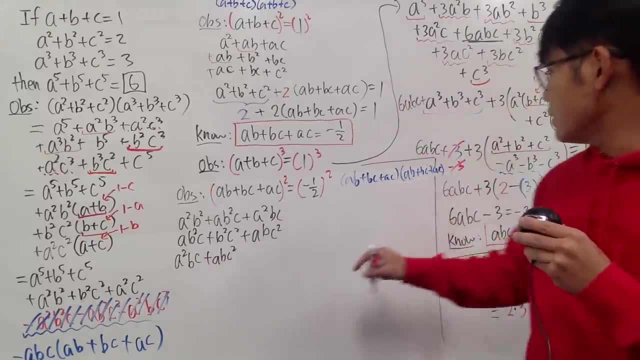 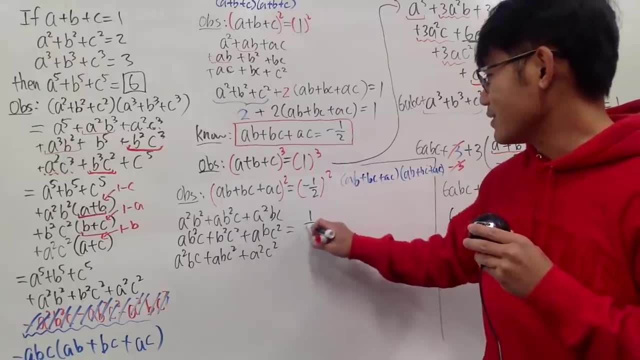 And you will have to do this times, that which is a- c squared, Both of them being squared Like this, a squared, c, squared Like that, And, of course, on the right hand side. this is just nice, It's just positive one over. 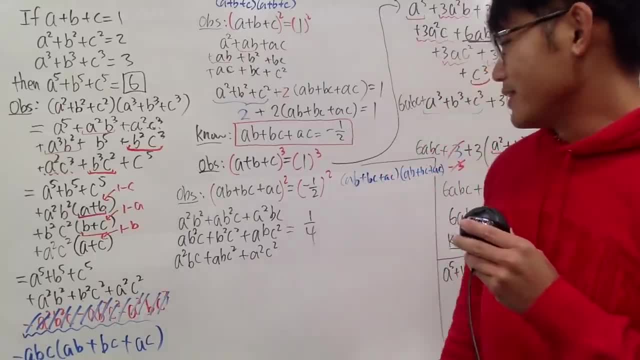 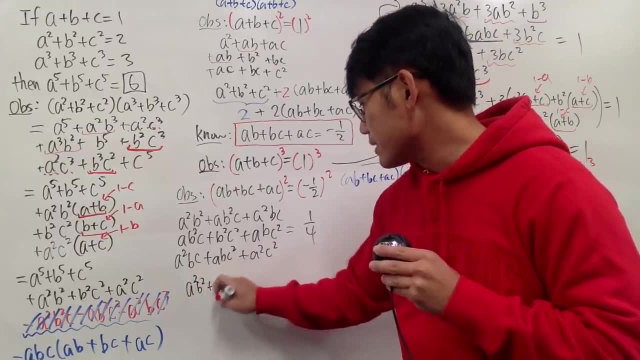 four. Alright, So a lot of algebra today. huh, Now we'll see. This is exactly what we want, So perhaps we just put on a squared b squared plus b squared c squared plus a squared plus a squared c squared Right. 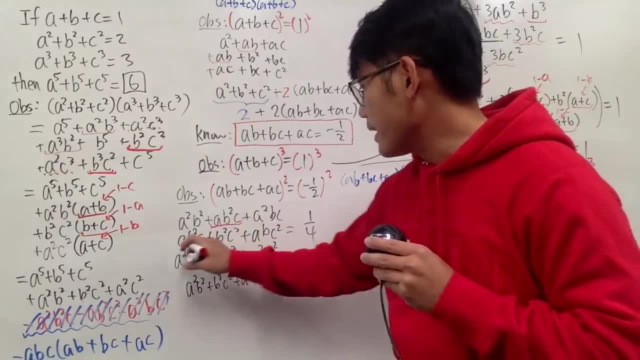 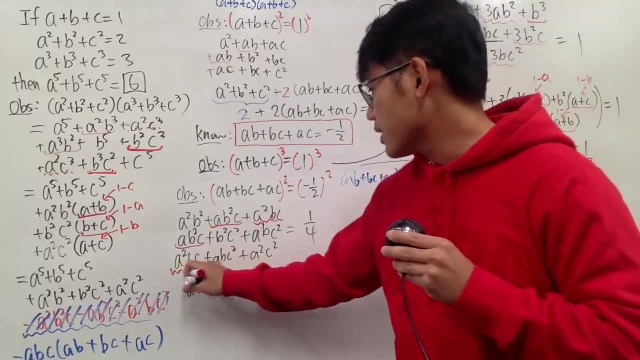 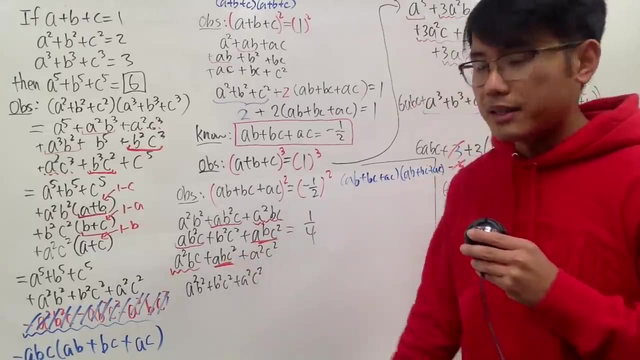 The diagonal. And you see that, in fact, we can combine like terms here and here, So we'll have two of them- And uh, this and that, We can also combine like terms. And uh, this guy and this guy, We can also combine like terms. 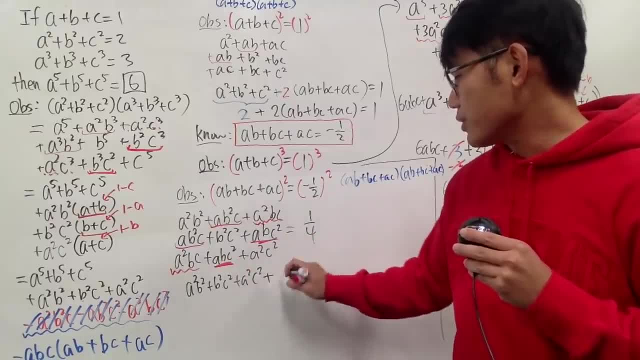 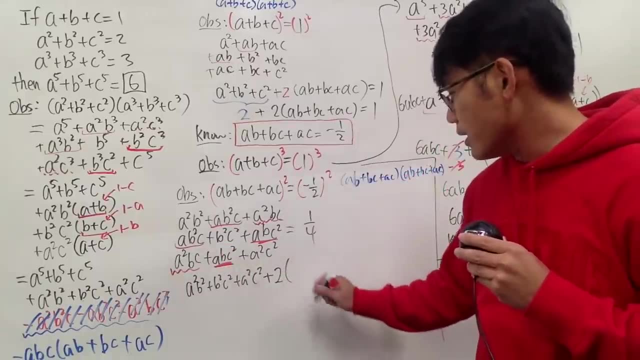 But the deal is that, okay, everybody has two. So I'll factor out the two right here, right Two of them, And you see that everybody have a factor a, b, c. So in fact we can just factor out the a b c first. 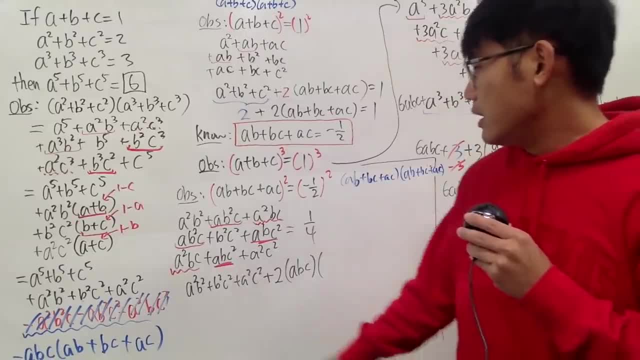 Like this And I'll put on another parentheses, And you'll see that for the first one, when you factor out the a b c, you have the b left, And then for this, and that when you factor out the a b c. 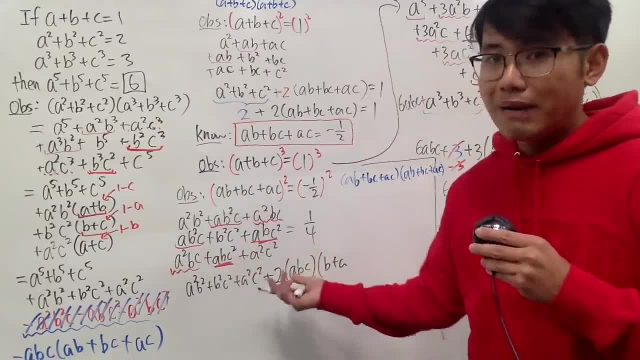 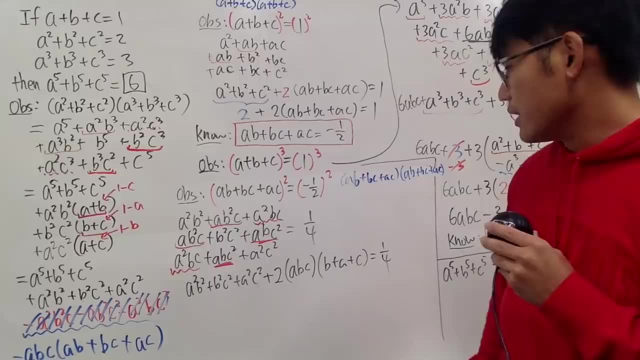 you have the a left And then for this and that you will have the c left, So it's pretty much a, b, c plus right here, And then this is equal to one over four. So that's good. So now this guy is. 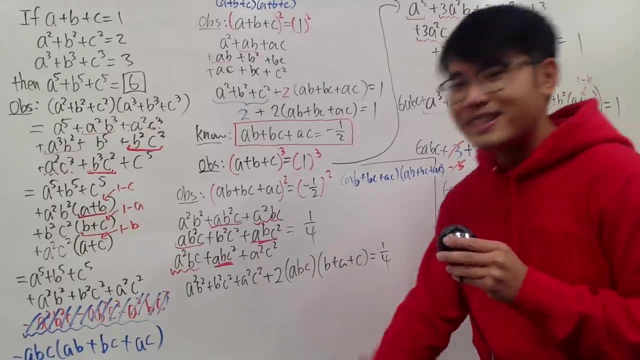 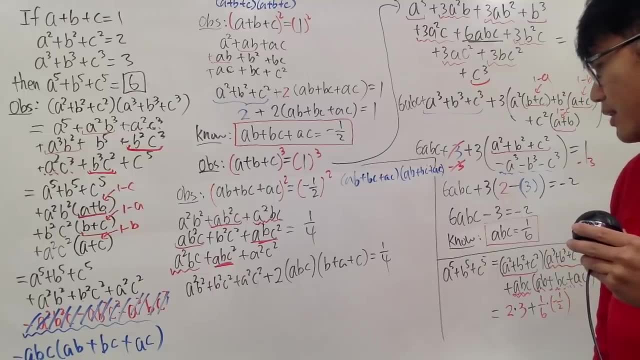 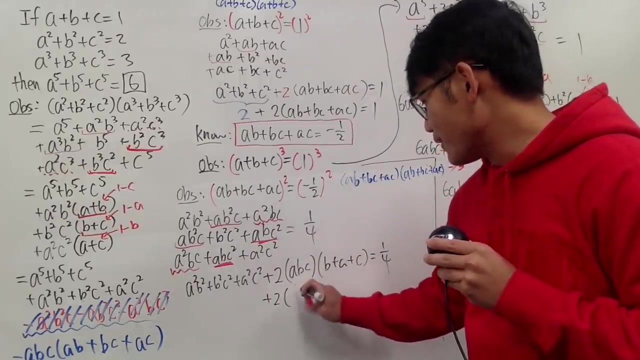 what we're trying to find. This guy, let's see. let's see. Oh yeah, So good, We have the one over six right here. We can use that. So of course we have the plus Two times one over six. Oh, so, thankfully. 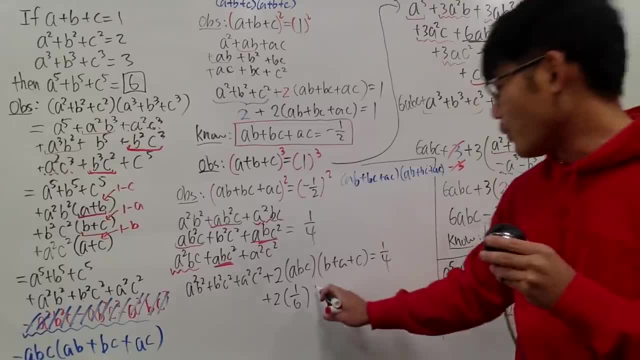 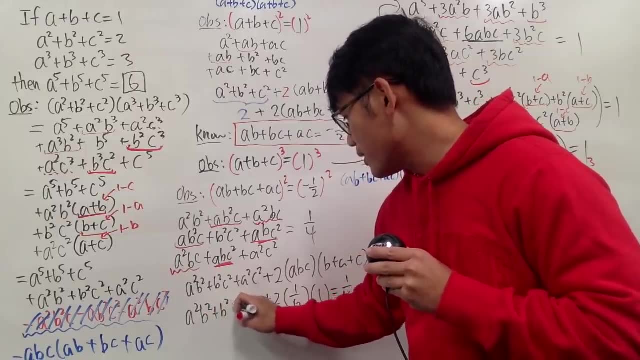 I did this first, So, and then you have the a, b, c, which is equal to one, And this is equal to one over four, And you have the a square b square plus b square c square plus a square c square. This quantity is what we are trying to find out. 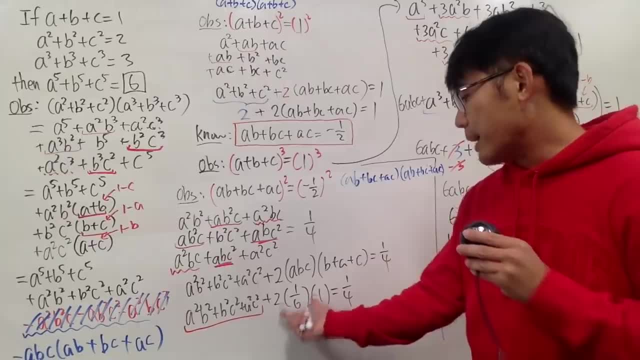 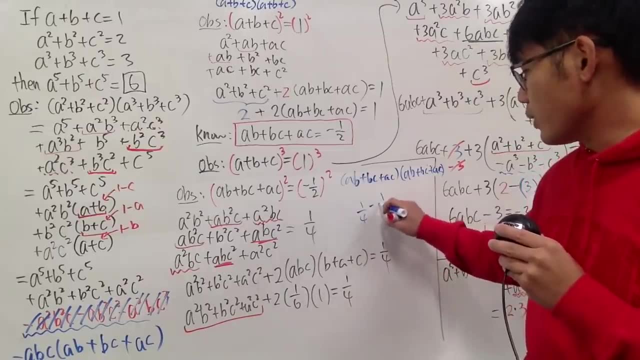 Now, let's do this: in your head, This is going to be past the one over three. Minus that to the other side, you get- let's do this- one over four. minus one over three, You get your common denominator, which is three here and four here. 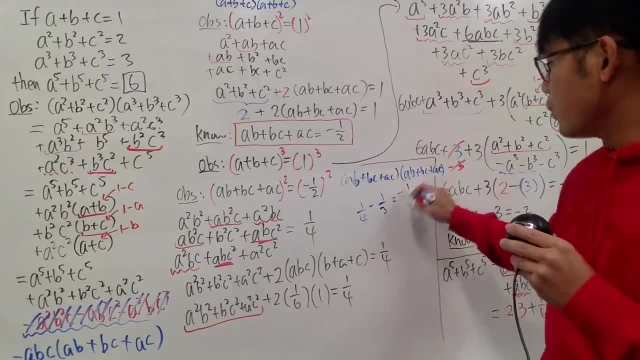 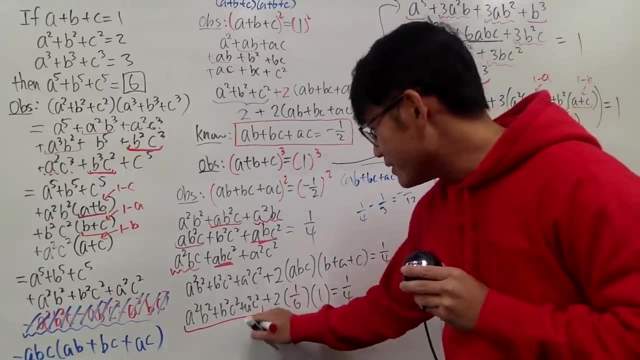 over twelve? right for the denominator. So you get negative one over twelve. Ah, Negative one over twelve? Oh my god, We end up with negative one over twelve as well. So this guy here is just equal to negative one over twelve. Perfect. 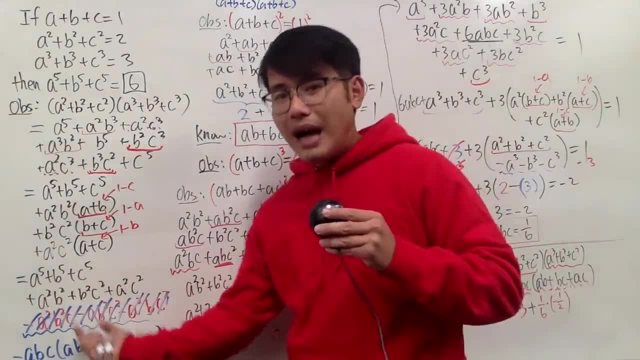 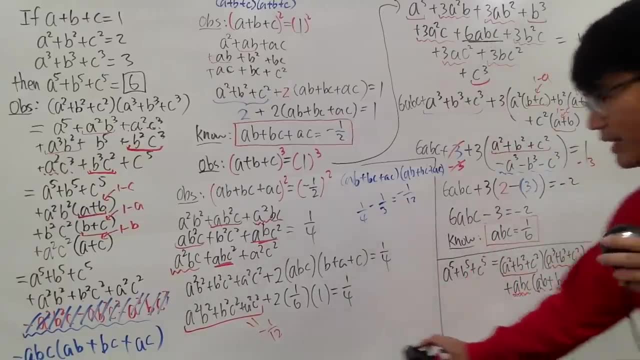 Now here is the deal. You see, earlier I put this down to the other side, so we add it here. But the truth is I will also have to erase that, and I have to do that again Because I will have to bring this guy to the other side, and that's a minus. 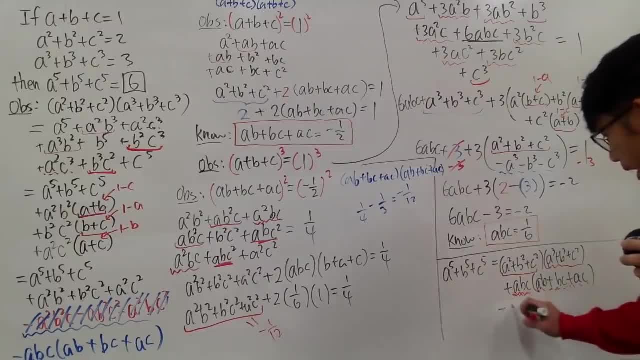 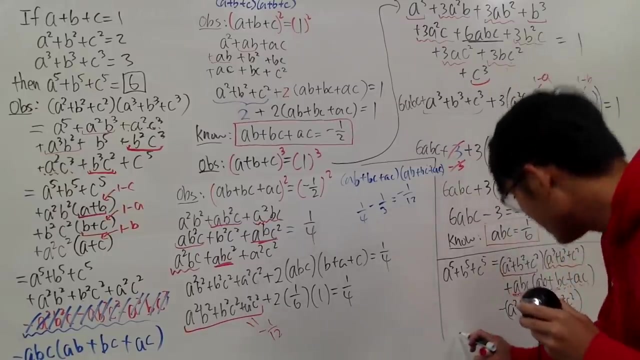 So I will have to minus a square b square, minus Everybody. let's do it like minus parenthesis, plus b square c square, plus a square c square, like that. Okay, Hopefully everybody is good now. So finally, this right here is, Let me actually: 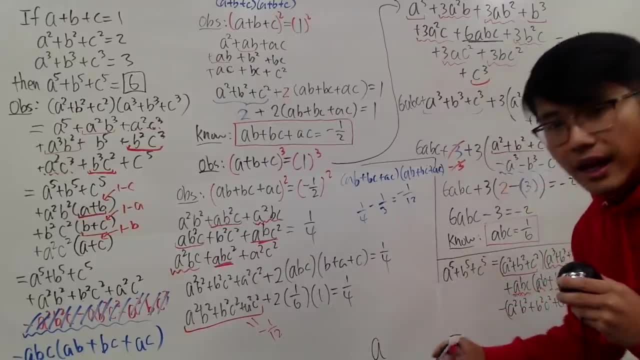 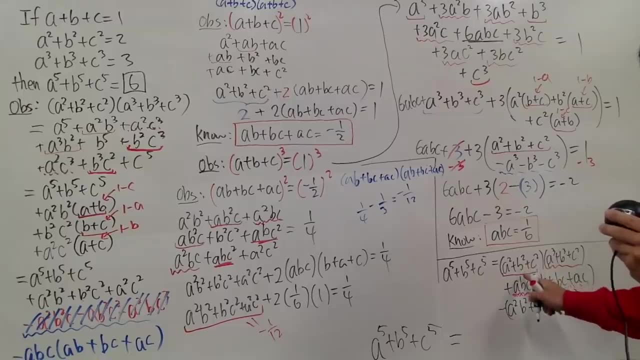 erase that. Let me just write this down legitimately: a to the fifth power plus b to the fifth power plus c to the fifth power is equal to this guy, which is two. This is two Times this guy is three. So that's nice. And then 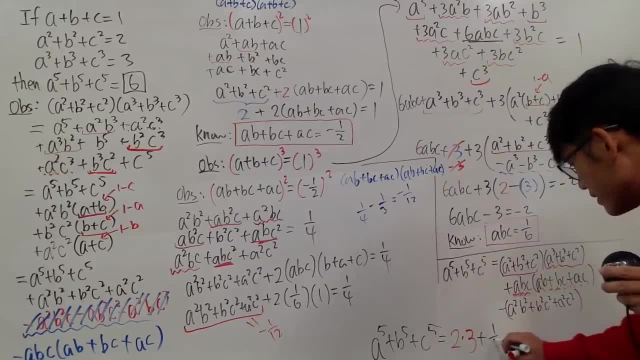 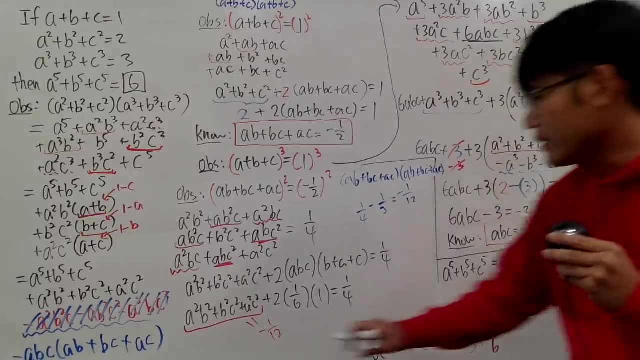 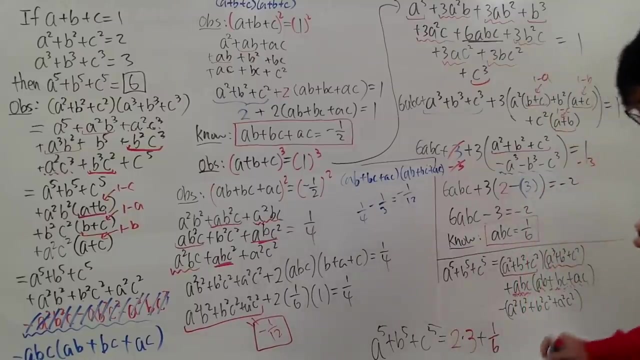 plus this right here is one over six, as we discussed it earlier. One over six, which is the one that's above us Right here somewhere. So this is the one that we got, And then this part is the negative one over two. So we multiply this by: 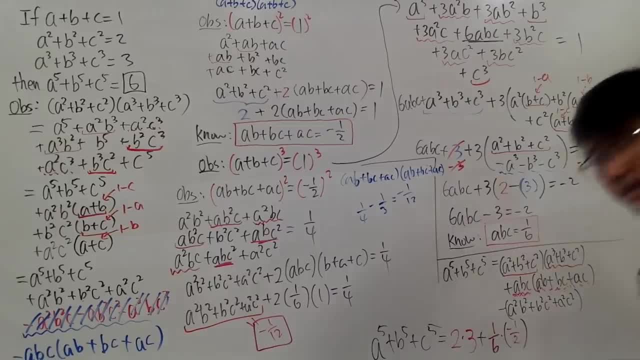 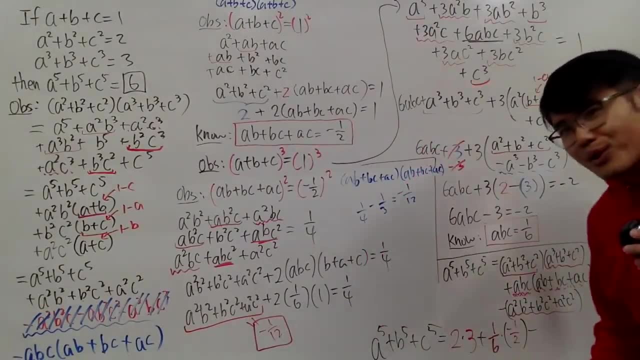 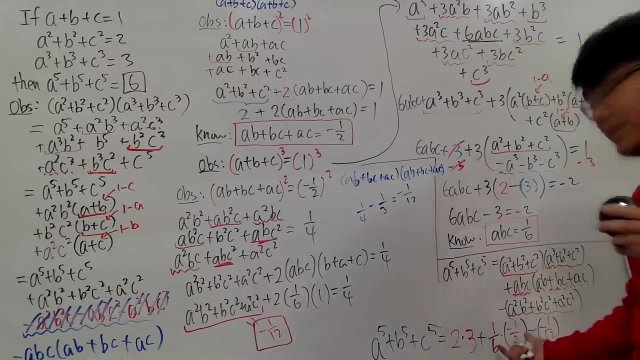 negative one over two And you minus all this guy here is equal to negative one over twelve. So you have your negative one over twelve already here, Alright, So you have the negative one over twelve And, as you can see, of course this is positive, That's negative. 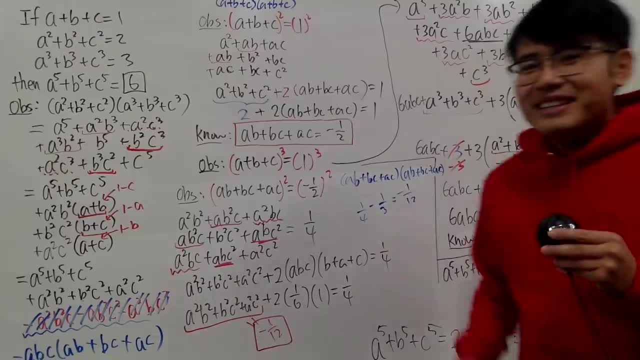 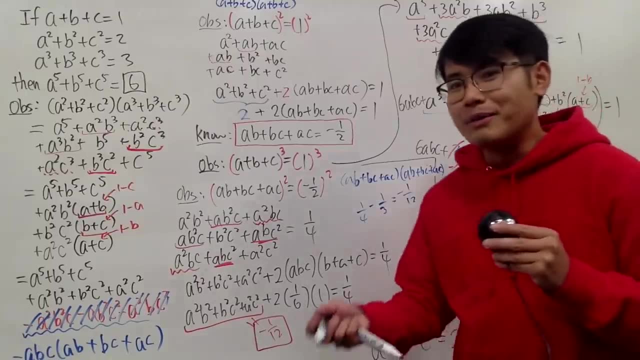 one over twelve. So this and that will cancel. So, ladies and gentlemen, a to the fifth power plus b to the fifth power, plus c to the fifth power is equal to two times three. I told you it's two times three. That's how we get the six. 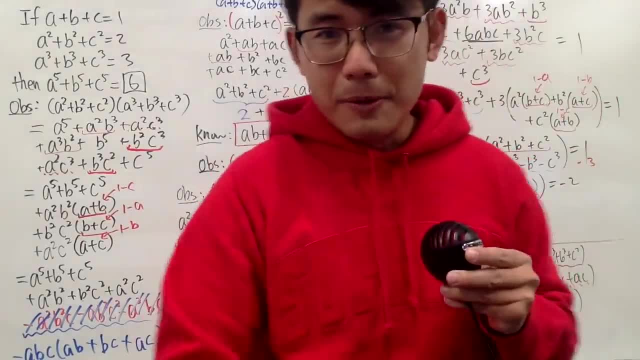 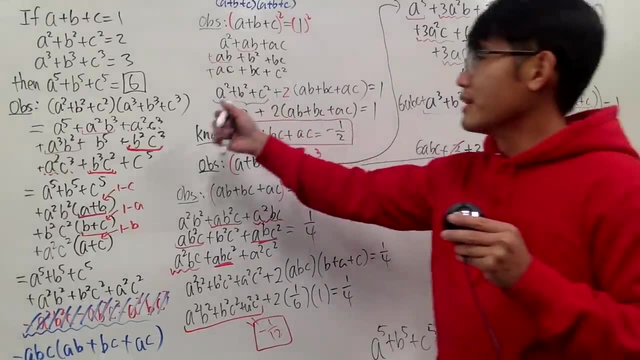 So I could have end this video about like I don't know forty minutes ago or something like that, right, So let's see, I'll just box it here somewhere. Oh, it's boxed right there. So here is the answer. This is the. 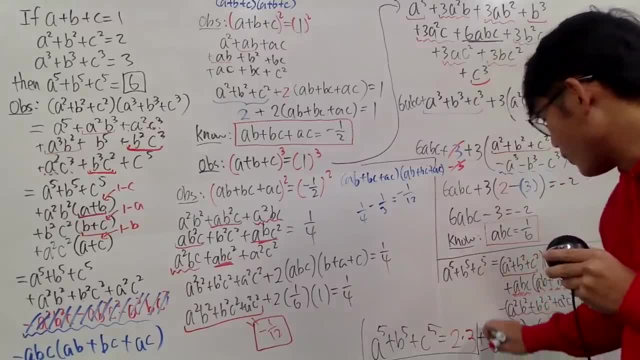 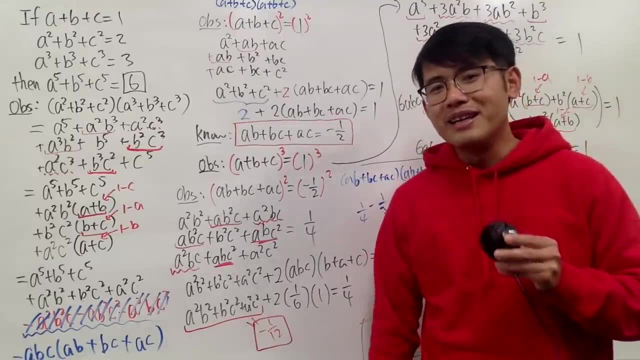 legitimate answer. So this right here is it Right Boxed, the final one for you guys. Okay, That's it. So another algebra right here, And hopefully you guys all like this video to a certain degree because I did show you guys the interesting part. 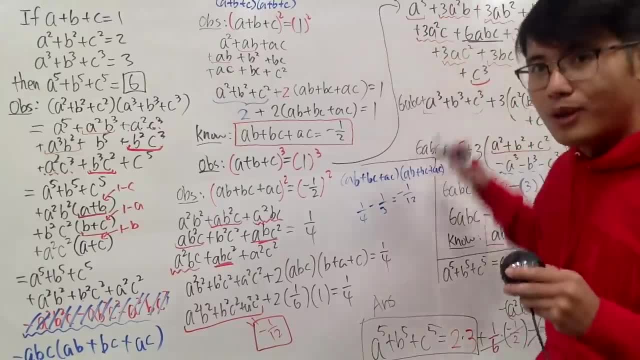 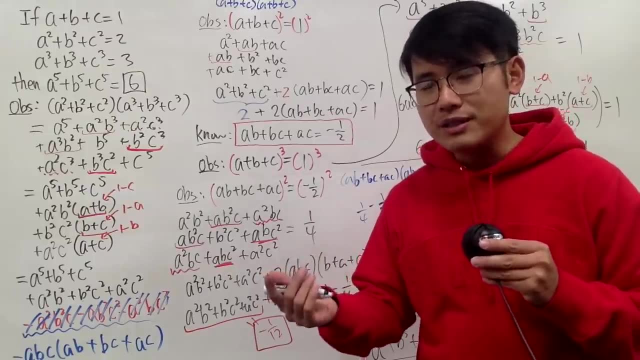 which is the more like a discrete math approach, The trinomial coefficient, And also we can talk about the. you know, if you have how to find the number of solutions, the water period will satisfy like a. like x plus y plus c is equal to n. 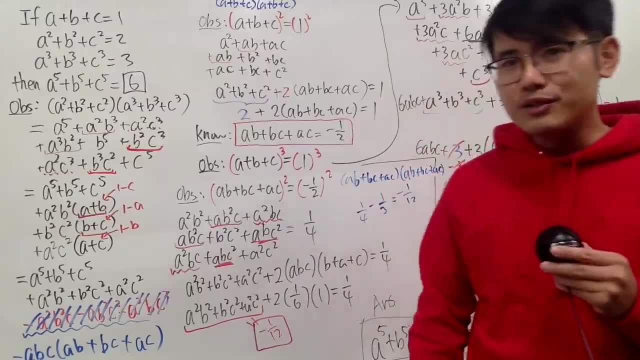 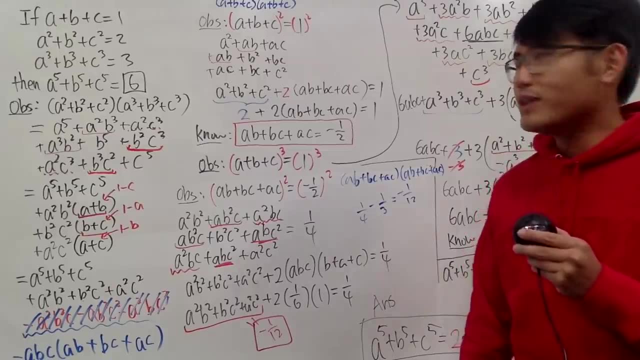 in non-negative numbers and all that stuff. So I will have those videos for you guys later on, But as of now this is a pretty classic math competition question, but we are doing the fifth power instead. The famous one is this one: a, b, c.